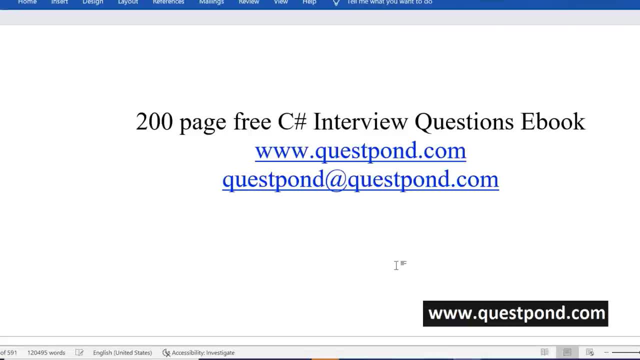 I want to give you a small gift out here. Here is a small gift which is a 200 page C Sharp interview question eBook. If you share this video anywhere on your LinkedIn or on your Facebook or on your Twitter, you will get this free C Sharp interview question eBook- a 200 page eBook. 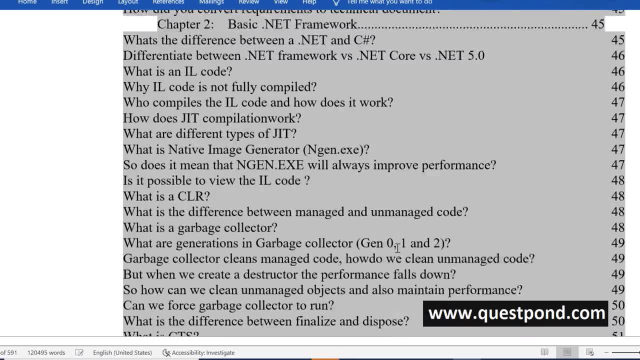 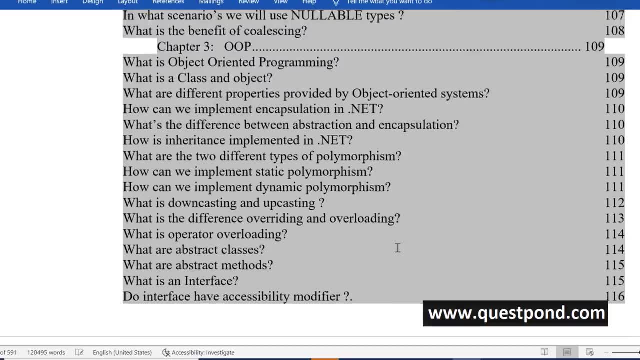 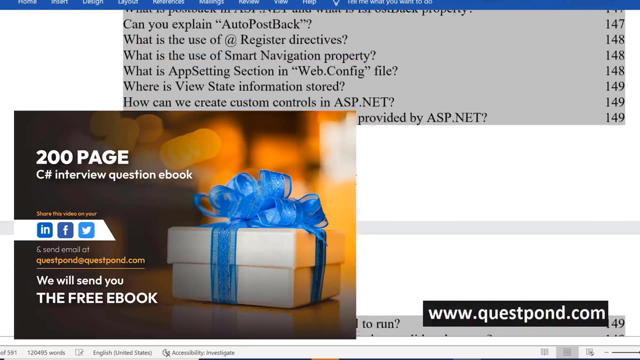 you can see here i'm scrolling this book. there are lots and lots of questions out here which every C sharp and dotnet developer would like to revise before going to the interview. right? so i would suggest guys go ahead share this video anywhere on your linkedin um on your. 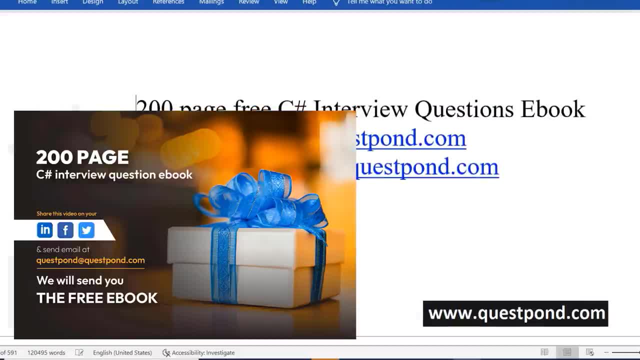 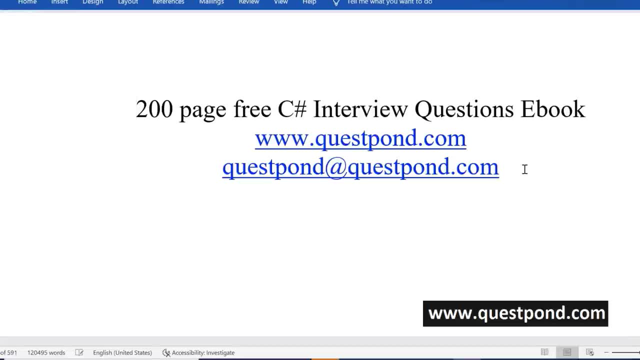 facebook, on your twitter, and get this free ebook. and please visit my website, questpondcom. we have lot of videos out there which are specifically meant how to crack interviews, how to get your next jobs, how to prepare for technical things right. so a lot of videos out. 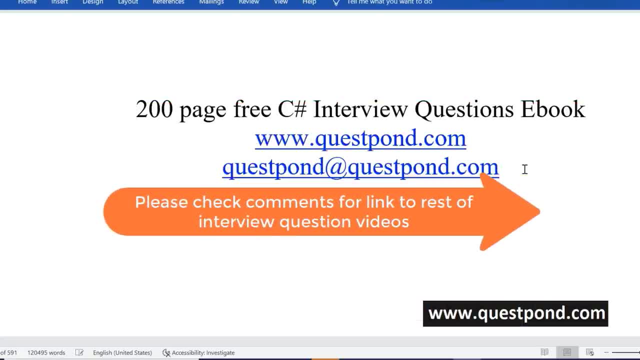 there, you know, c sharp interview questions, asp dot interview questions, sql server interview questions, azure interview questions, angular interview questions. so interview questions with demonstrations, um, you know, with proper explanation, which will help you to get the next job right. so with that, you know, let us go ahead and get started over here with 25 plus important object. 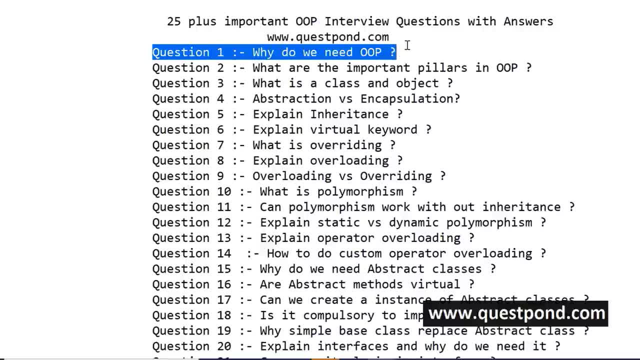 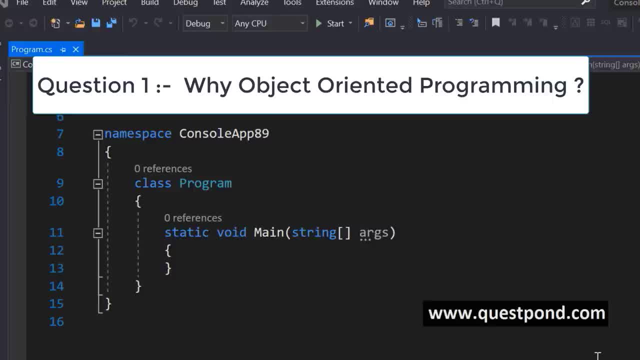 content programming interview question. and let us start with the first question: why do we need object oriented programming? what is the need of object-oriented programming? what is the benefit of using object-oriented programming? now, when this question comes up right, many developers, many developers, answer: like: object-oriented programming will make your code. 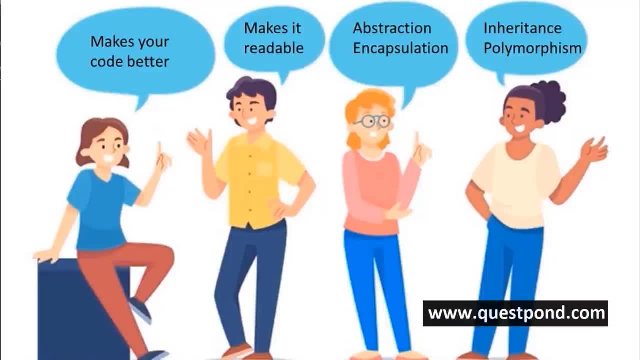 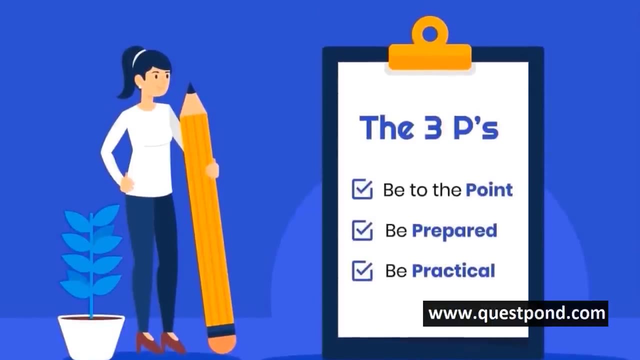 better. it makes your code readable. some developers talk about features of object programming like abstraction, encapsulation, polymorphism and so on. please, please, do not hit around the bush. answer to the point: the first p in a technical interview. answer to the point: the person who is taking your interview is a senior person. he does not get extra paid for it, at least to my best. 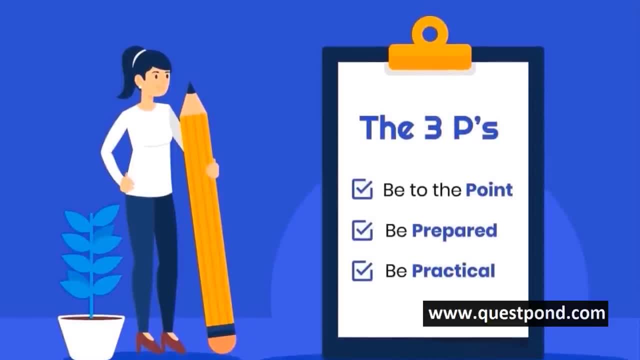 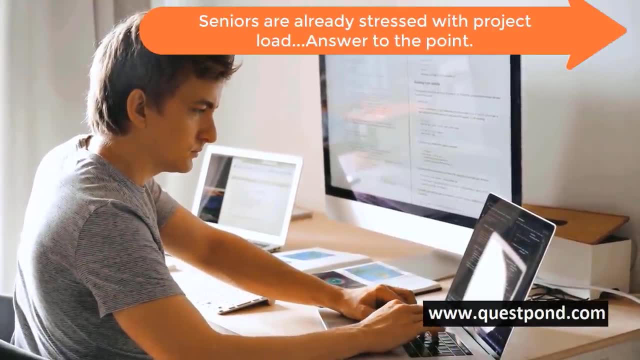 knowledge. when you take an interview as a senior, you don't get paid. he is already stressed with project deadlines and the and on the top, you know in the interview, if he's seeing hitting around the bush, it just irritates him, right? so let us try to answer this question to the point. why do we need 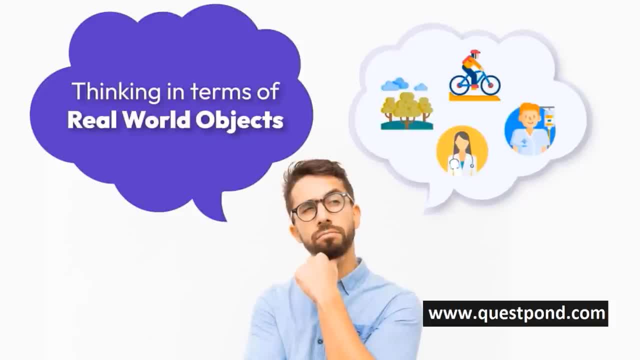 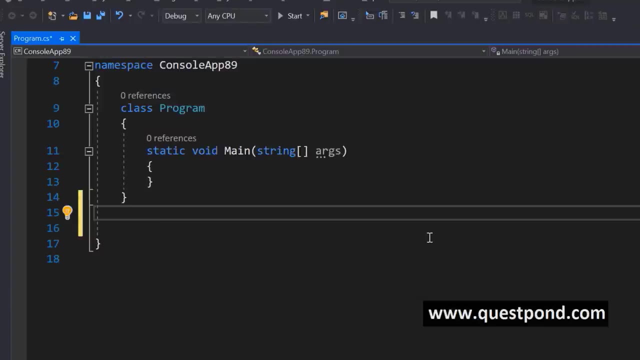 object-oriented programming. object-oriented programming helps us to think in terms of real-world objects. let me trade this sentence: object programming helps us to think in terms of real-world objects. let us try to understand this statement: thinking in terms of real-world objects. so let us say you are creating a software for an hospital. 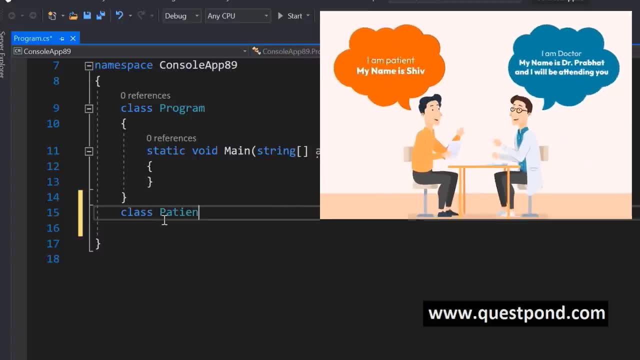 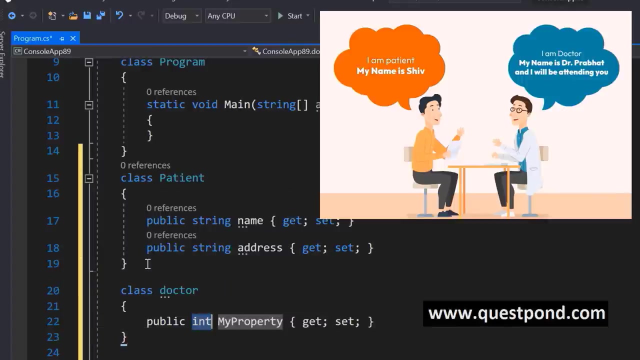 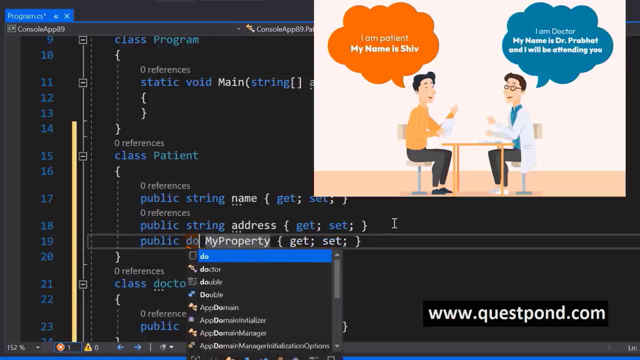 so what does a hospital have? a hospital has patients, fine. so what you will do now? you will go Go to the code and create a class: patient. The patient is allocated to a doctor. a doctor treats a patient. This is the doctor object aggregated inside it. 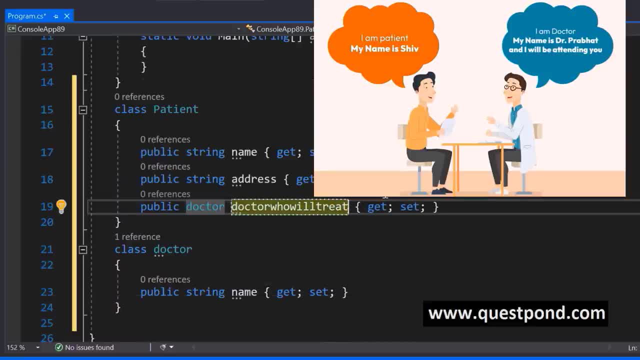 The code is mimicking the real world. object: patient has a name address. there is a doctor. there is a doctor who is allocated to a patient. By having such approach, we can manage the code better. the code gets organized properly. Object oriented programming. 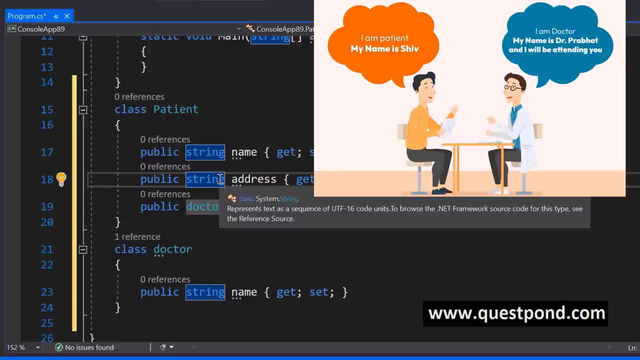 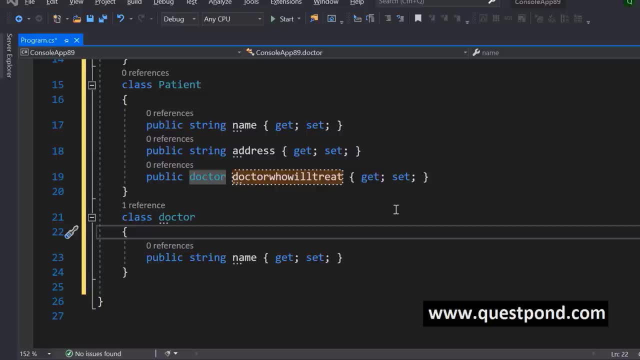 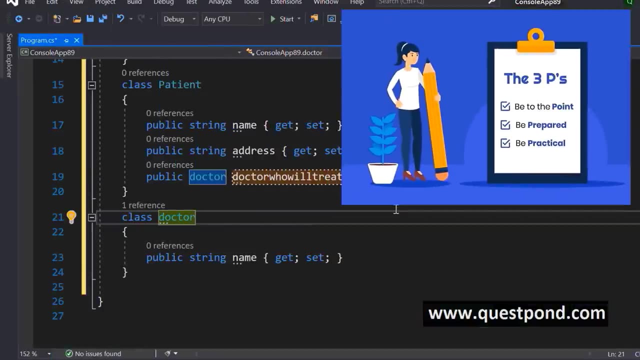 helps us to think in terms of real world objects. As we complete the first question's answer, we will stress one more important P about technical interviews, ie be practical. Whenever we give an answer in an interview, always try to substantiate it with some practical examples. 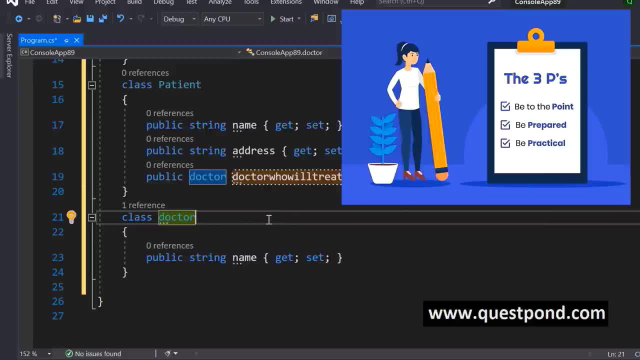 Object oriented programming helps us to think in terms of real world objects. We gave an example of a hospital. we gave an example of a patient, of a doctor attending the patient. we talked about aggregation. Try to support your theoretical answers with some practical examples as well. 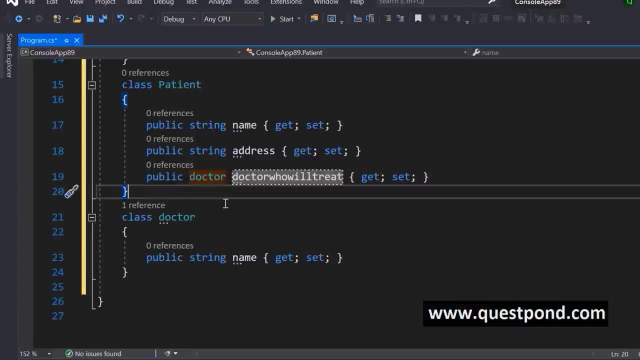 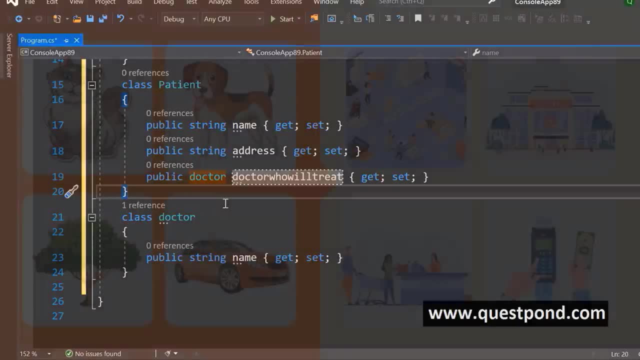 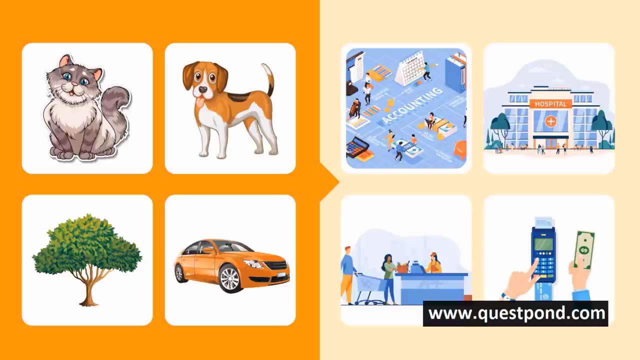 This sends a message to the interviewer that, yes, you have worked on enterprise applications and you are the person for this job. One serious request: when it comes to object oriented programming, don't give examples about cars and dogs and cats and trees and fish and TV and so on, because 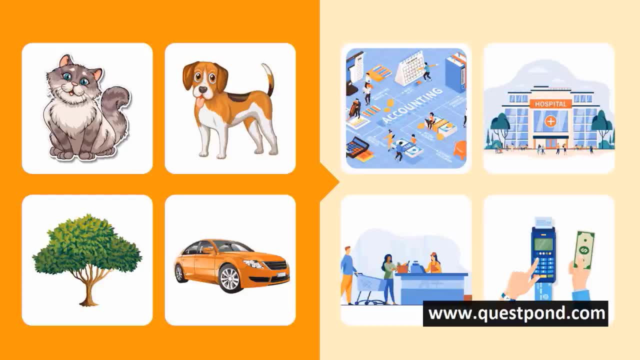 it can send a wrong message to the interviewer. It can make the interview very weird. Always try to give examples like inventory, payroll, billing, accounting, hospital management system or something your domain. whatever domain you have worked with, try to give examples around that domain. 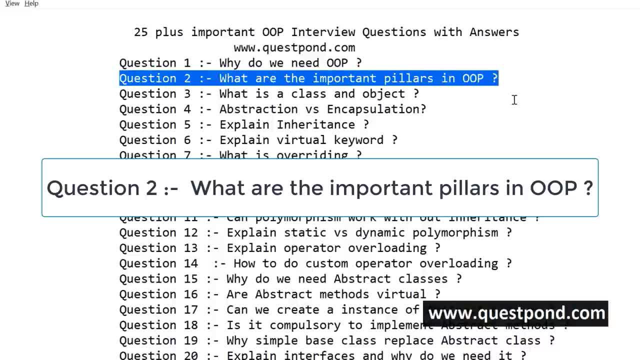 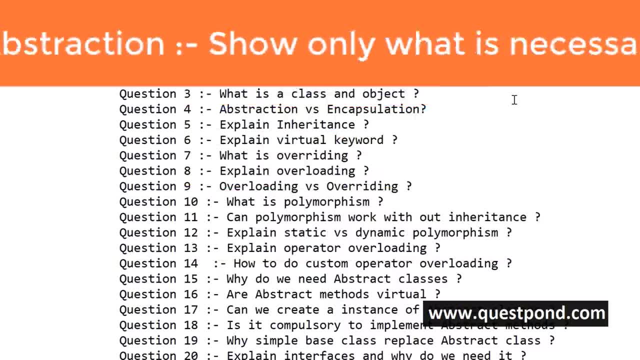 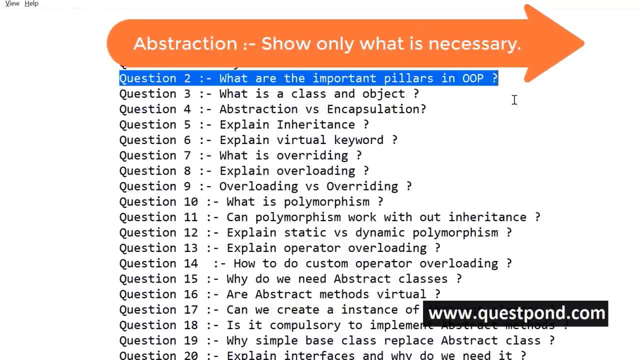 Will start with question no 2. What are the important pillars in object oriented programming? There are four important pillars in object oriented programming. The first one is abstraction. Abstraction means show only what is necessary. Second one is polymorphism: Object can act differently under different conditions. 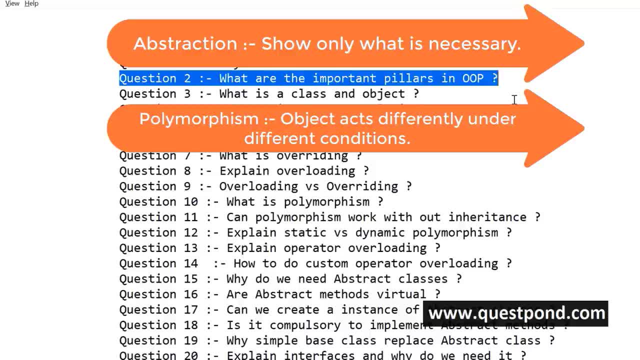 A user object can become an employee, user object can become an admin or user object can become a worker. Object can take different shapes in different conditions or it can act differently under different conditions. Third one is inheritance. You can have a parent-child relationship where you have some things common in the parent. 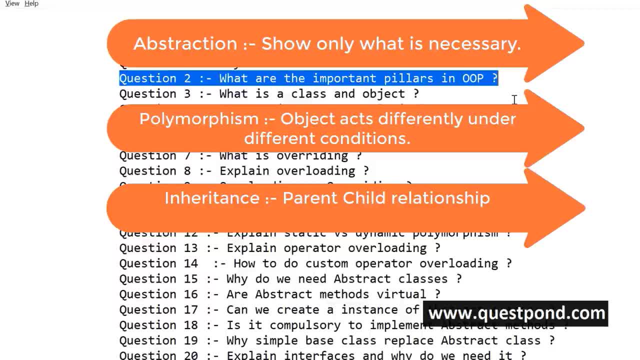 and the child can inherit and add something more to it. Last one: Encapsulation means hide complexity. so hide anything which is complex, which should not be shown outside the object. you should try to hide it. Abstraction, Polymorphism, Inheritance and Encapsulation. 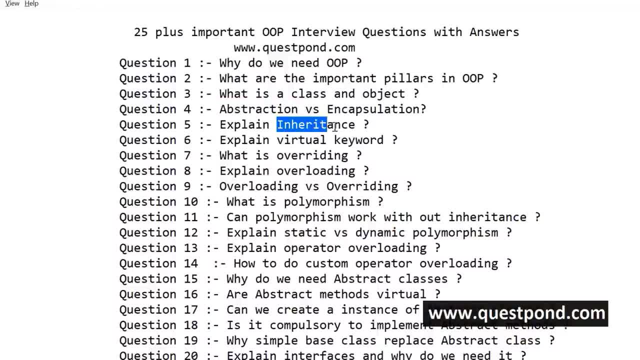 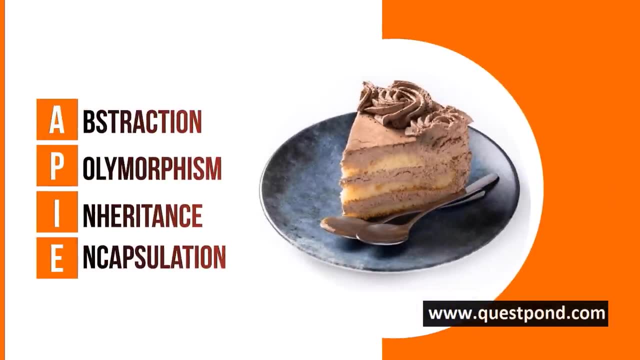 In the coming up lectures we will talk very detail about Abstraction, Inheritance and so on, but this question is very focused. the question is: what are the important pillars? so I just answer these four points. Very important point in case you don't remember these four things, remember the word API. 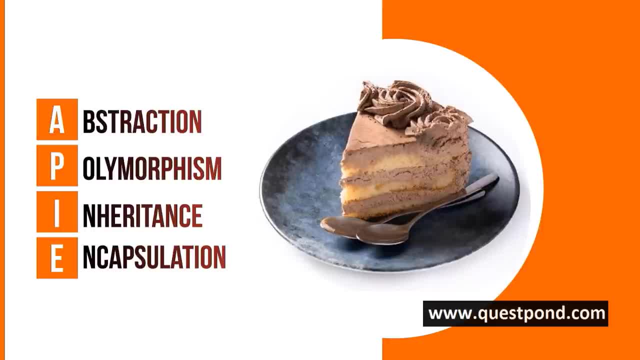 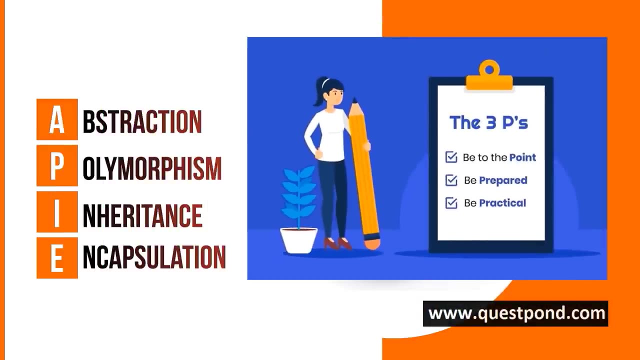 A for Abstraction, P for Polymorphism, I for Inheritance, E for Encapsulation. Do not shy. Do not be shy. The third P: always be prepared. everything is fair in job and war. it's okay to use acronyms. 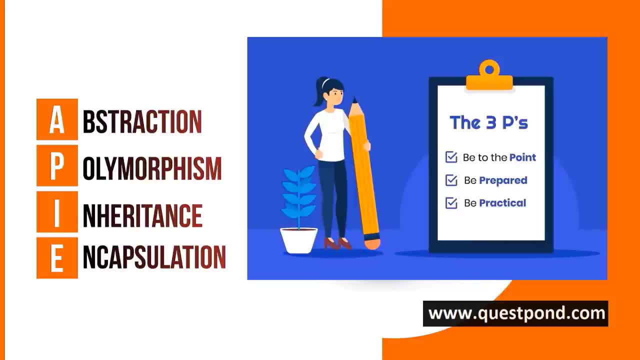 You are working in a company. you are doing some practical works out there. you are sending emails the whole day, you are not revising the whole day, you are not learning. you are actually doing a job. so doing a job and cracking an interview are two different things. 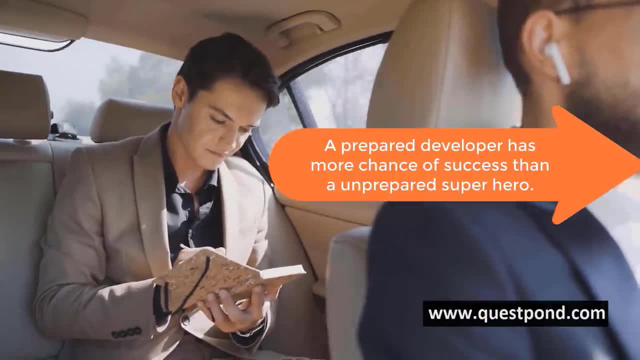 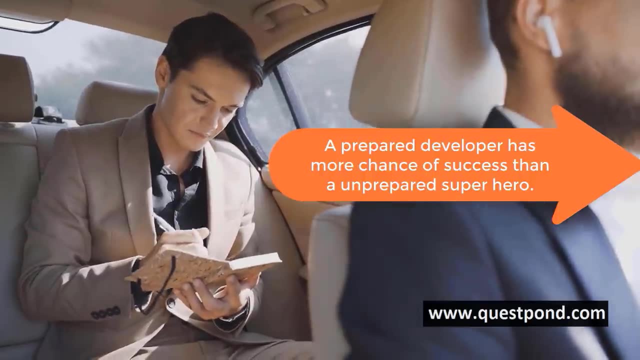 So be prepared. a prepared developer has more chance of clearing the interview than an unprepared superhero. You can be a super hero in a company. you would have delivered big projects. but if you don't answer simple questions like what are the important characteristics of object oriented? 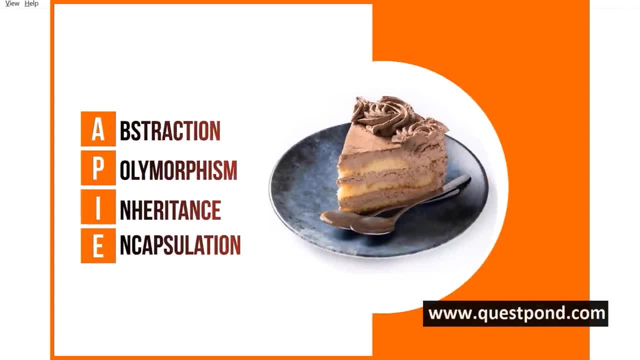 programming. it is very difficult. you can clear the interview For this question. you can remember this acronym: API, Abstraction, Inheritance, Polymorphism and Encapsulation. Before we move to the rest of the questions, We will talk about the key components. 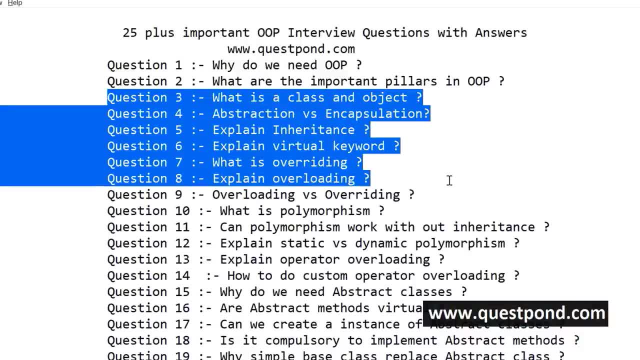 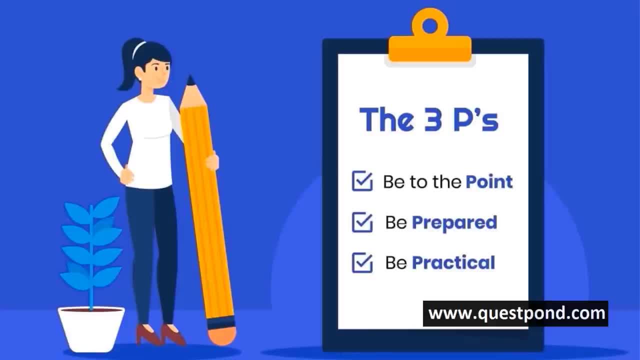 Let us reiterate those three P's. If you remember these three P's while you are giving the answers, believe me half of your problem is solved. First P: be prepared. Second P: be to the point. don't waste the interviewers time. and the last P: be practical. talk about. 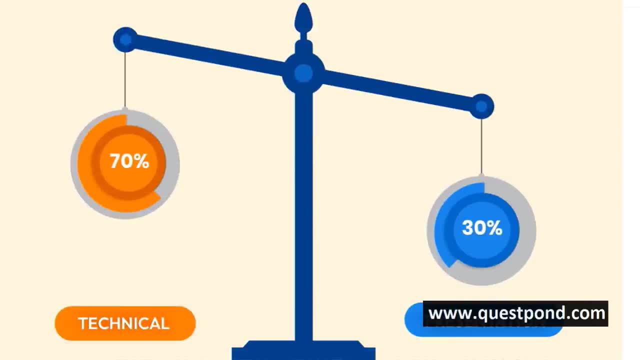 some practical examples. Cracking a technical interview is 70% technical. 70%, yes, you should have a knowledge of the topic, But 30% you will like it. So be prepared. Whether you like it or not. like it is about presentation, it is about your technical vocabulary. 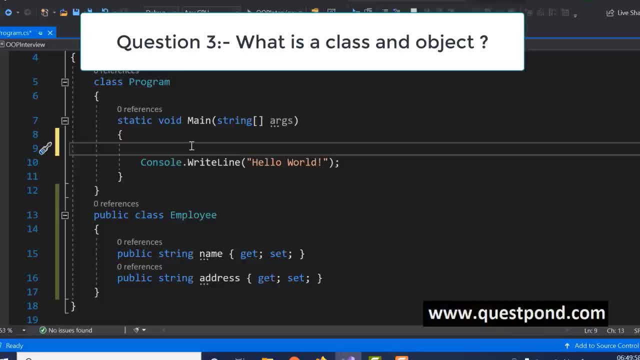 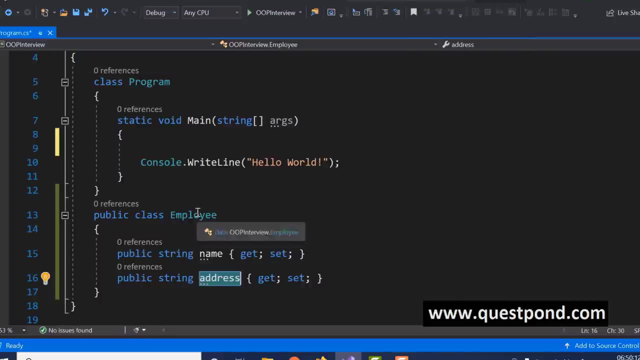 Let us move to the next question: what exactly is a class and what exactly is an object? A class is a blueprint, a class is a type. so you can see: this is a class employee, it has name, it has address. probably it can also have some functions, methods, right. so this class? 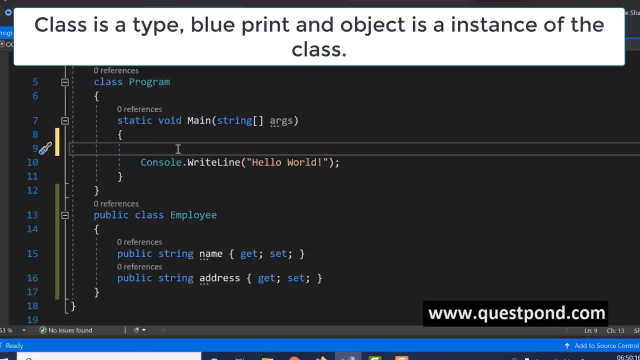 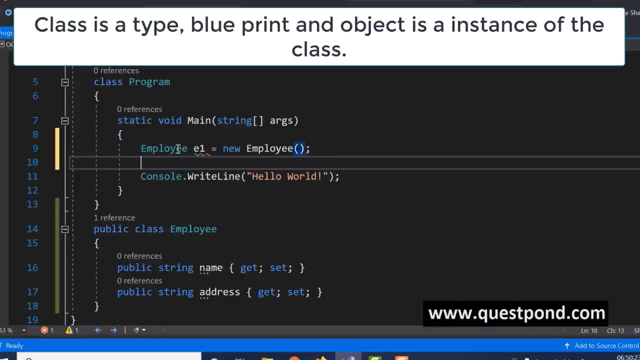 is a blueprint. Now if I want to go and use this class then I need to go and create an instance. So for I will say, employee E1 is equal to new employee. So now here E1 is an object, it is an instance, right? or I can create one more instance: E2. 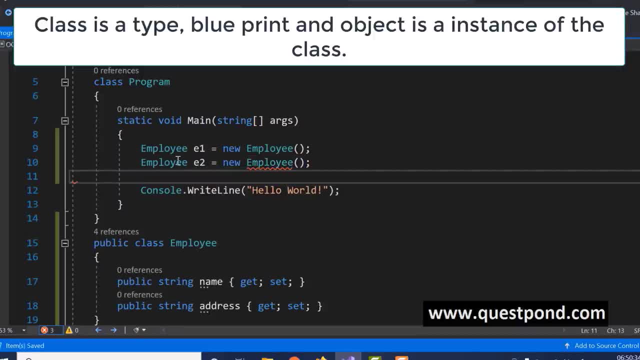 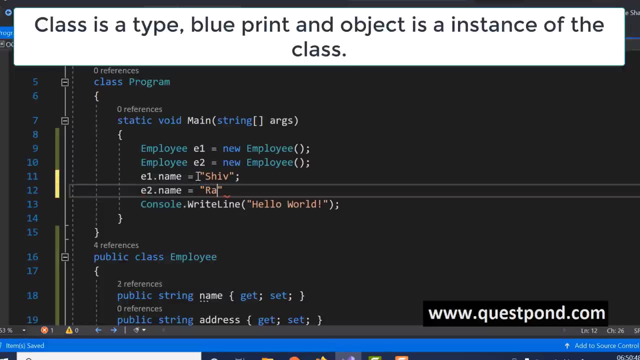 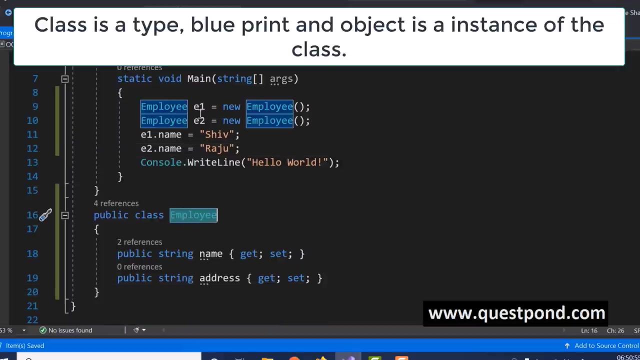 is equal to new employee. So this is a second instance. so you can say that, okay, E1 name is Shiv right employee and the E2 name is something right. So We can say: a class is a type a blueprint, why, if you want to use the class, you need. 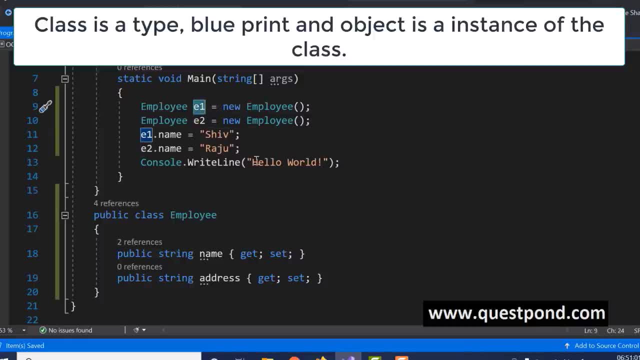 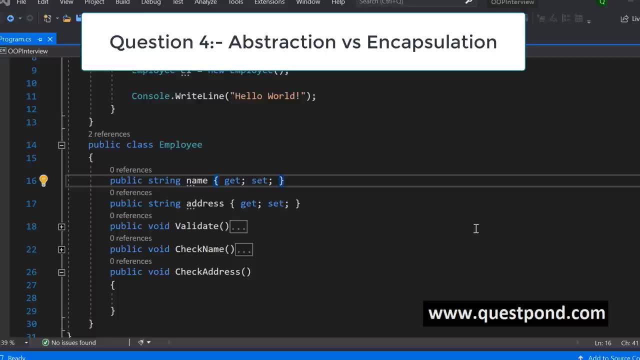 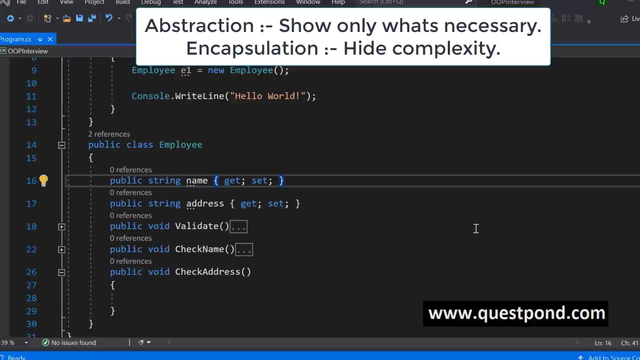 to go and create an instance of the class which is an object. differentiate between abstraction and encapsulation. So now the answer to this is: abstraction means show only what is necessary and encapsulation means hide complexity. I repeat the answer: abstraction means show only what is necessary and encapsulation means 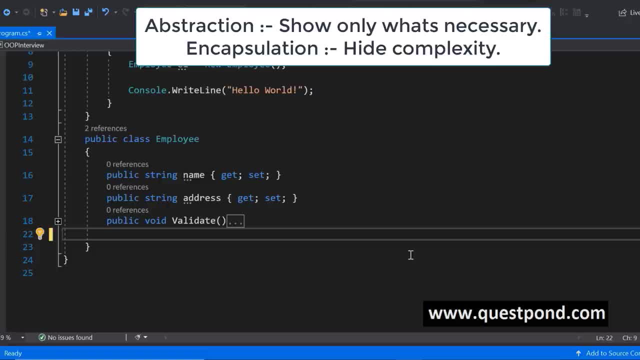 hide complexity. If you look at the answer, it is so synonymically same. it is like saying that we are happy when we drink beer and drinking beer makes us happy, right? So definitely again. the interviewer will counter question you saying that: what's the difference between abstraction and encapsulation? 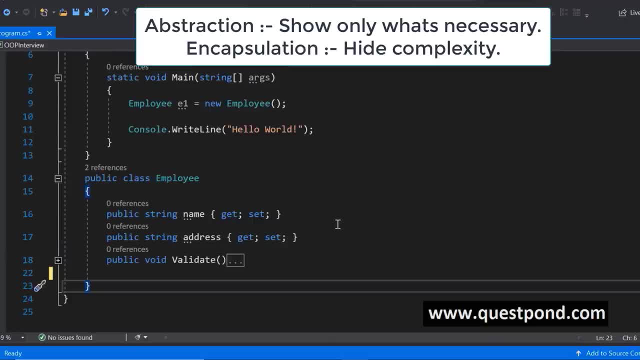 So here it is. Abstraction says that show only what is necessary. so for example, now let us say this is an employee class, so in the employee class the name has to be shown outside. so we made it public. address has to be shown outside, we have made it public. and then this is the validate function, which 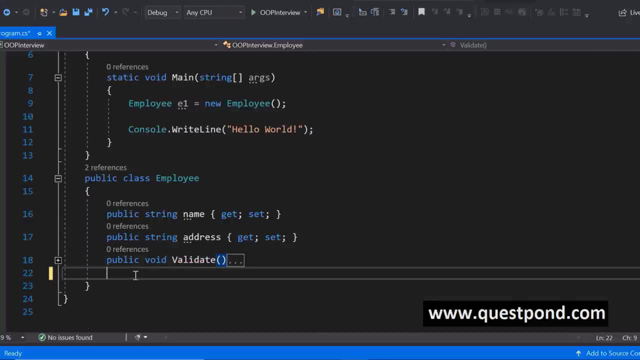 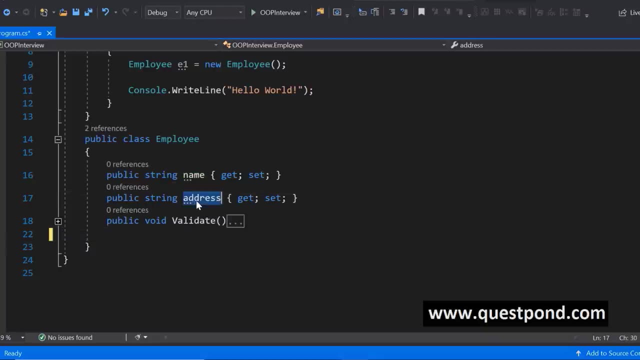 has to be shown outside and we have made it public. But now what happens is you know, for example, you know when you say validate, right. so you would like to go and validate the name, you would like to go and validate the address, right. so what happens is you create the two more functions. 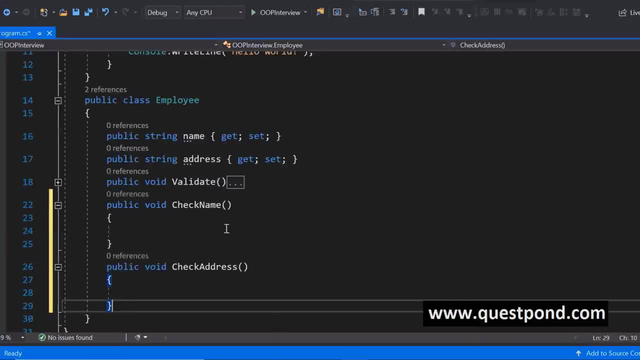 So I will say rather, developer will create two more functions, like saying check name, which will actually check the name, check address, which will actually check the address right. So inside the validate function you will have now check name and, must be, you will have check address right. 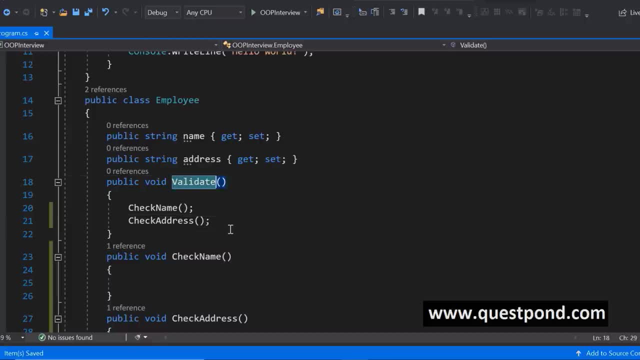 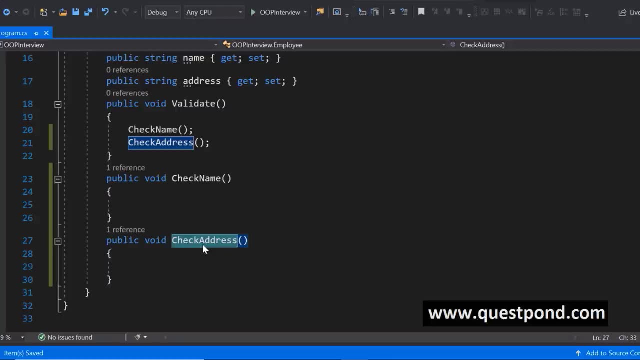 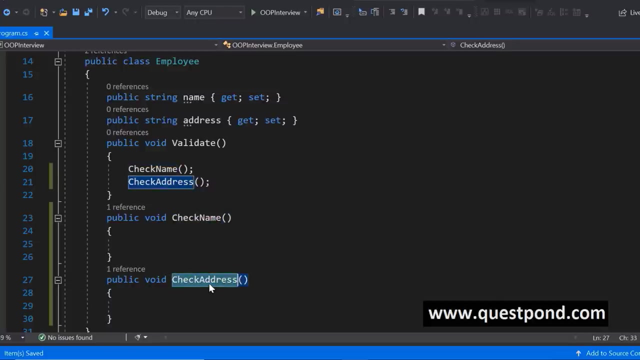 But now you want to only show validate outside and not check name and check address. check name and check address Right. Internal things: developer has created it right, actually, So when he actually started coding, developer has created both these functions so that the validate function can be completed right. 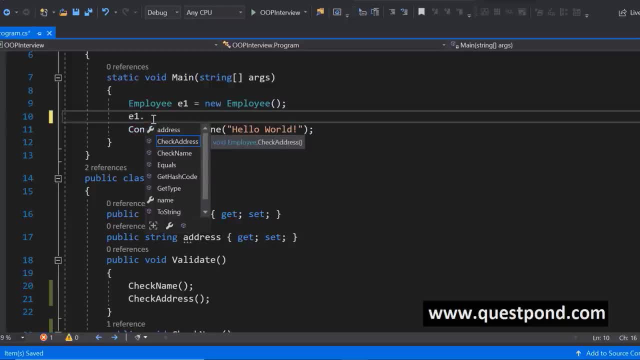 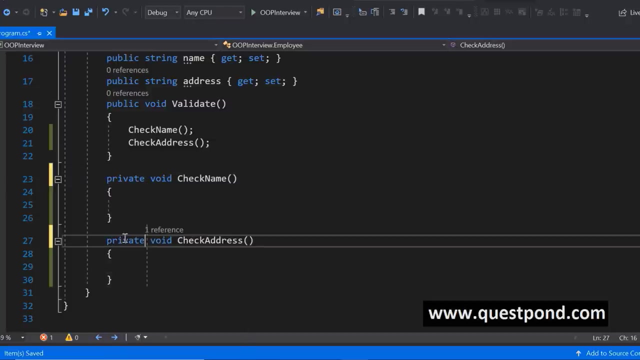 But now what happens? because of making everything public, you said in abstraction that or we decided that for the employee class only validate should be seen outside, but we are also seeing check name and check address. So what do we do? We go ahead and we make this as private, we make this as private. 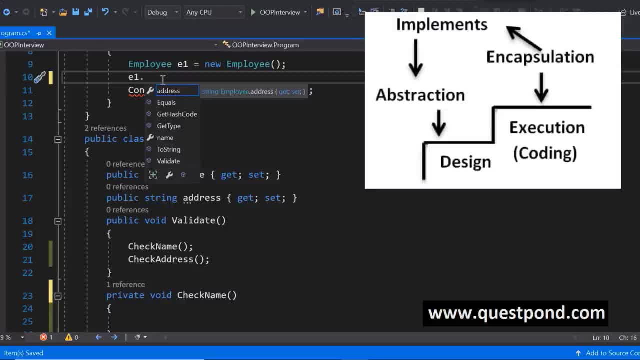 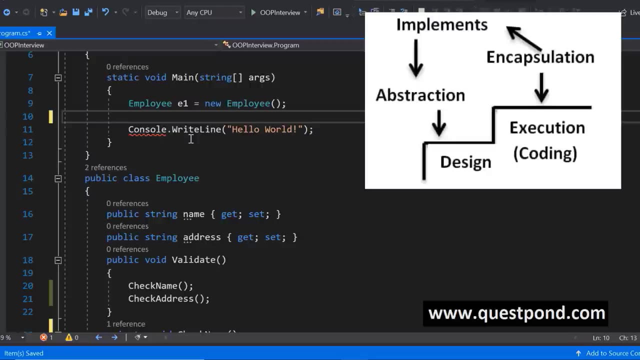 Now, if you see, I only see what is necessary. I see the name, I see the address, I see the validate, but I don't see check name and check address, right. So abstraction, abstraction is nothing but it is a design thought process or it happens during the design phase. so when you get the requirement in your, in your technical document, 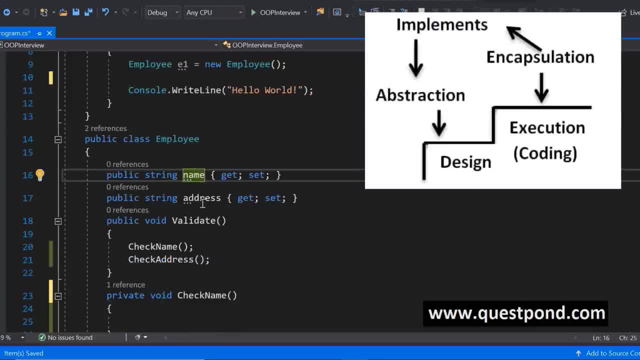 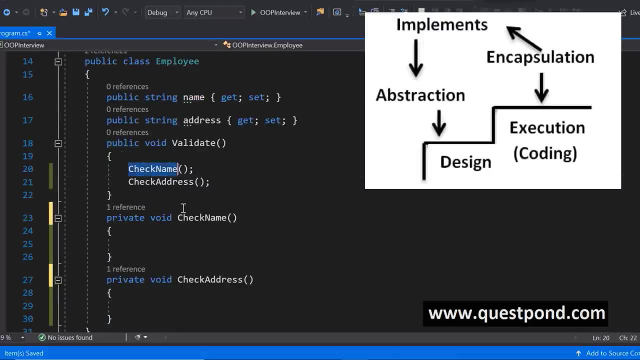 right. you say that you, in your class diagram, you say that what are the public properties? you decide, you know what are the public methods, public properties and public classes which has to be exposed outside while implement, during implementation or during the coding phase. the developer needs more functions, you know, to complete the abstraction or the design. 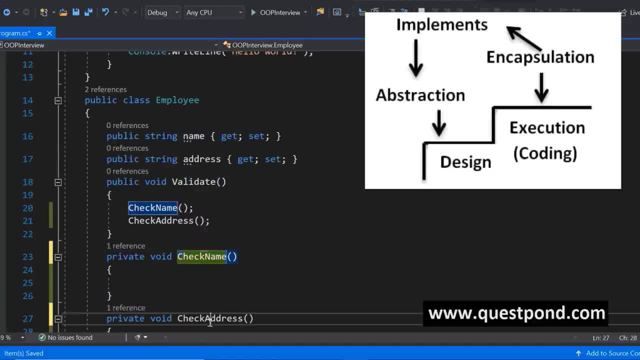 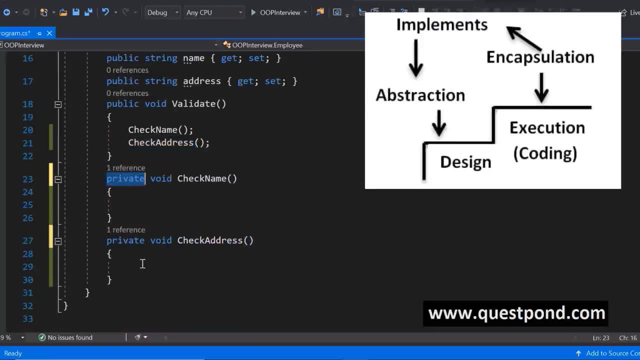 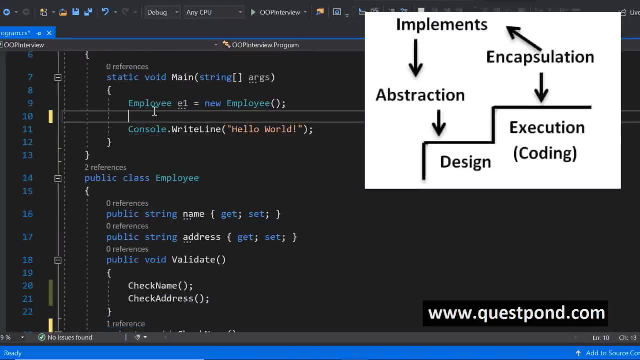 right The thought process. So He creates more of these functions and he needs to use the access modifiers like private, public and protected- to implement encapsulation. so what we can say is that abstraction happens during the design phase. so just trying to put a more appropriate answer: abstraction. 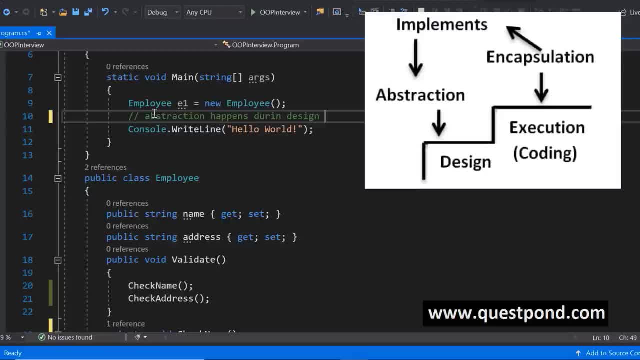 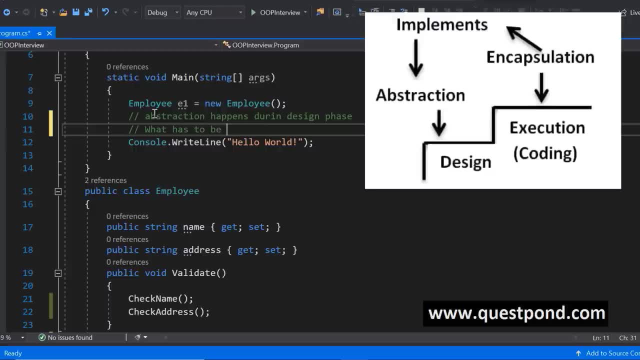 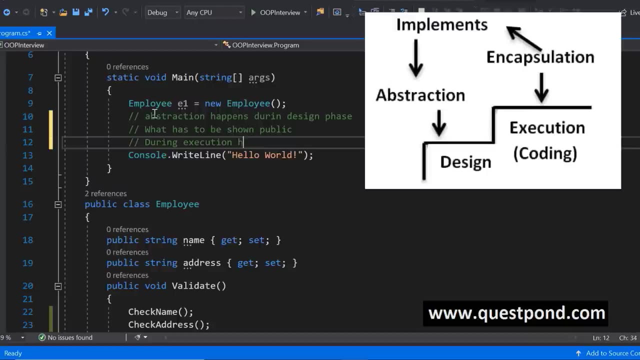 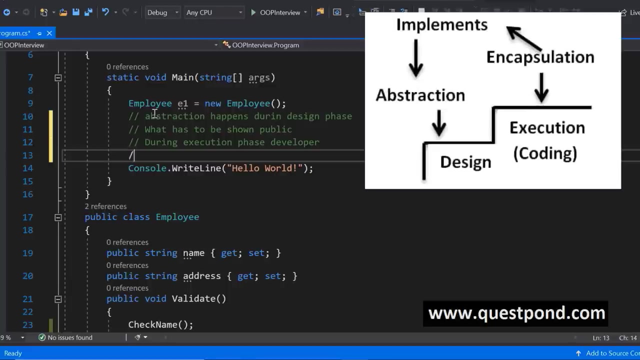 happens during design phase, right? so in the design phase you say that you decide what has to be shown- Public Right- and during execution phase. during execution phase, developer uses encapsulation. when I say he uses encapsulation means he uses the private and public and protected access modifiers. 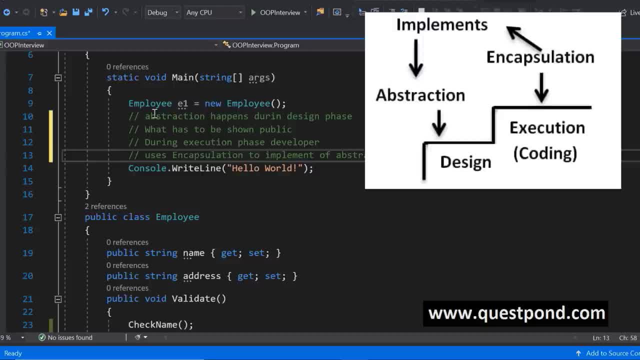 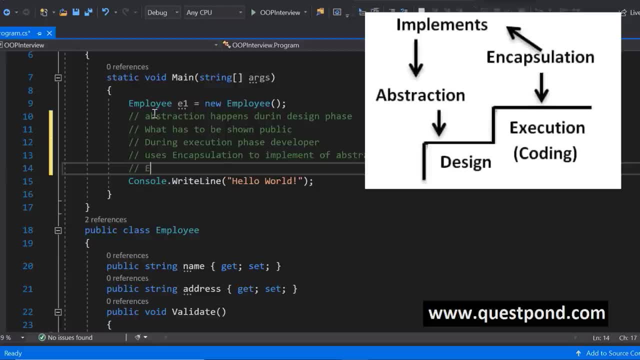 to implement the thought process of abstraction. so you know, one more thing which you can really put ahead before the interviewer is encapsulation. encapsulation implements abstraction, right? so just again summarizing the answer: abstraction means show only what is necessary. encapsulation means height, complexity. abstraction happens during the design phase, so initially when 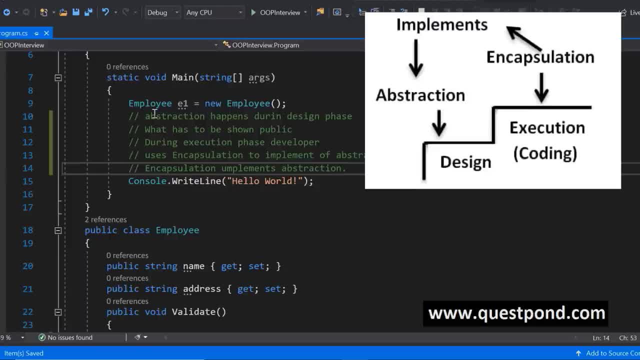 you say that you want to design the employee class, you decide. you know what is what has to be public But why. the developer goes to the execution phase. you know he needs to create more functions and those functions have to be hidden right, or else you know the the object will look. 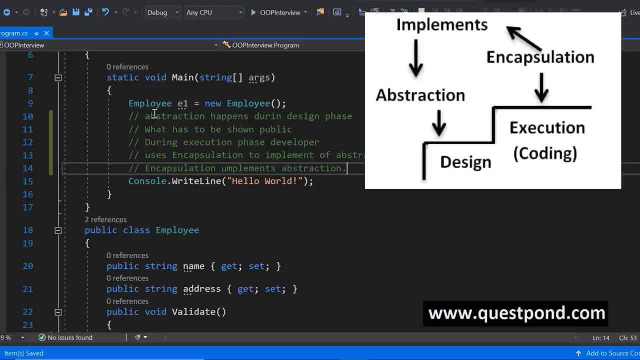 very complex. so encapsulation happens during the execution phase and encapsulation implements abstraction. so abstraction and encapsulation actually complement each other, right so? so just try to you know, when you, when you give the answer, just try to emphasize that abstraction and encapsulation complements each other and encapsulation implements abstraction and abstraction. 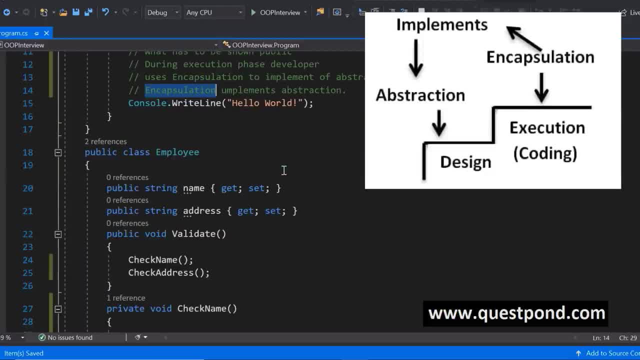 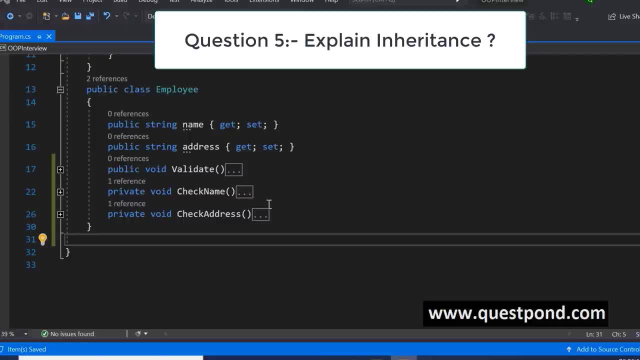 happens during design phase and encapsulation happens during, or it's executed during, the coding phase. right, explain inheritance. inheritance is one of the properties of object-oriented programming wherein you can define a parent and a child relationship between two classes. so, for example, you can see this is an employee class out. here you can go and you can create. 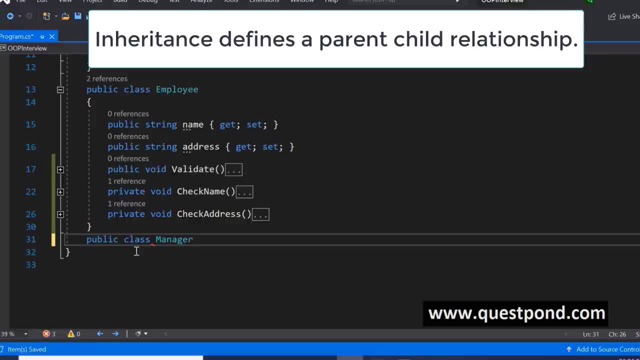 a new class. This class is called as, let us say, manager. so this manager will have all the properties and the methods of the parent class. so to do inheritance you will use colon manager inherits from employee. so now what happens is you get all the properties of the parent. 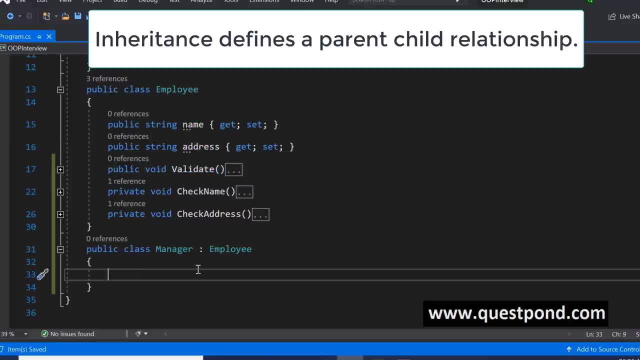 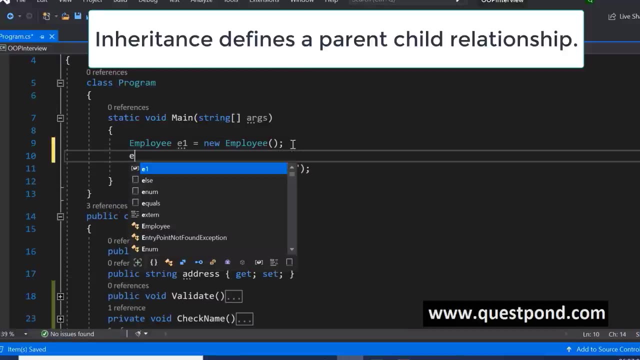 class, the methods and everything. but you can go and you can define your own methods in the child class. so you can, you can, I can go and I can say here: manager does management right. So you can see, now, if I create the employee class, I will, I will get X methods, X properties. 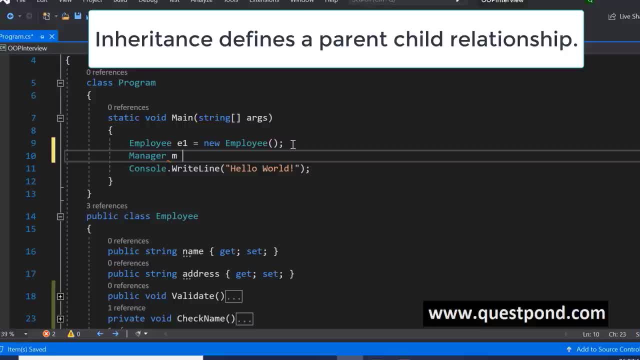 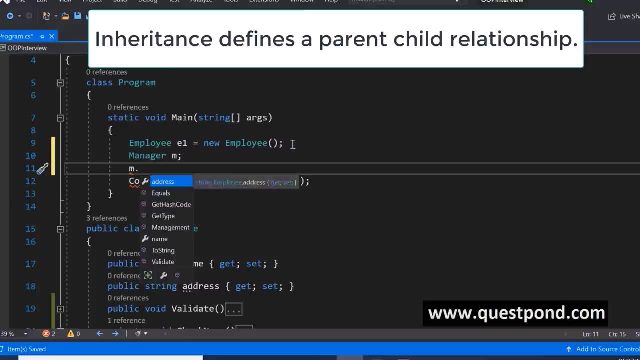 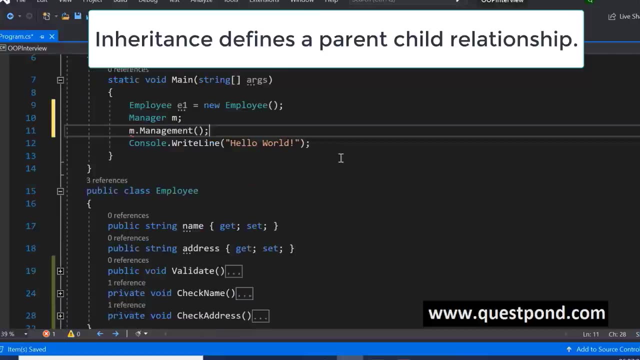 right. but if I create the manager class right, the object of the manager class, I will get all the properties and the methods of the parent class. but, as well as you know, the manage, the manager class, has its own extra methods, like management. so inheritance is nothing but. 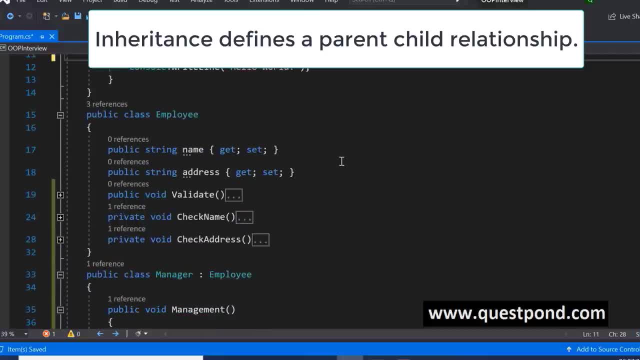 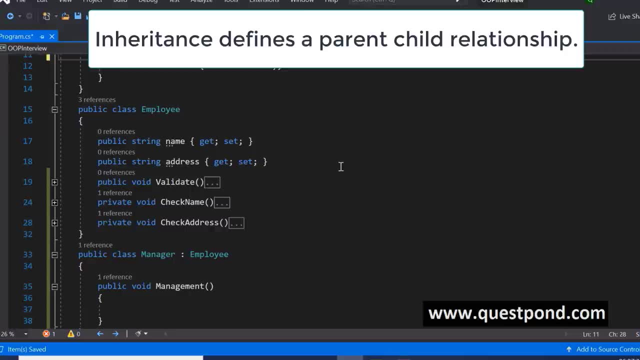 It defines a parent and a child relationship between two classes. Now remember that in the interview a lot of times you know this question can also be tweaked and the interviewer can ask you: what is a is a relationship? so is a relationship. is again a parent, child relationship is a relationship. means manager is a child of employee, so a 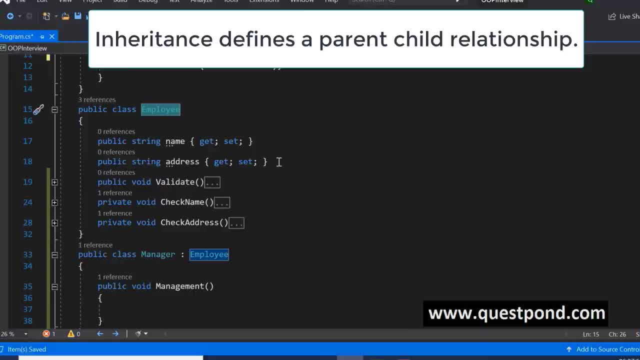 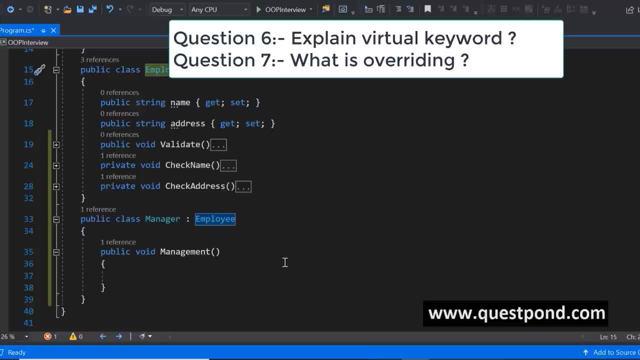 lot of times, you know, this inheritance question is also tweaked by asking that: what is a? is a relationship? What is the use of virtual keyword or what exactly is virtual methods? This question can also come in a tweaked fashion wherein the interviewer can ask you explain the concept. 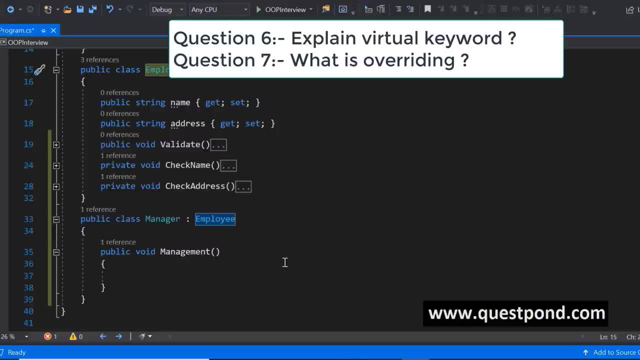 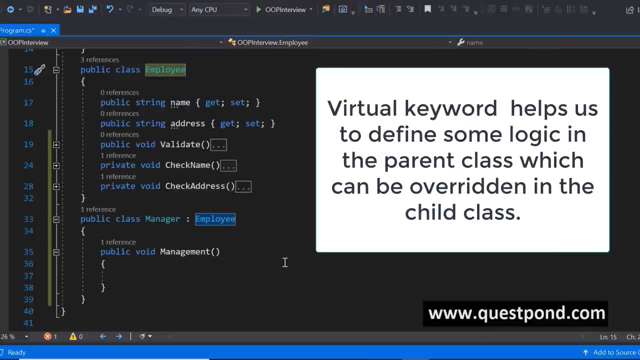 of overriding, Overriding virtual keyword, virtual methods? the answer lies in the same concept. A virtual keyword helps us to define some logic in the parent class which can then be overridden by the child class. For example, we can see that we have this class Employe: 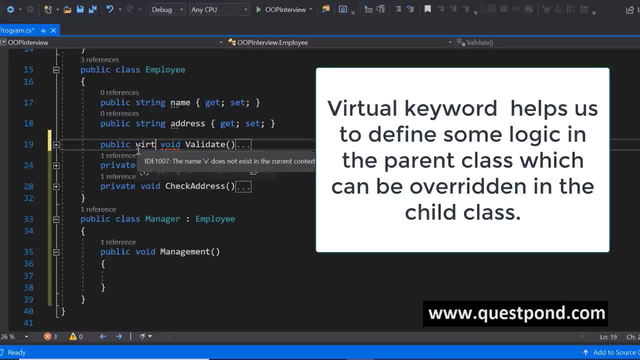 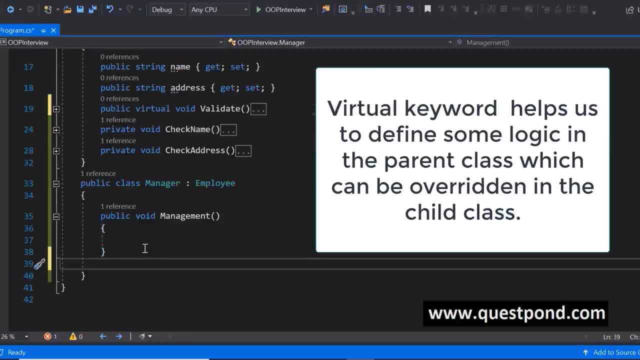 and say that this method as virtual. as soon as we give this word virtual out here, you can go to your child class, for example, this manager is inheriting from the employee. the manager becomes the child class. We can go here and override, validate The employee. 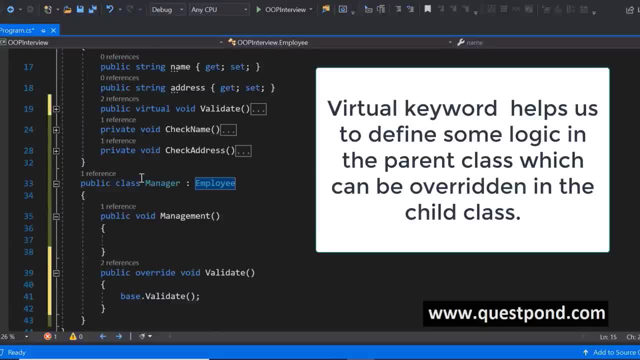 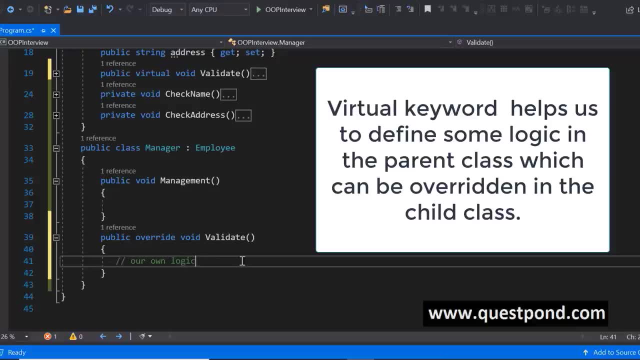 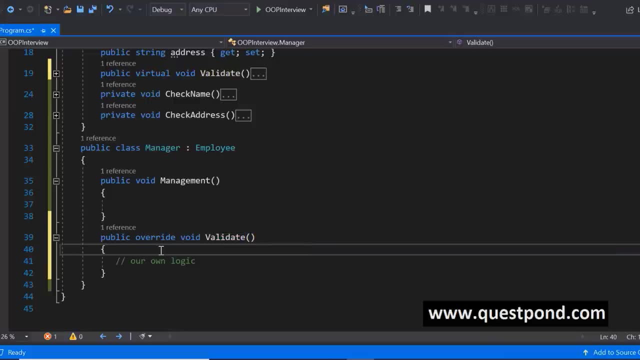 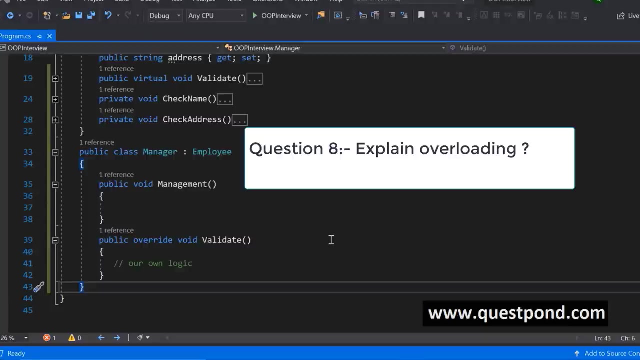 class will have certain functionality, but we can override here with our own logic. Virtual keyword helps us to provide some implementation in the parent class which can later be overridden in the child class. This concept is also termed as overriding. One of the connected questions which comes with overriding is: what exactly is method? 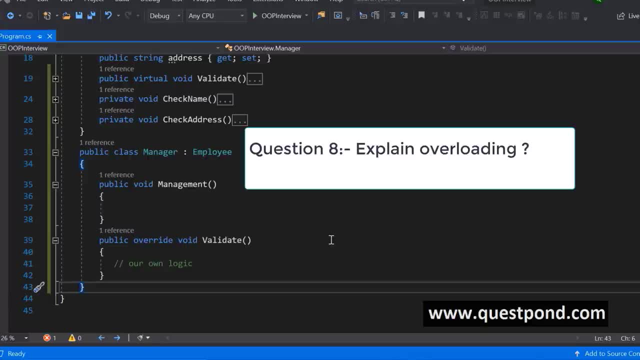 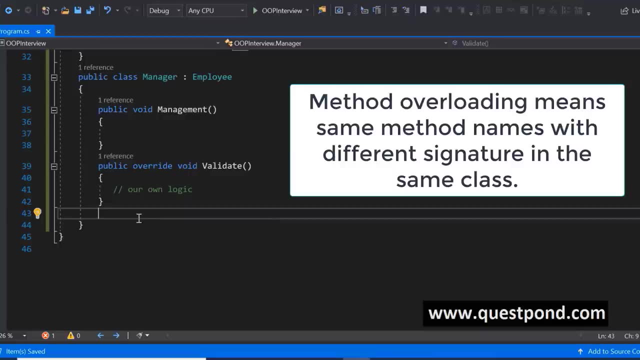 overloading. This question can come in a tweaked fashion. what is the difference between overriding and overloading Method? overloading means you will have the same method names with different signature. We have a validate method out here and we will have one more method here called as validate, but it has an input. This is validate without. 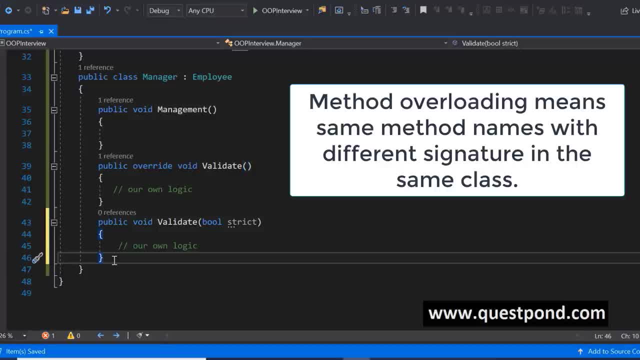 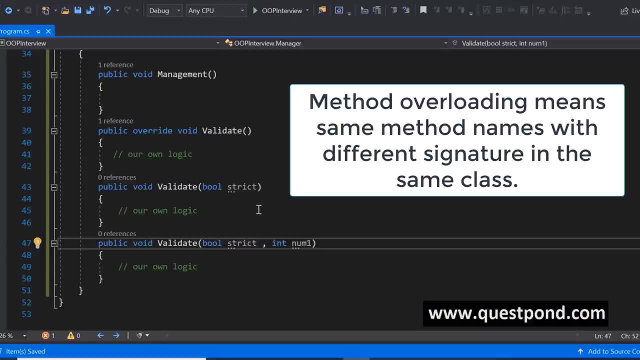 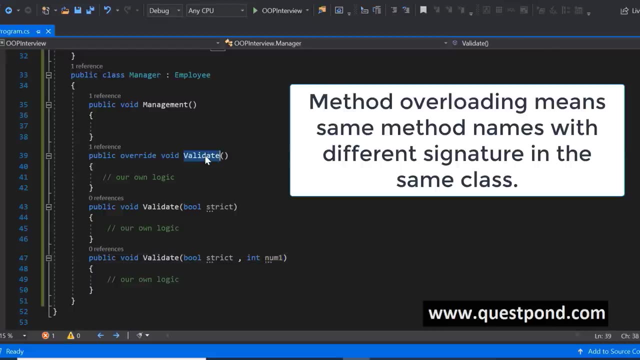 any inputs and this is validate with an input. We can have one more validate where we say some another input. The validate method in this class, in the manager class, has been overloaded three times. One is: it has validate without any signature. another one: it has validate. 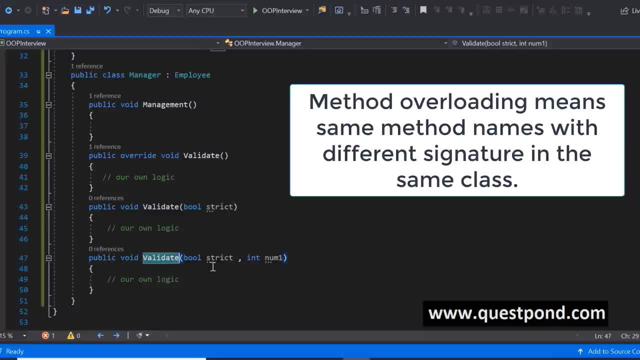 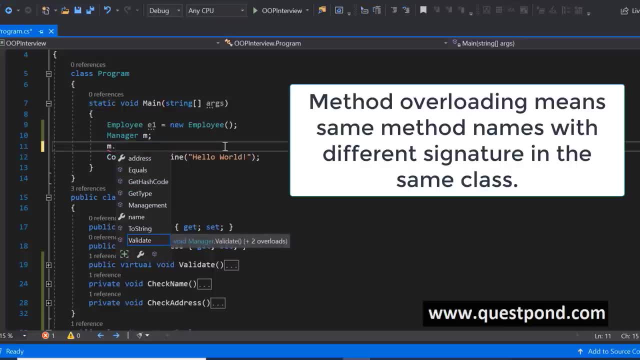 which has a boolean input, and there is another validate, which it has two more inputs. Method overloading means in the same class you can have same method names. 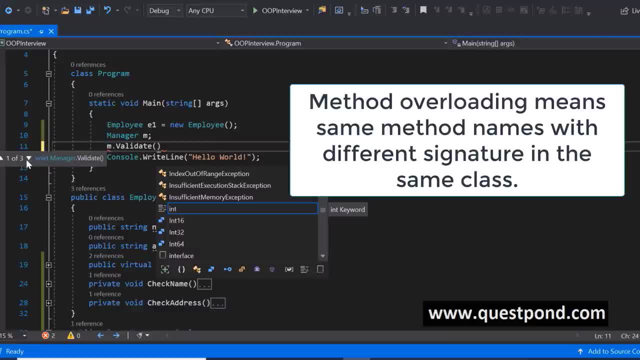 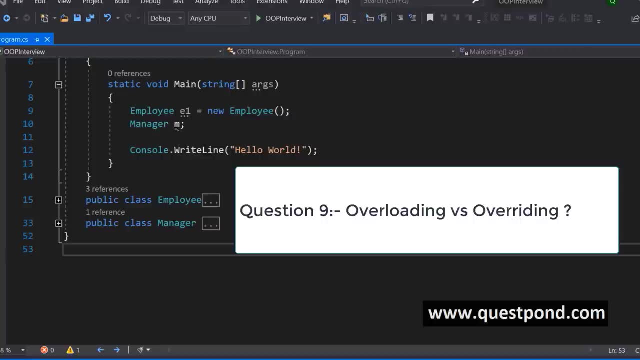 with a boolean input and validate with two more inputs. this is termed as method overloading. Also, let us quickly summarize the difference between overloading and overriding. I am not. 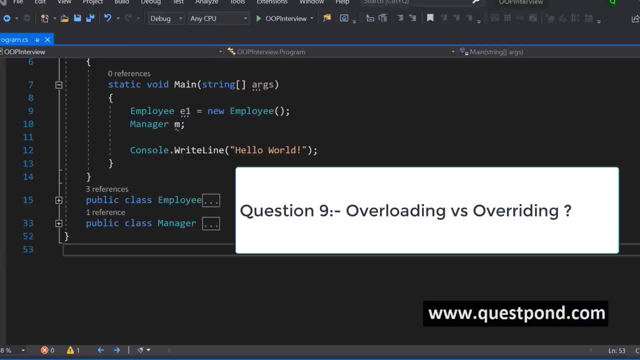 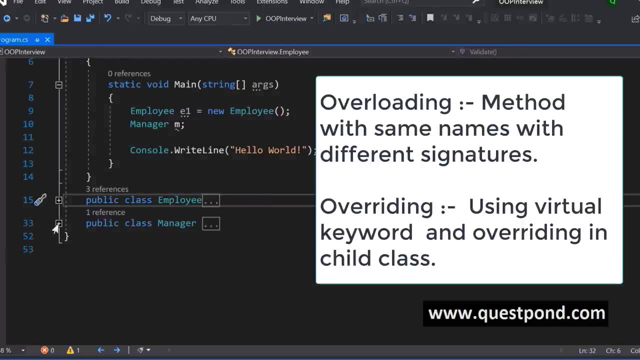 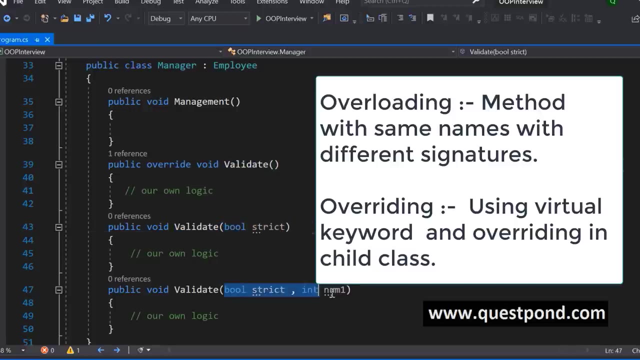 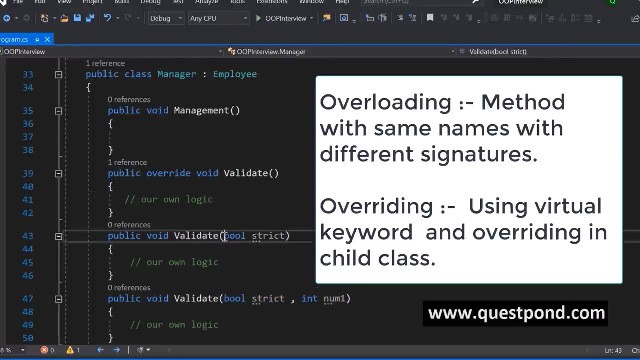 sure why this question comes up, because it is comparing Apples with Mangos, but let us try to atleast put some sentence around it. thop th Records. then in the same class you have the same method names with different signatures. But when we talk about method overriding, it comes in a parent-child relationship, so there, 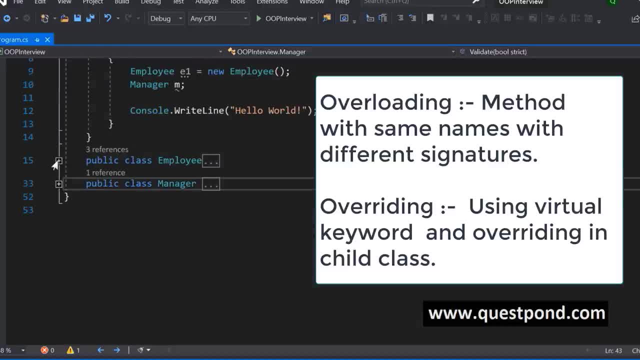 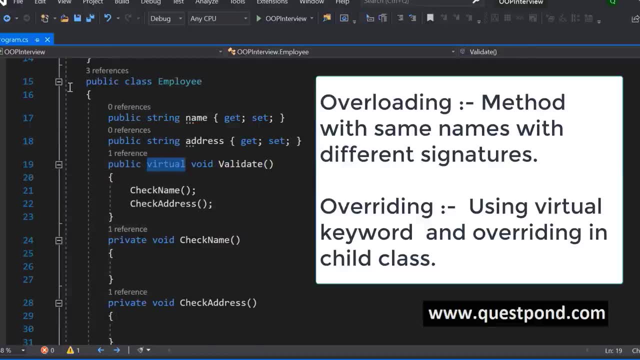 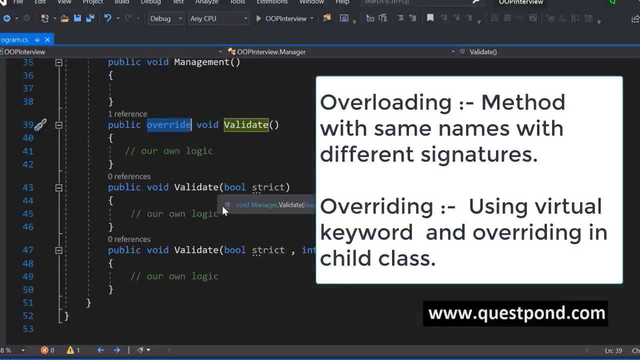 should be a parent-child relationship or else method overriding does not exist. For example, here we have an employee class, it has a validate method which is marked as virtual, and then this virtual method is later overridden by using the override keyword In method overriding. we are actually using this override keyword and there is a parent-child. 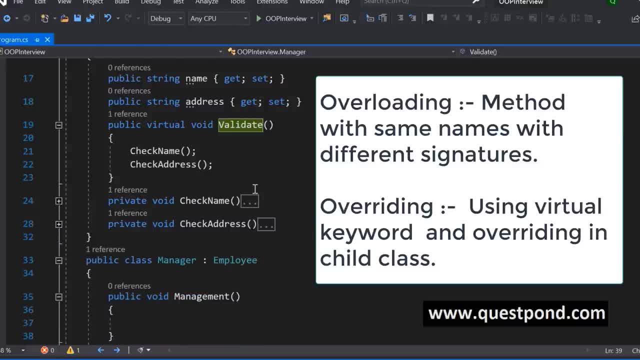 relationship where in the parent class has a virtual method. This is a parent class, it has a virtual method and later the child class uses the override to override it. Method overriding makes more sense when you talk about parent-child relationship, when you talk about a parent method being overridden, when you talk about method overloading in. 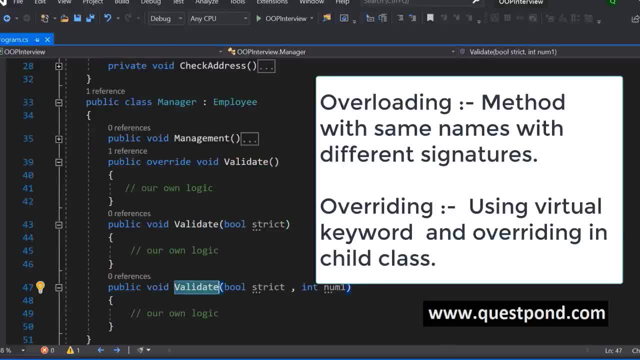 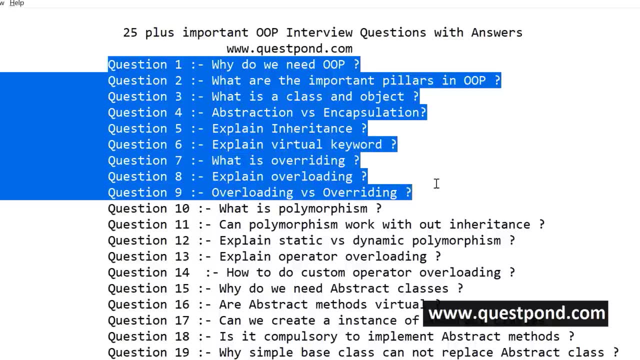 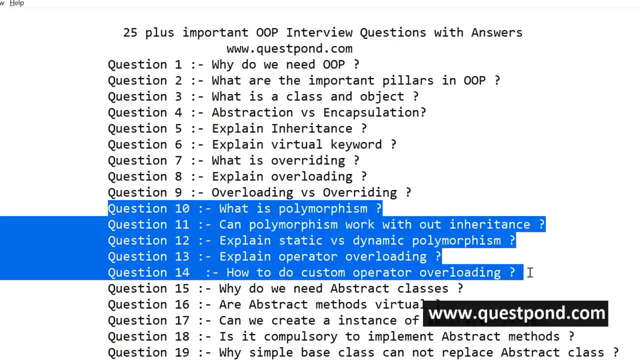 the same class. you have the method names with different signature. First thing, congratulations. we have completed approximately 20 minutes and we have completed nine questions. The coming four questions, that means from question number 10 till question number 15, is completely on polymorphism. 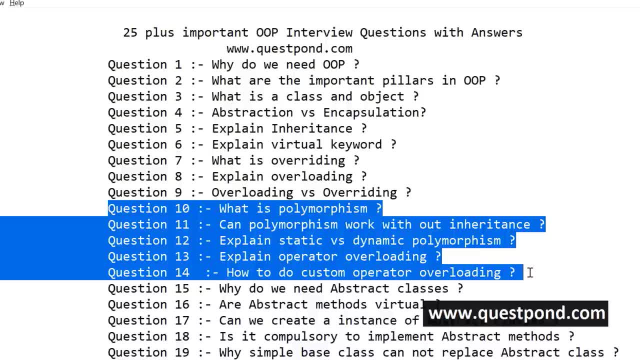 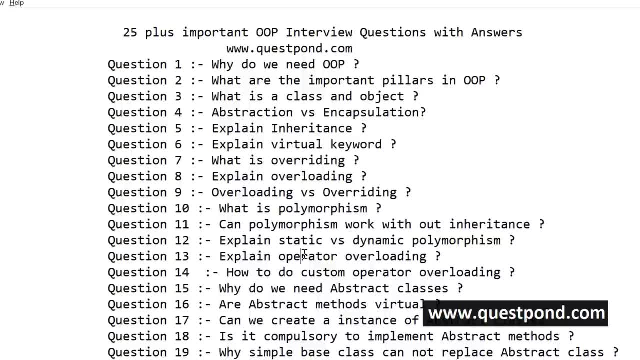 No object oriented programming interview is complete without a question on polymorphism. So we are going to talk about what is polymorphism, what is static polymorphism, what is dynamic polymorphism, what is operator overloading, and so on, Before we move ahead with the questions on polymorphism. if you are really liking this, 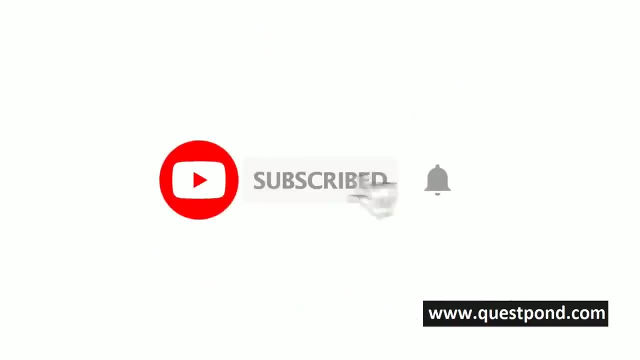 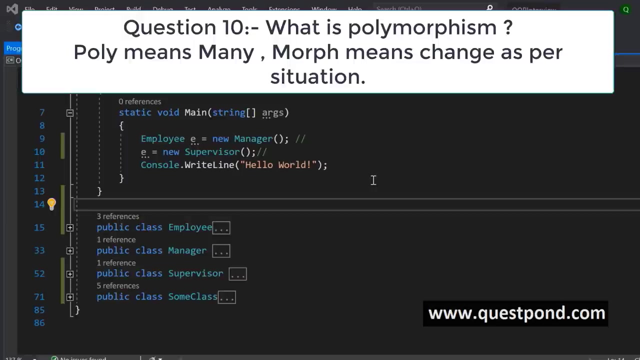 video. please go ahead and subscribe to this channel. Please hit that bell button out there so that whenever we upload an interview question video, you get an indication. Explain polymorphism, If you see the word polymorphism: poly means many and morph means change as per situation. 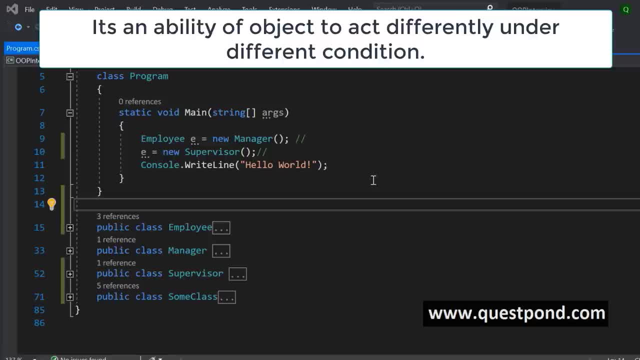 Polymorphism is nothing, but it is an ability of an object to act differently under different conditions. For example, you can see the code on the screen here. you can see this employee in this line number 9 is acting like a manager, And the same employee, object E, in line number 10 is acting like a supervisor. 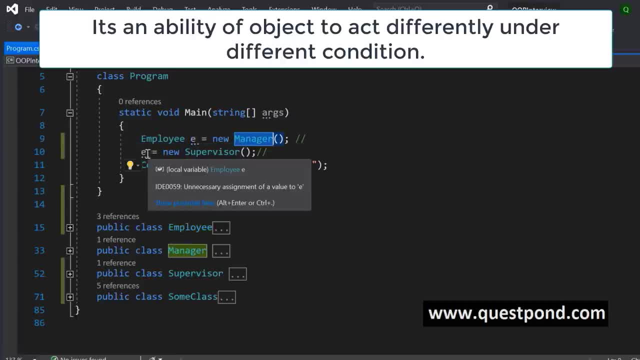 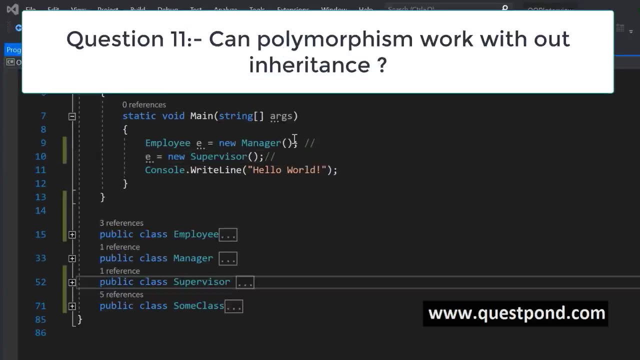 In line number 9, it is becoming a manager and then dynamically, in line number 10, it is becoming a supervisor. This is termed as polymorphism, the ability of an object to act differently under different conditions. Can we implement polymorphism without inheritance or without parent child relationship? The 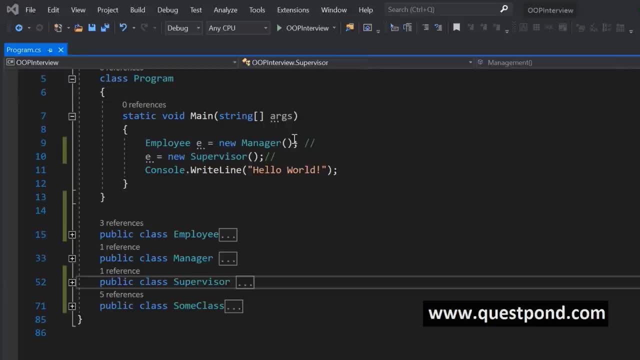 answer is absolutely no. This question is specifically thrown to you from the interviewer, from the point that: do you understand polymorphism in detail? For example, in our case here, if you see this, employee E is becoming a manager in line number 9 and in line number 10 it is becoming a supervisor, because both the manager class is inheriting. 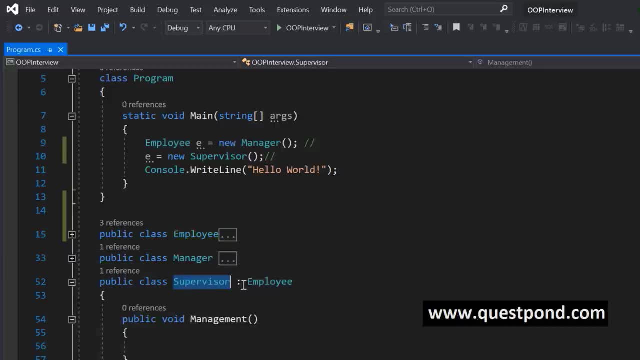 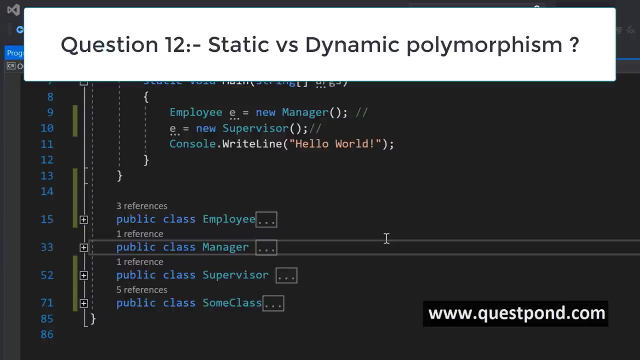 from the employee as well. as the supervisor class is inheriting from the employee, For example. if you remove this inheritance out here, you will see that C sharp will start throwing exceptions. To implement polymorphism, inheritance is a must. What are the two kinds of polymorphism in C sharp? 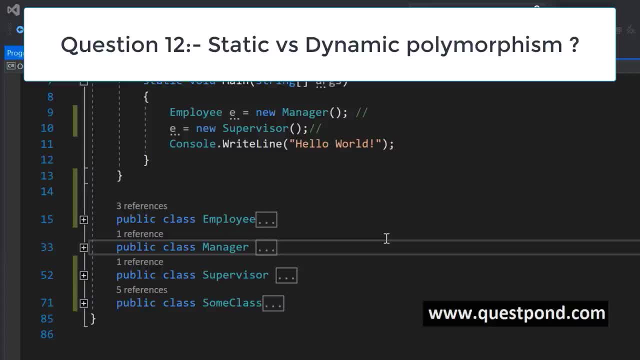 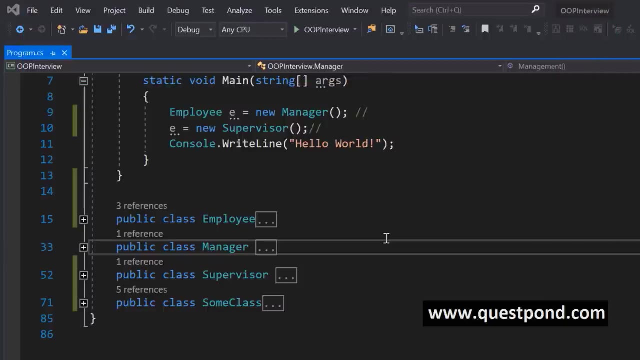 The two kinds of polymorphism in C sharp are static polymorphism and dynamic polymorphism. Many developers also term them as run time polymorphism and compile time polymorphism. Runtime polymorphism means dynamic polymorphism, Dynamic polymorphism, and compile time means static polymorphism. 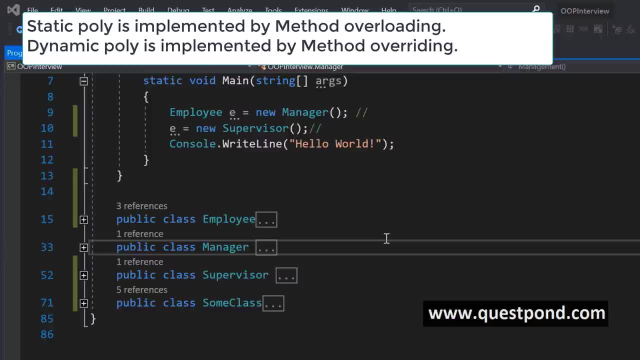 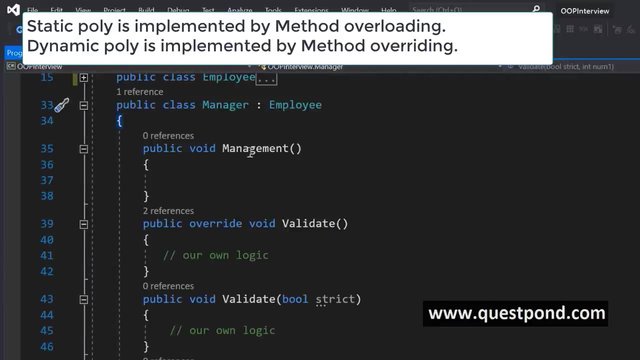 Static polymorphism is implemented by method overloading, while dynamic polymorphism is implemented by overriding, Static polymorphism is implemented by method overloading. We have this manager class, which has a validate method, and this validate method one is: we have a validate method, Not a signature, and then we have a validate method with a signature, with one signature. 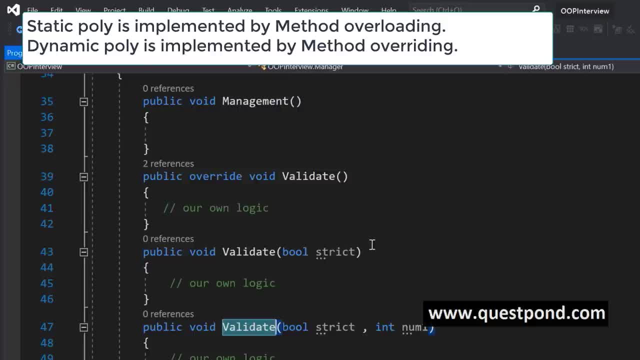 and then we have a validate method with two signatures. This is static polymorphism. This will be checked during the compile time means when I hit the build. at that time it will be checked. When you talk about runtime polymorphism or dynamic polymorphism, that happens in a parent. 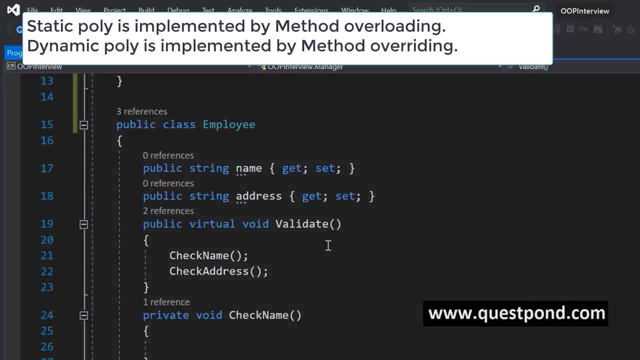 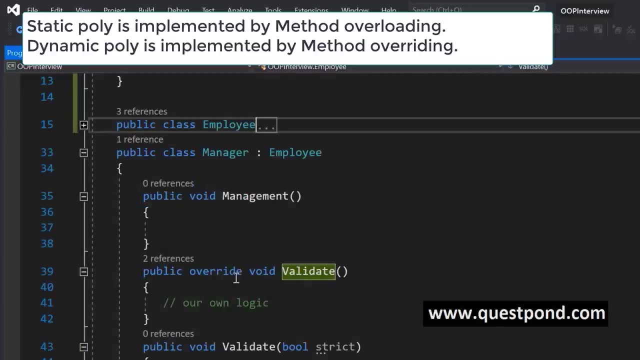 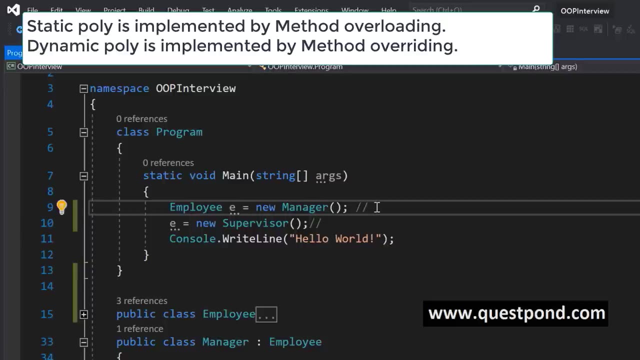 child relationship. In a parent child relationship, for example, we have to use the virtual keyword. so this is the virtual keyword validate. Then the manager goes and inherits and overrides this validate. so what I can do now is I can say dynamic polymorphism, employee E can point towards manager and he will call here validate. 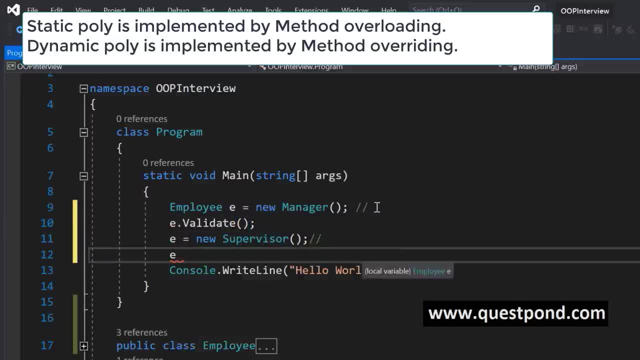 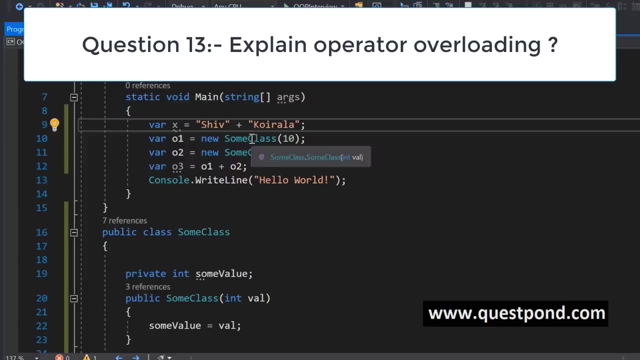 and the same employee can point towards supervisor and he can call validate. This is runtime polymorphism. Method overriding is runtime polymorphism. Operator overloading is static polymorphism. Explain operator overloading. Operator overloading is a concept of polymorphism where you can redefine operators like the: 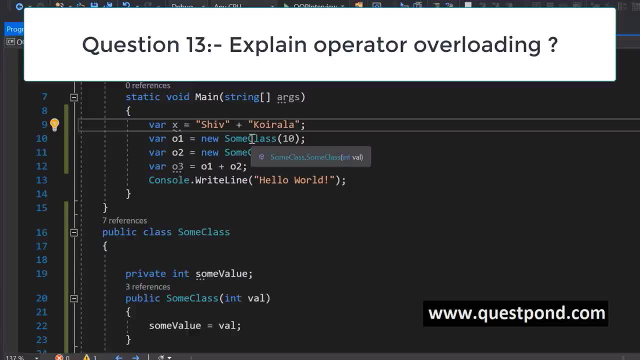 plus sign and the minus sign and the multiplication sign with additional functionalities. For example, you can see inbuilt inside NET by default. if you see right, when you say, when you use the plus sign with strings, for example, you can see in this line number 9, I am saying: 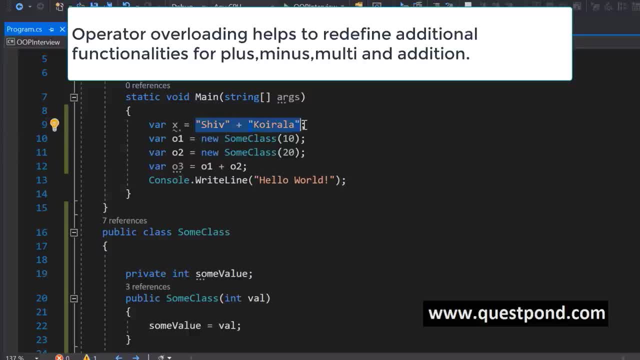 that This will do a concatenation. this will concatenate both the strings. but if I go and if I say here 1 plus 2, if I say this, then this will actually do an arithmetic addition By default itself. you will see polymorphism in NET. but now definitely the next cross. 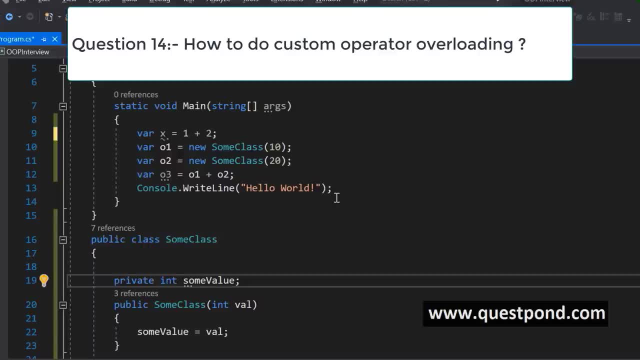 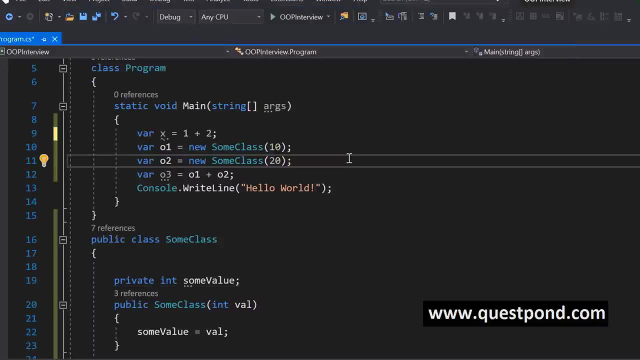 question from the interviewer can be: what if you want to go and implement your own logic of polymorphism or do a custom operator overloading, For example? you can see here I am creating an object of some class called as O1 and then I am creating another object called as O2. what if I want to go and say O1 plus O2? I want. 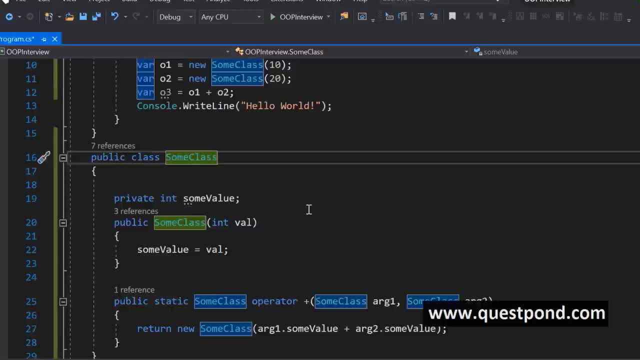 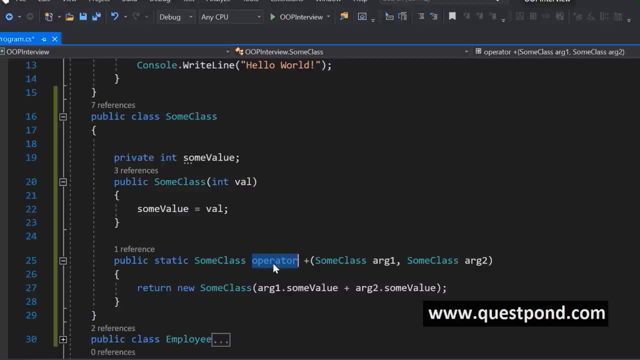 to and add both of these objects. For that, what you do is that you have to go ahead and use this operator, overloading keyword here, operator, so we can see operator and the plus sign and this complete method, this method, you have to define it as static. 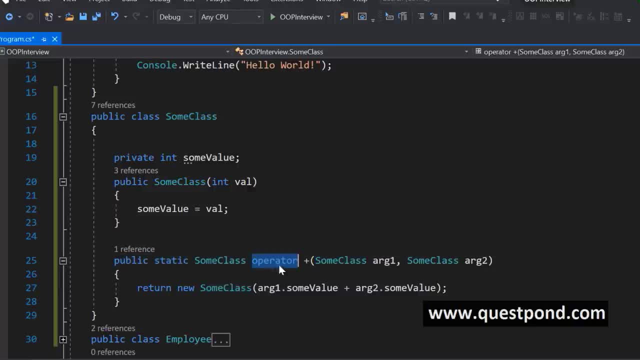 see public static, some class operator and you pass the first instance of some class, you pass the second instance of some class and then you define your logic. what you want to do Here, what I am doing is I am adding these two numbers out here of some value. 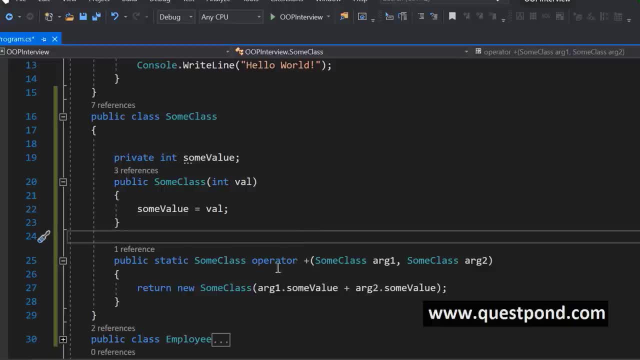 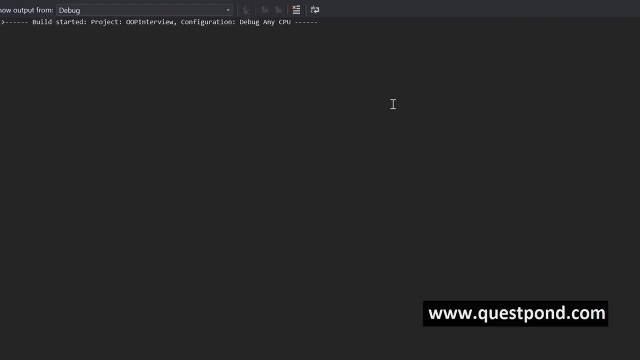 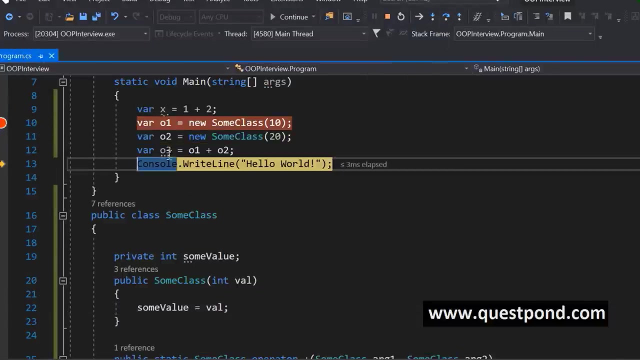 If you want to do a custom operator overloading then you need to use the operator keyword. If we run this application out here, in this application two objects will be added. so O 1 plus O 2 will give you O 3, and in O 3 you have 10 plus 20, which is 30. In the O 3 object, 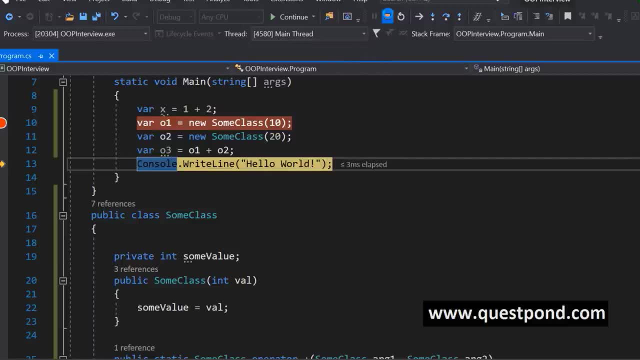 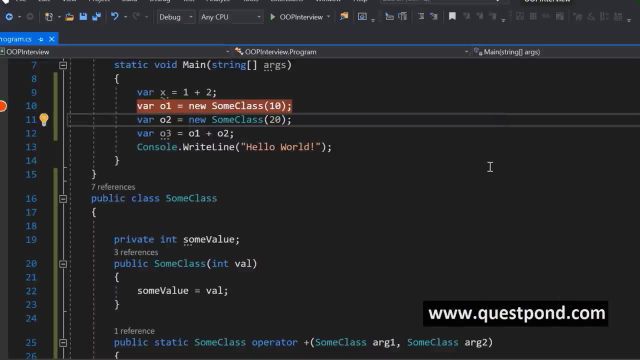 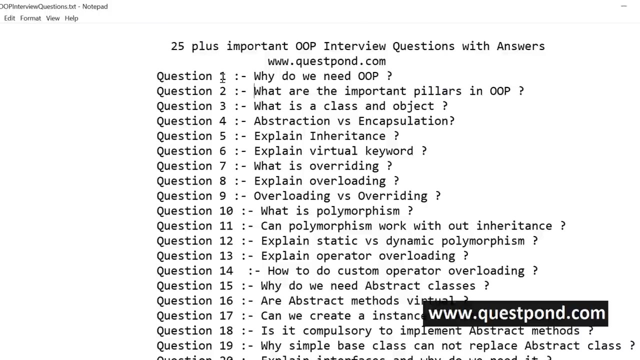 of some value is 30.. Operator overloading means the ability that you can overload an operator with additional value functionalities and if you want to do custom operator overloading, then you need to use the operator keyword. Congratulations to you and congratulations to me as well. we have completed 30 minutes. 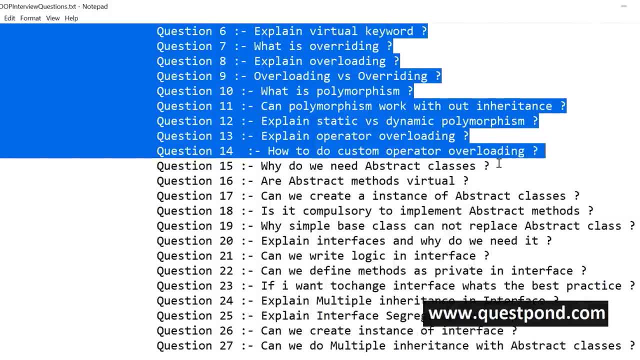 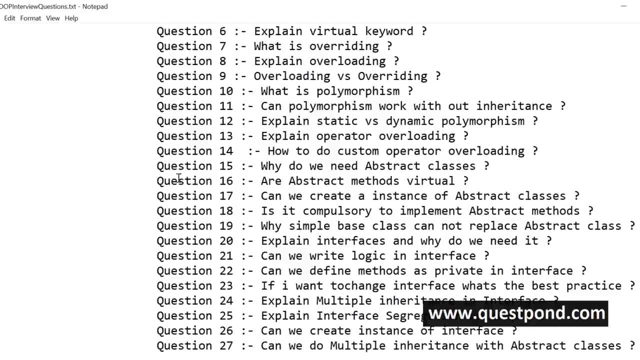 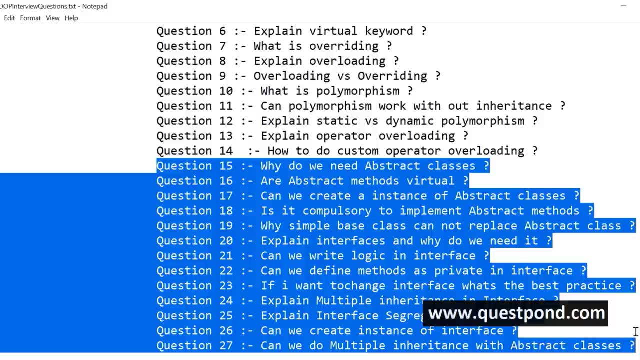 of this video. we have completed 14 questions till now, From question no 15 till question no 27. these questions are on abstract classes and interfaces. No object oriented programming interview is complete without a question on abstract class and interface. It is one of the most confusing topic. it is one of the most important topic and it's one 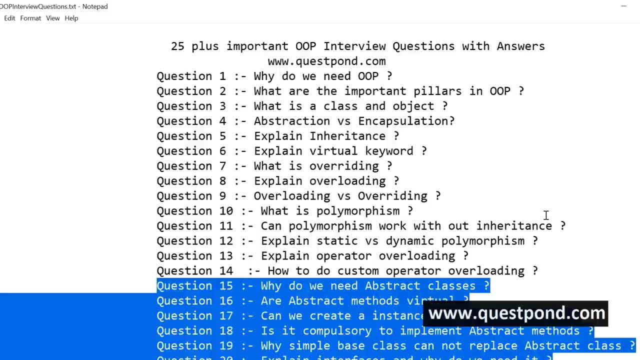 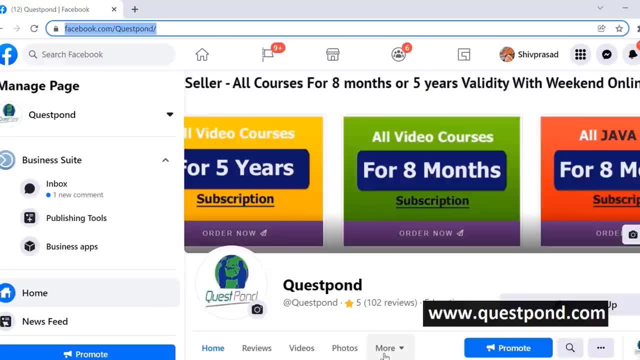 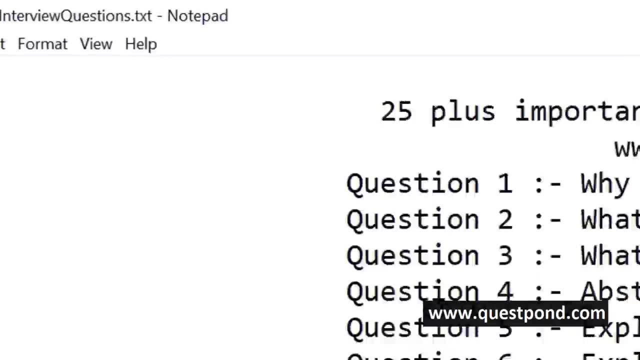 of the most loving topics when it comes to object oriented programming interview questions. Before we start with abstract classes and interfaces, a small request: if you can go to facebookcom, slash questpond and if you can say that, yes, I am on question no 14. I am on. 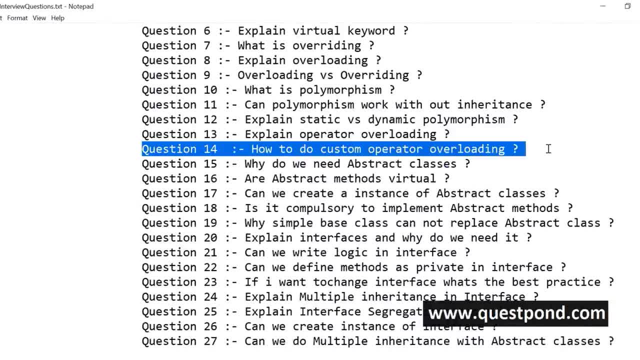 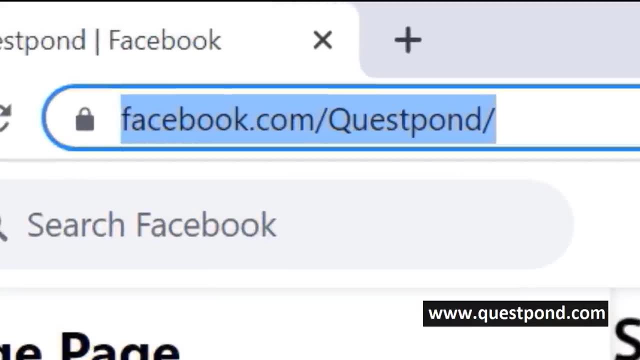 question no 15.. It just tells us that how many people are watching our video, till what limit, and this encourages us to record more videos on this channel. Please go ahead on facebookcom, slash questpond and say that, yes, you have liked this video, or you are on question no 14. you are on question no 15. you are on question no 25. that will. 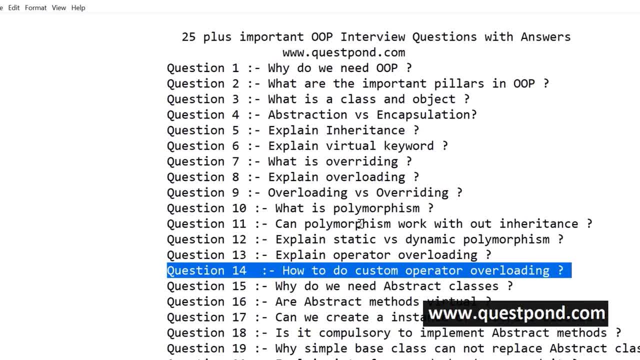 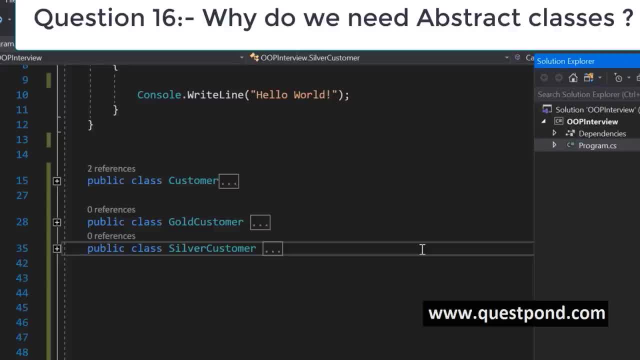 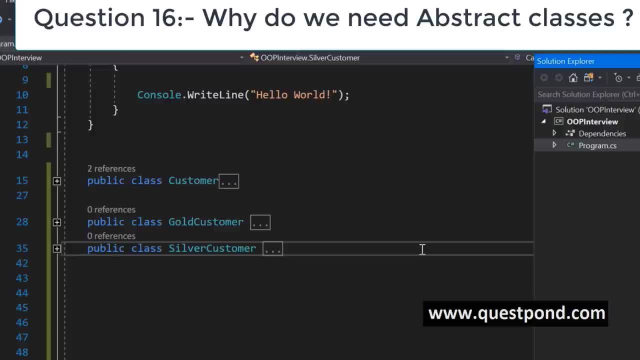 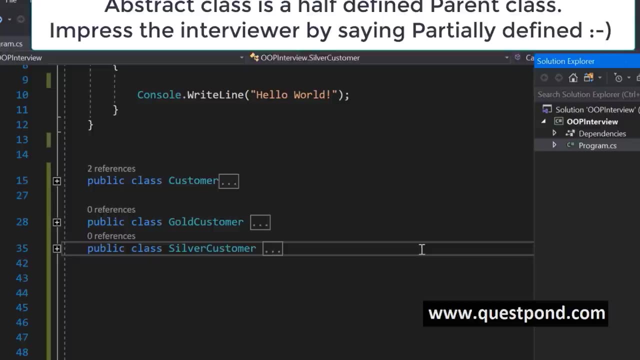 first, and then we will go towards interfaces and then we will compare the difference between abstract class and interface. So what exactly is an abstract class? an abstract class is a half defined parent class. or you can say: an abstract class is a partially defined parent class. 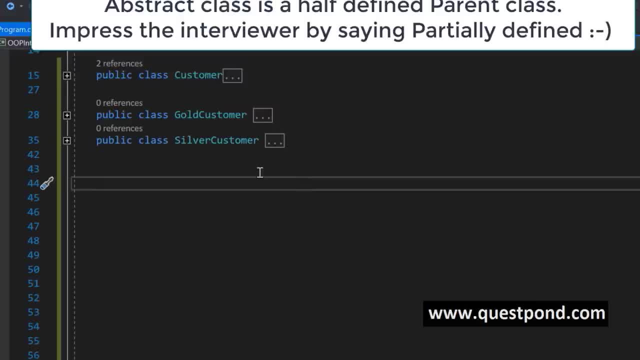 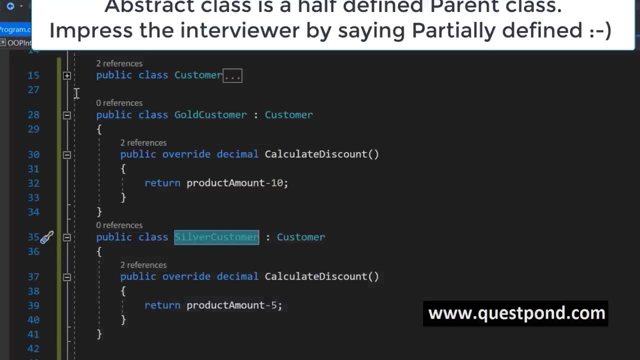 Now let us try to understand this with an example, so you can see: here I have a custom class and then from this custom class, we have two other classes which are inheriting. one is a gold customer and another one is a silver customer. Now, both the gold customer and the silver customer share lot of common properties. you 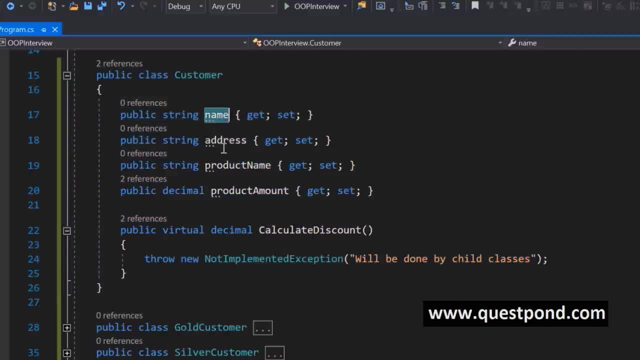 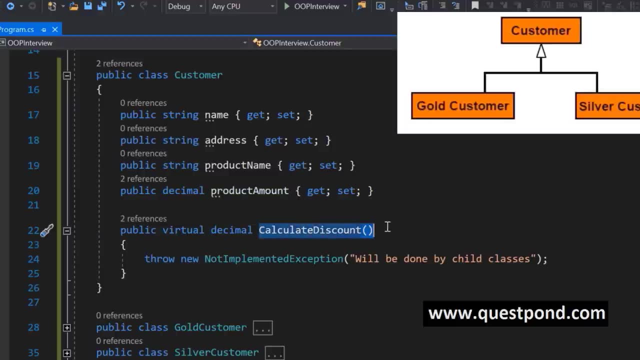 know, for example, they share the customer name, the address, the product name, the amount, right. but you can see there is a calculate discount out here and this calculate discount is overridden by both of the classes with their own name. Now, this calculate discount is overridden by both of the classes with their own name. 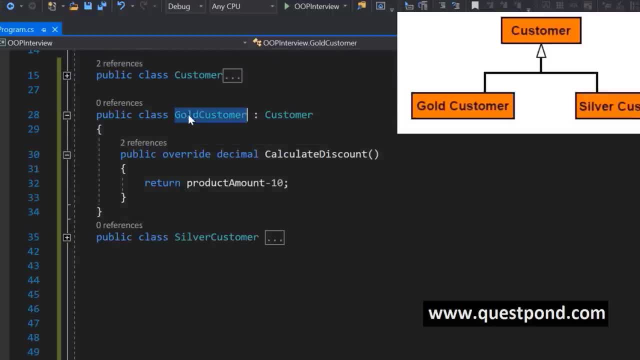 and their own behavior means, for example, if you see the calculate discount of the gold customer, it is giving a 10% of discount. if you look at the calculate discount of the silver customer, it is giving a 5% of the discount right and in the parent class. you know, because 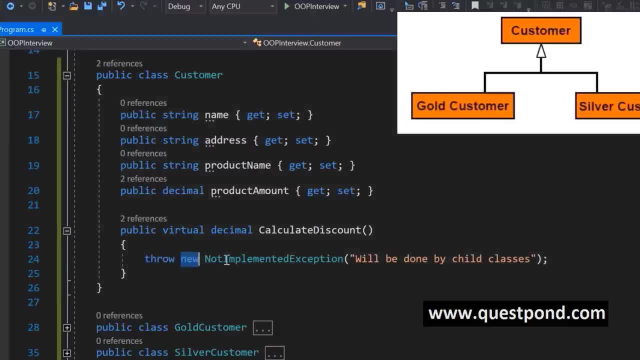 we don't have any implementation. we have said here: throw new, not implemented exception. in other words, we are saying that if anybody tries to go and invoke this calculate discount of the parent class, it will say that This will be done by the child classes. so there is no implementation. out here now the 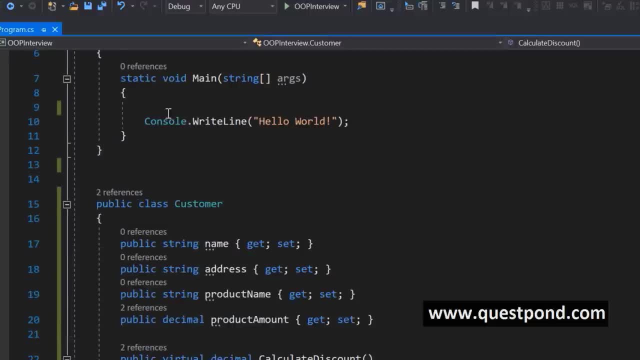 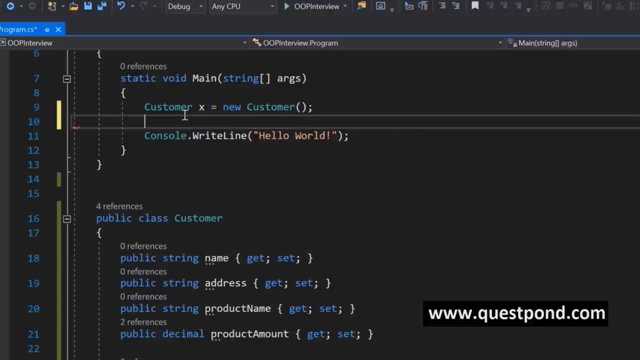 problem with this approach is right. the problem with this approach is that somebody can go and create an object of a customer class like this you can see here: somebody can go and create the object of this customer class and he will try to invoke the calculate discount. 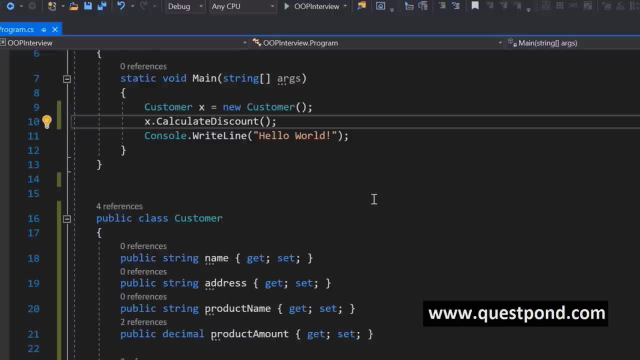 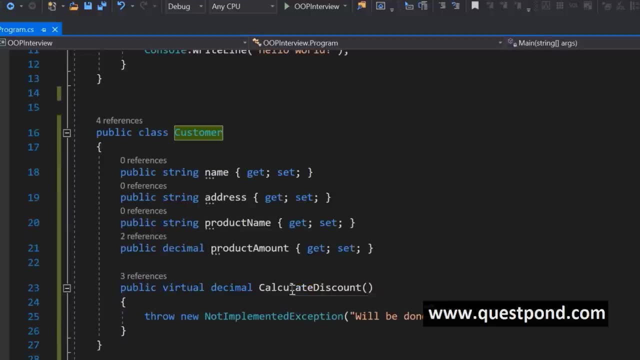 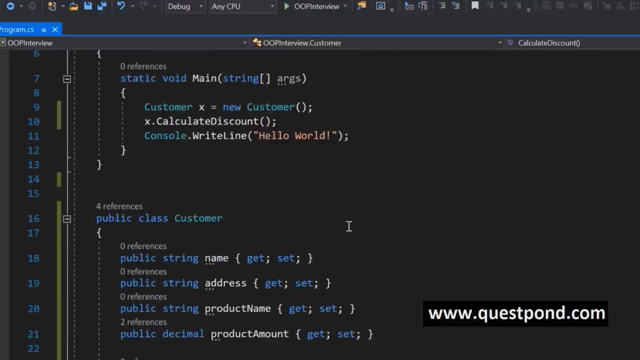 So what will happen here is we can have confusion because you have a customer class, so the developers will try to Create an instance of the customer class, they will try to invoke this calculate discount and they will get this not implemented exception, which is really bad, isn't it? now? why is this? 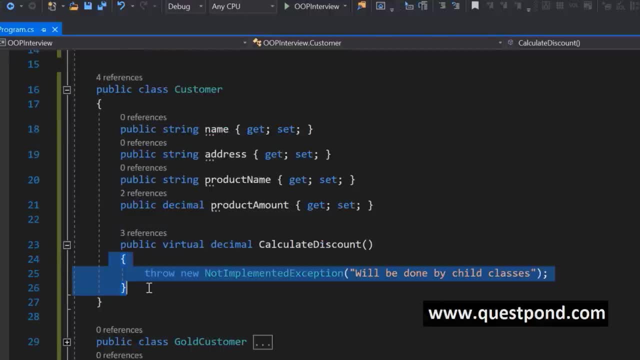 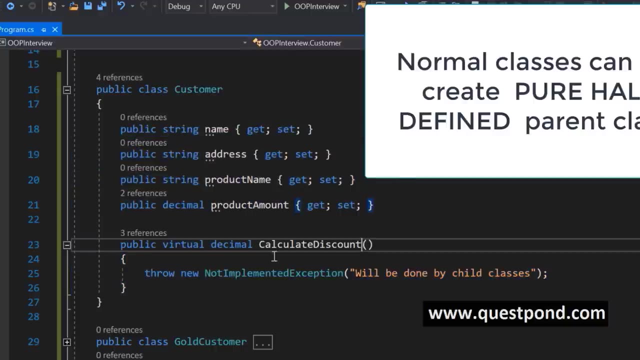 happening actually over here. you know there is no implementation right. in other words, in this customer class there is some implementation and for some of them there is no implementation. and those implementation has to be defined by the child classes. In other words, We need to create a class which is half defined, partially defined right. so for that we need 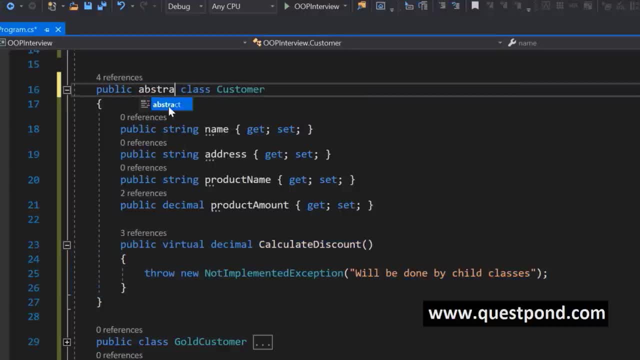 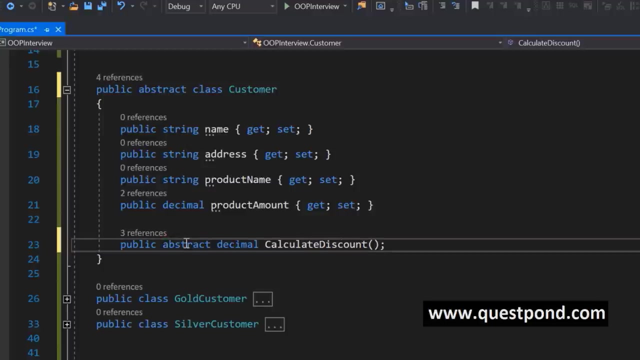 an abstract class. so we create an abstract class by saying abstract. now this method- calculate discount- is without any logic, right? so it should be half right, so in other words, there shouldn't be any logic out here. so we go and we say this as an abstract, so you can. 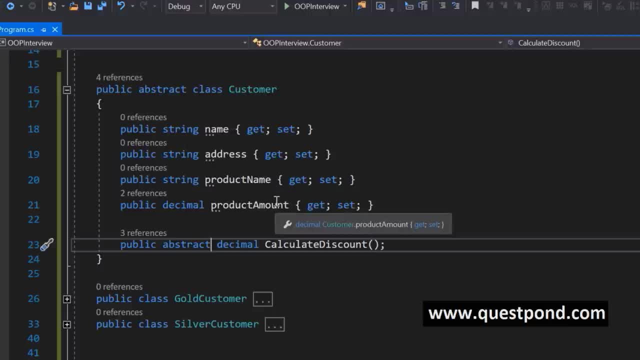 see here now. This Customer Class is half defined. in other words, the name, address, product name and amount is fully defined, but the calculate discount will be overridden by the child classes and the logic will be defined. The best part about the abstract class is that, because it is half defined, you can't 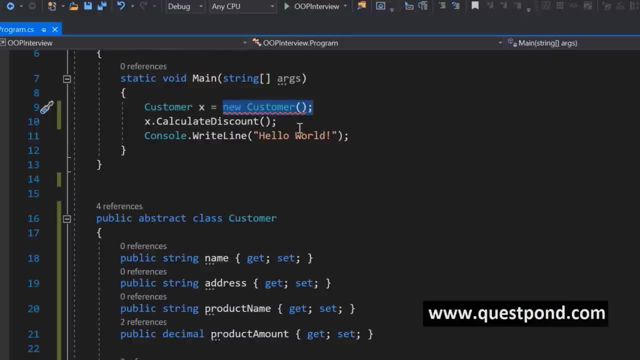 create an instance of it. So the confusion in aware you can go and you can invoke an invoken half-class and then later on you get an error Now is actually stopping you to not create an instance, which is actually very good. Just trying to put ahead what you have to speak to the interviewer: an abstract class. 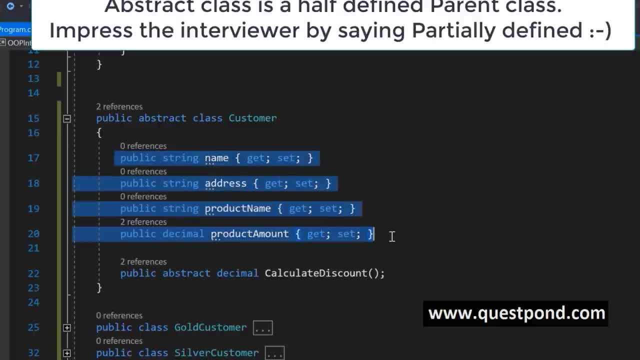 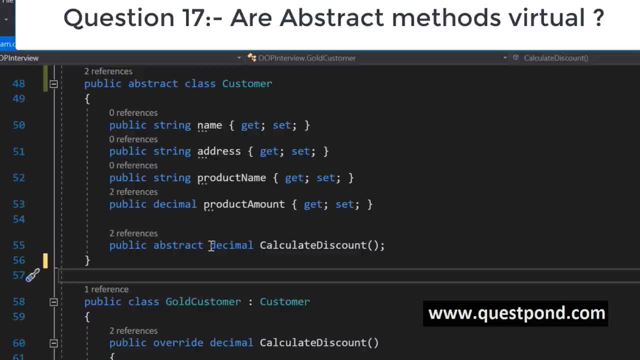 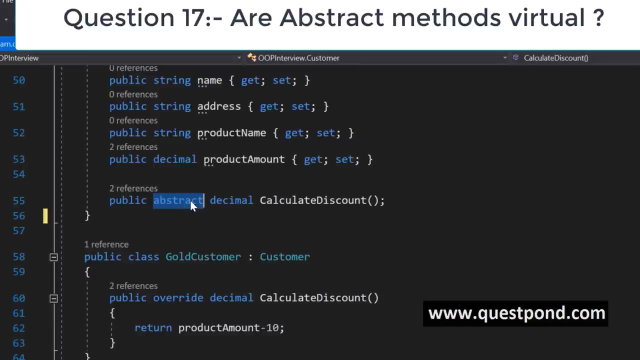 is a half defined parent class where there are some implementation which is defined and some implementation is left to the child classes to be defined. One more tricky question which comes around abstract classes. are abstract methods of an abstract class virtual? The answer is yes. In the last object oriented programming interview question I had talked about the virtual keyword. 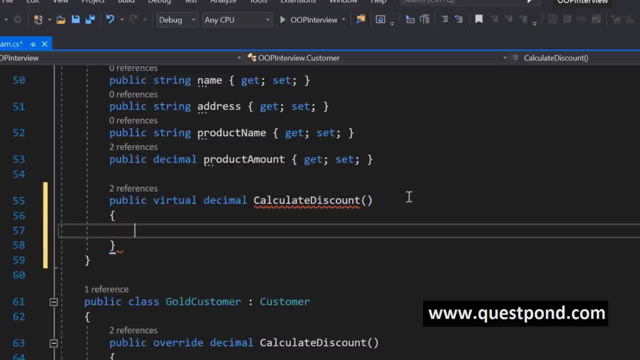 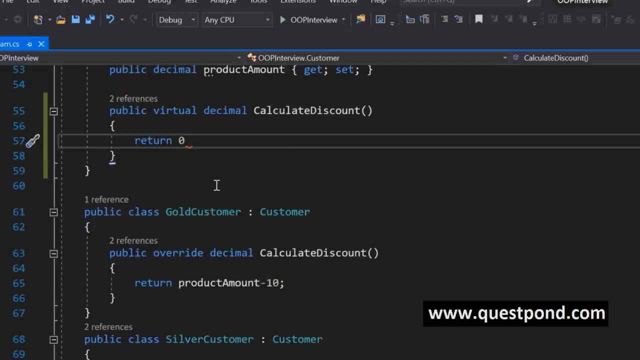 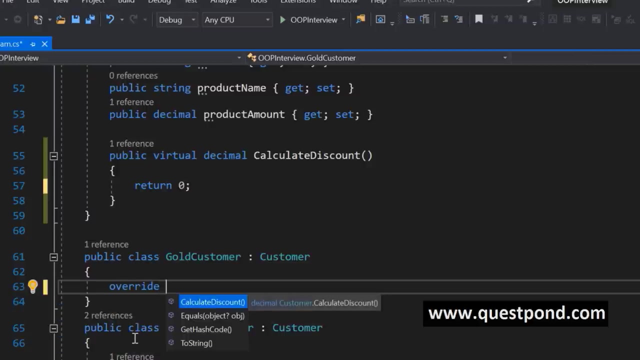 Virtual keyword. what it does is, if you define in a parent class a method as virtual like this, in the child class you can override it. In the child class you can go and say override, So You can see this calculateDiscount is seen, because this is virtual. 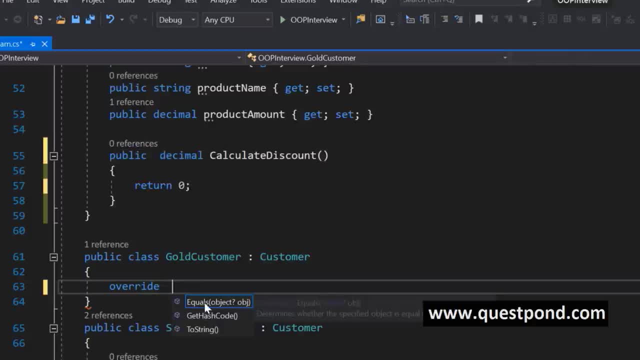 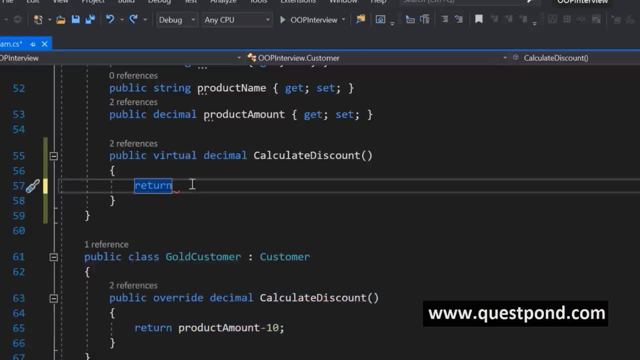 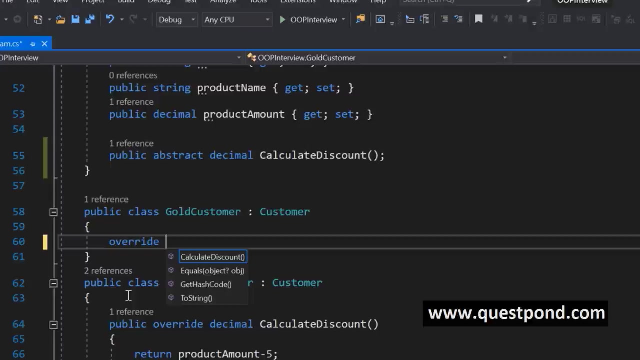 If I remove this word virtual, I will not see the calculateDiscount. The question here, what the interviewer is asking, is that if I declare a method as abstract in an abstract class, is it virtual? yes, it is virtual, because down below you can go and you can say override. 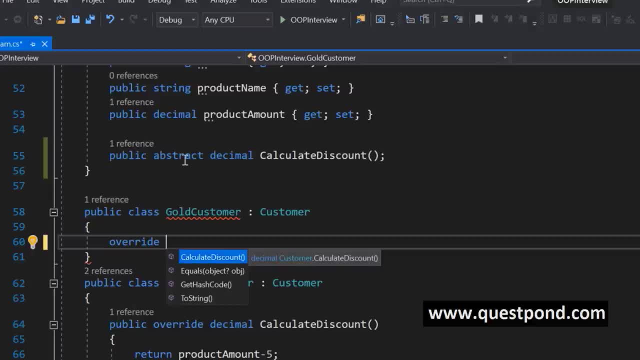 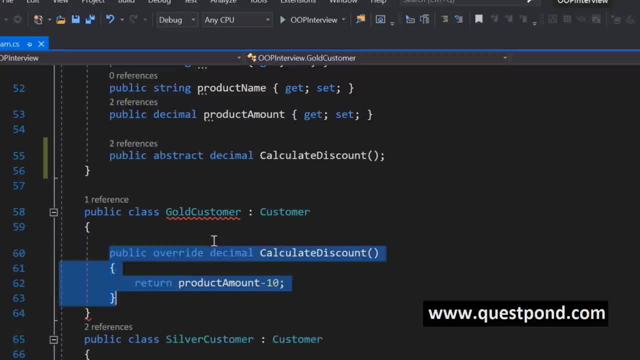 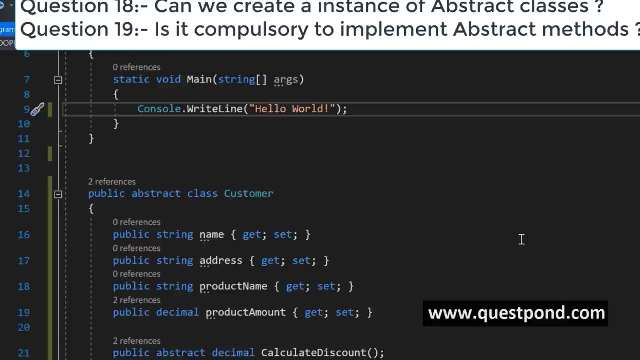 If you don't declare this as an abstract, it will not be seen. Abstract methods in an abstract class are, by default, virtual. There can be some short questions around abstract classes which can be asked, and those answers are just yes and no. but be very careful when you are answering them. 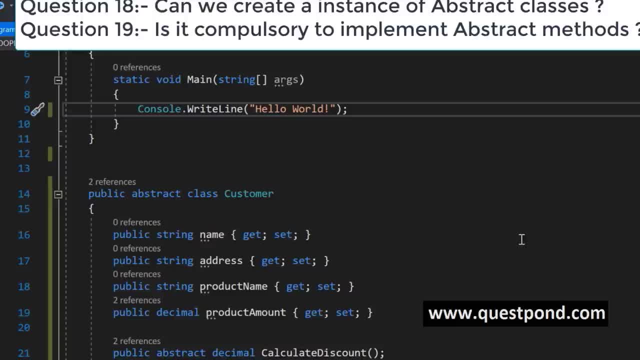 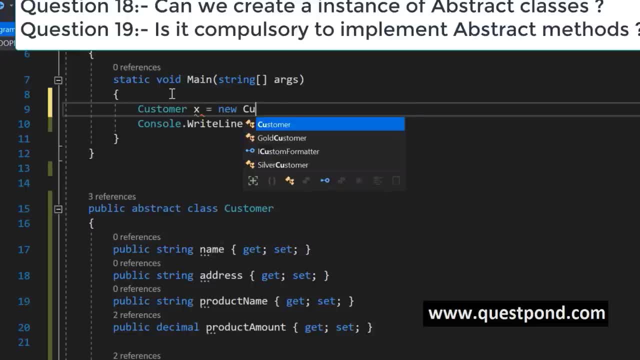 The first short question which comes around abstract classes is that: can we create an instance of an abstract class? Absolutely no. If you can't create an instance of an abstract class, the compiler will throw up an exception. When I say newCustomer, it says you cannot create an instance of an abstract class. 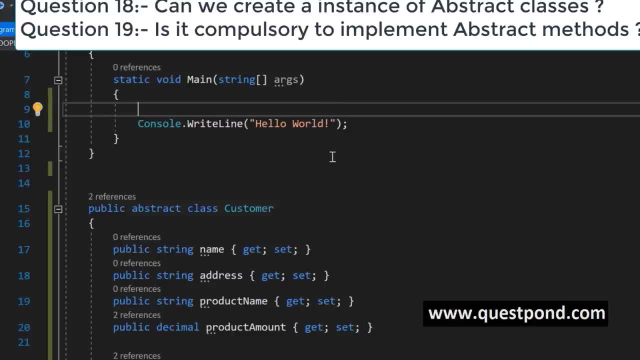 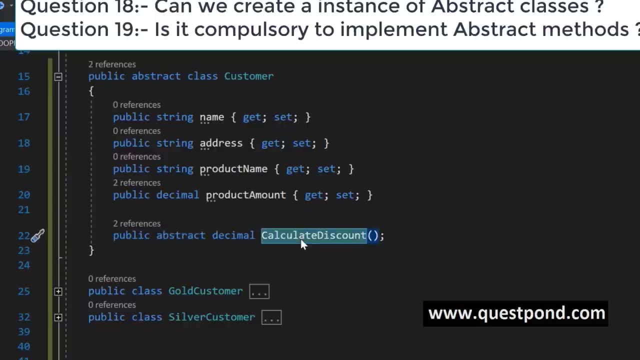 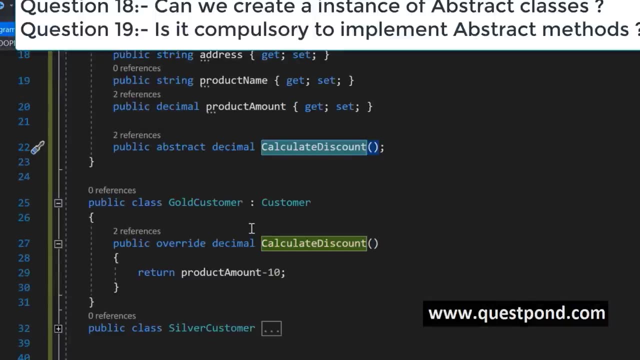 That is the first short question. The second short question which is asked around abstract class is that: is it compulsory to implement the abstract methods in the child classes? Means, for example, we have calculateDiscount. is it compulsory that we should implement those methods in the child classes? 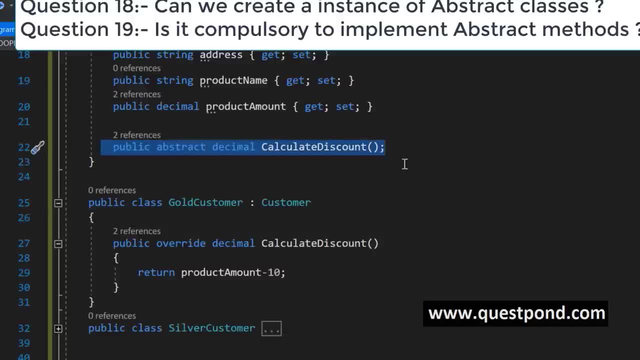 Yes, it is compulsory. These methods are half defined. If you don't implement them- for example, if I don't write a code in the child class- you will see that it gives me an exception saying that the goldCustomer does not implement calculateDiscount. If there is an abstract method or an abstract function that it has to be implemented compulsorily. 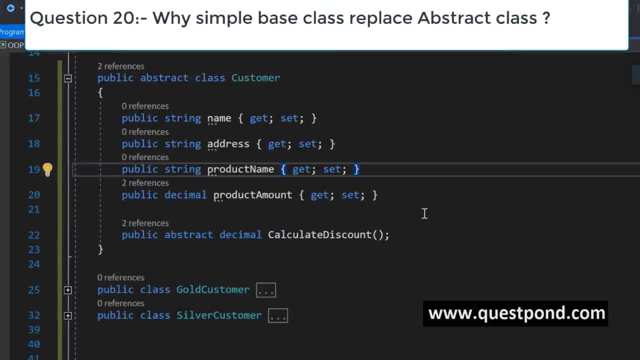 in the child classes. Yes, one more cross question which can be asked around the abstract class is that: why can't a simple base class, simple parent class, replace an abstract class? Now remember that a simple base class or simple parent class, we cannot define it in half-way. 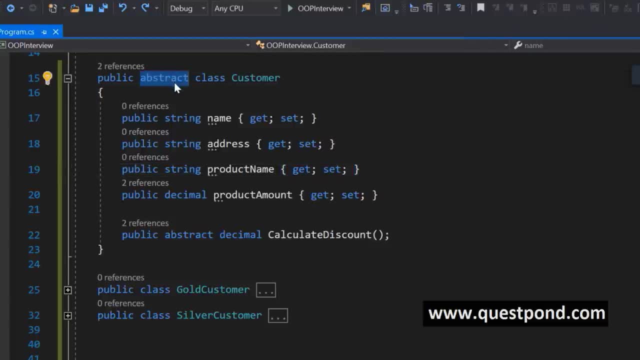 we cannot define it partially. In other words, for example here, if I make it a simple class out here, I need to go and write some kind of an HackLogic. So if I have a simple class, like it calls rinal of ali after here, then I need to go an. 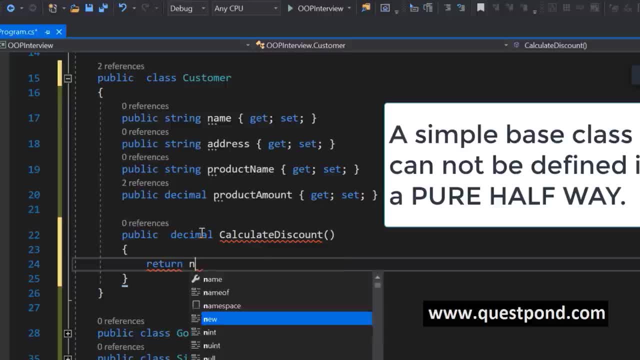 write some kind of a Mangager Application, Add a string strings Or for example. for example, if I create a responsive learning class, all right now. so that' example I will say here return null, or I will say return zero, or must be, I will say throw. 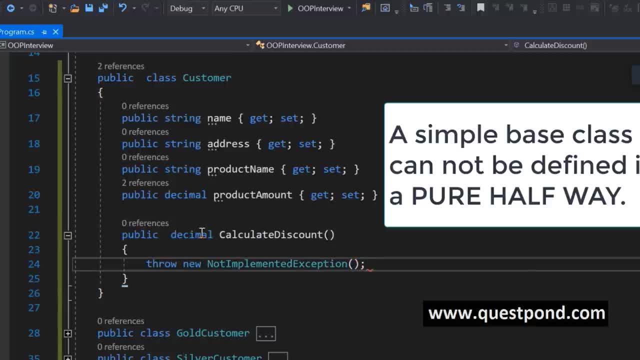 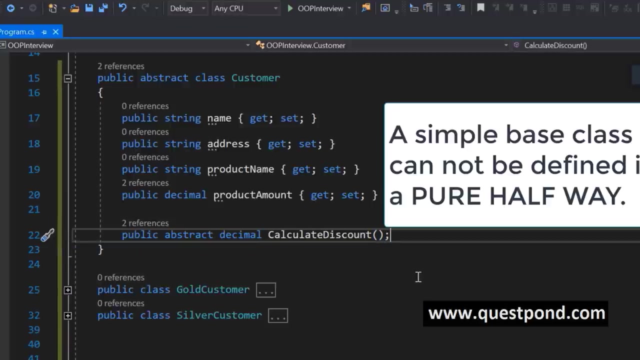 new, not implemented exception. It's not a clean way of creating a half partial class and half base class. it's like a hack. but when we actually go and create an abstract class, this becomes a pure partial class. some things are defined and some things are not defined. 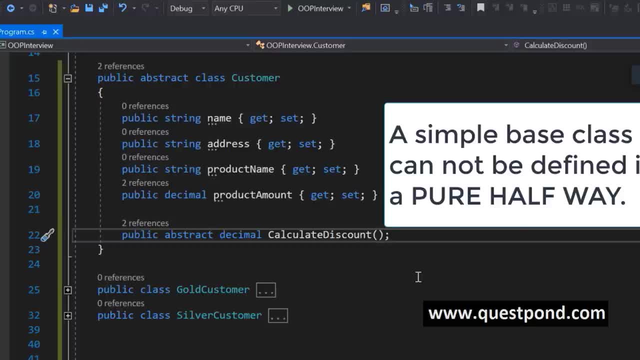 The difference between a simple class and an abstract class is that abstract class is a pure half defined class, while a simple class is a class. and if you want to make it half defined then you need to go and write those hack logic, then you need to go and write those. 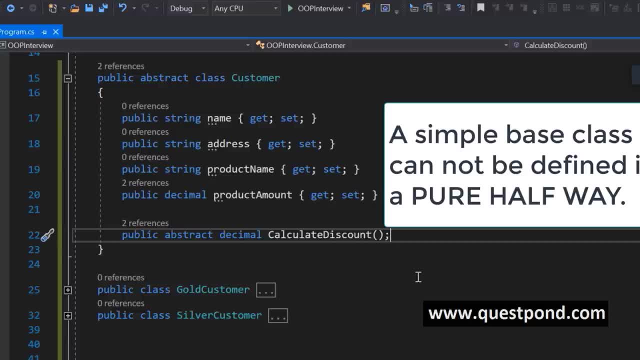 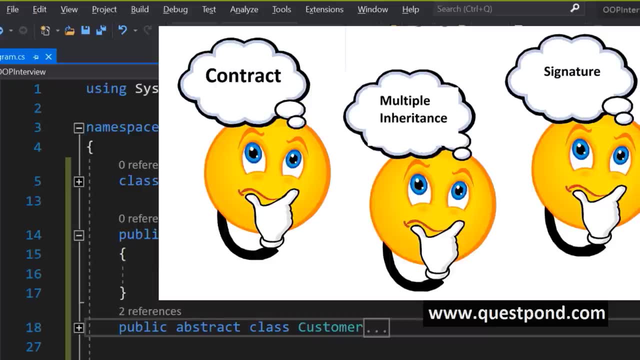 logic, which can be very uncomfortable in terms of programming. Now let's talk about interfaces. interface is where all the confusion happens. the main root cause of the confusion is that interface has lot of benefits and every interviewer wants to hear his benefit in the interview, like some interviewers would love to hear. 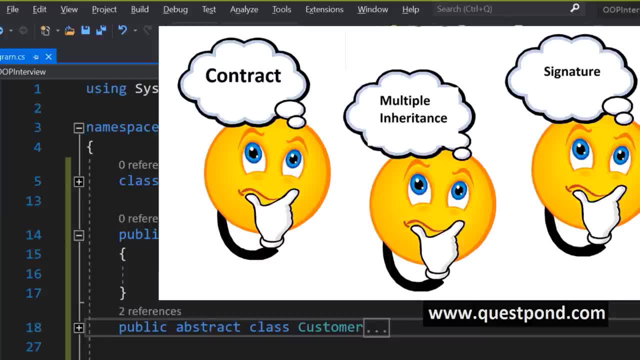 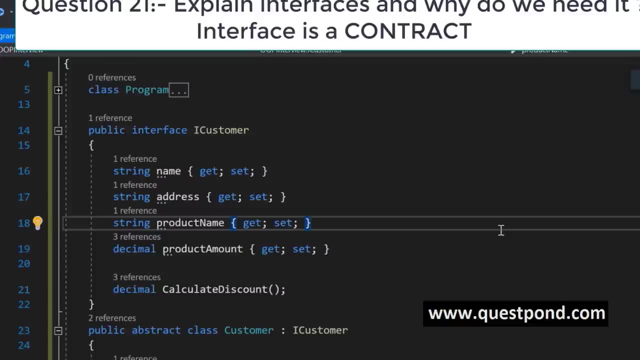 that interface is a contract and then some would love to see that you speak about multiple inheritance and so on. That's why, when we try to answer questions about interfaces, it's quite challenging. To my best knowledge, the most widely accepted definition or the most common definition across the industry for interface which I have seen, 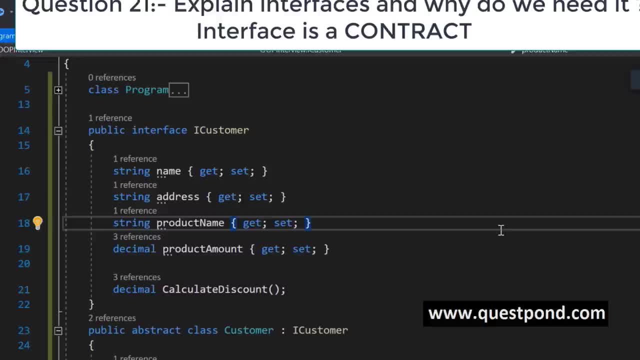 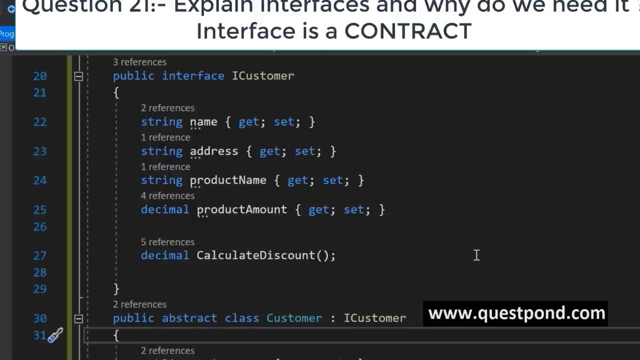 is that interface is a contract. Interface is a contract. it's a legal binding between the developer, who is creating the class, and the consumer, who is using the class. Let us try to understand this statement. interface is a contract because once you say to the interviewer that interface is a contract, you are bound to get lot of cross questions like: 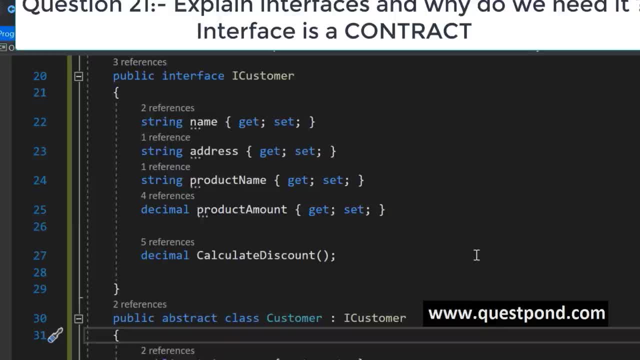 saying that, can you explain what do you mean by interface? is a contract? can you give an example? Let us try to see an example so that you can answer the counter questions in a proper way. You can see a. there is an interface here, called as ICustomer, which has name, which has address, which has 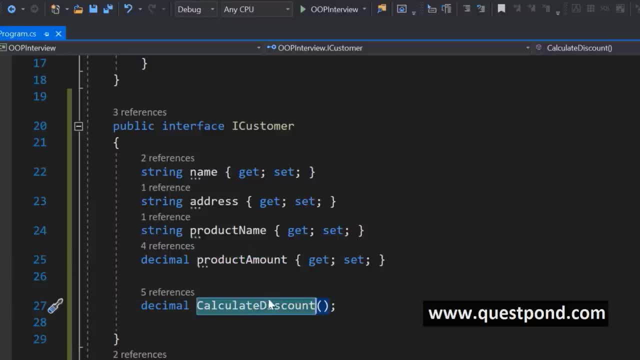 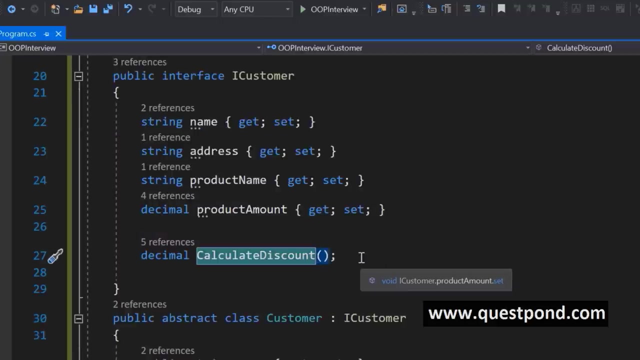 product name which has product amount and calculateDiscount. The first thing you will see that to create an interface you have to write this word interface and all the properties or the method names or the functions are just pure signature. they don't have any logic. In other words, you can see this calculateDiscount function out here. you can't write any logic. 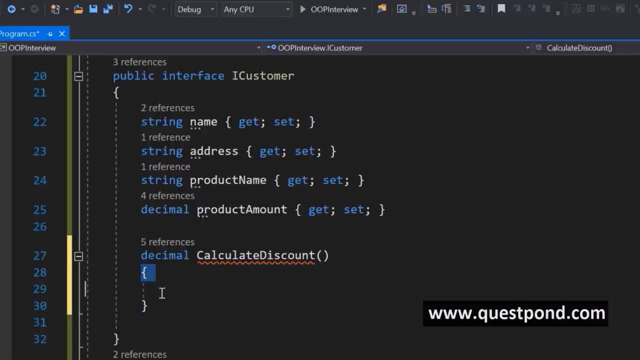 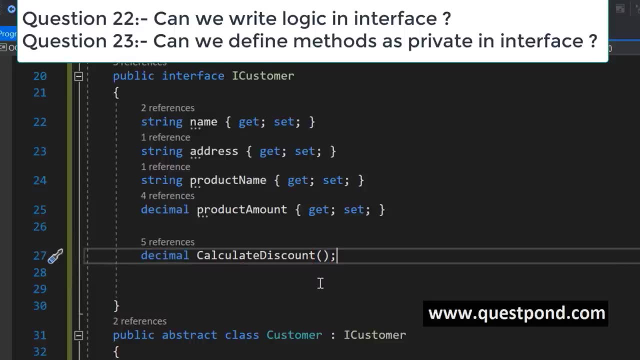 in an interface. Please understand in case if the interviewer is asking you that, can we write some logic inside the interface? no, you can't. in interface you can only have signatures, pure signature. The second thing you will notice out here is that I have not defined here anything called 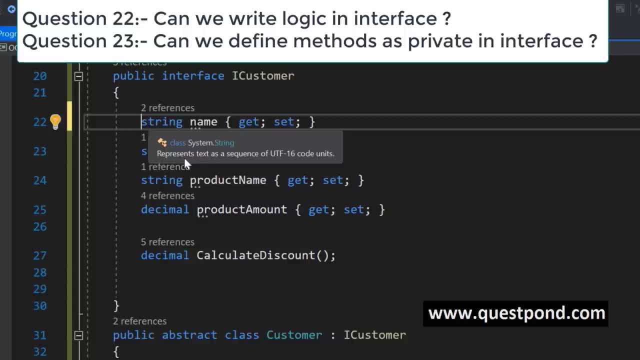 as private or public, by default. all the methods of the interfaces are public. all methods, all properties, all functions are public. Two things Remember in an interview he can ask you that: can interface have logic? no, interfaces cannot have logic. second, can interface have other than public, like private or protected right? 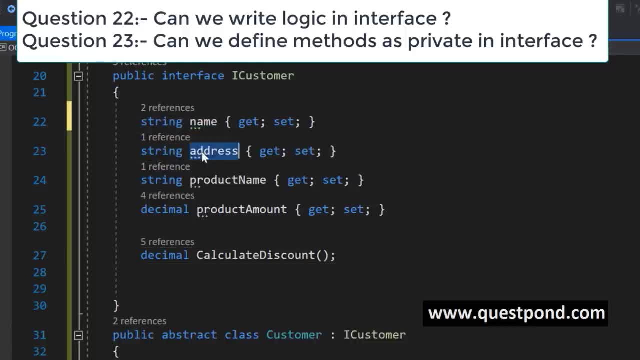 no, all the methods, all the properties in interfaces are always public. You can't even write here public. you know by default it is. public means if you try to write, your public is okay, but if you try to write here something like private, he will give you an exception saying that no customer must declare a body you know and must declare. 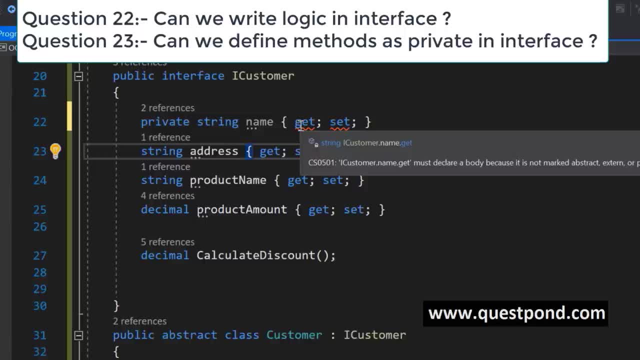 a body, it's not marked as abstract, and so on. in other words, he is complaining that you are putting up a access modifier here, right? So two things remember: interfaces only have pure signature and second, all the properties and all the methods and functions of an interface are always public by default. 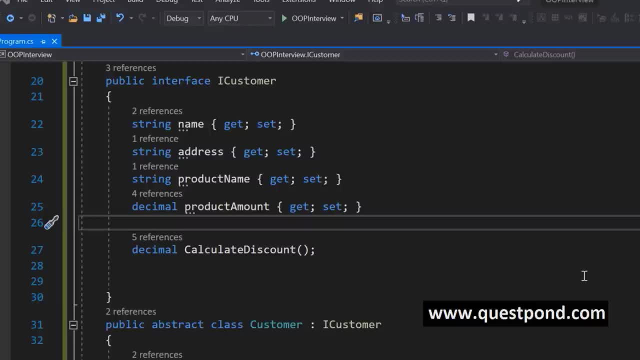 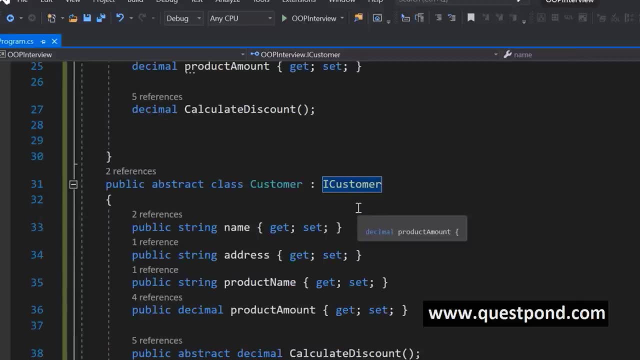 Now let's again come back to the main theme. You know which we were talking about. We were discussing. what do you mean by interface? is a contract, right? so this is the interface here: I- customer. now this I- customer is implemented in this customer class out here, so you can. 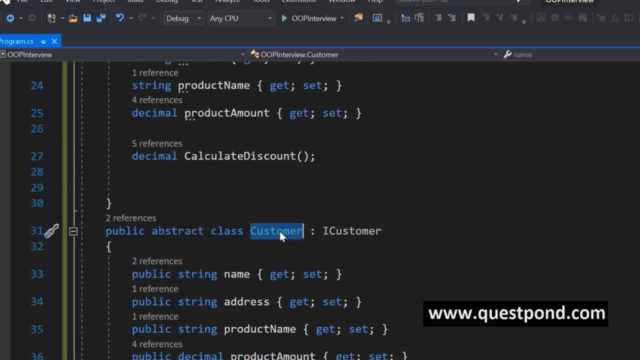 see, here we are saying colon I customer, so we are actually implementing this interface. What do you mean by when we say implement an interface? when we say that we implement an interface, this means that this customer class is now promising that he will follow I customer. 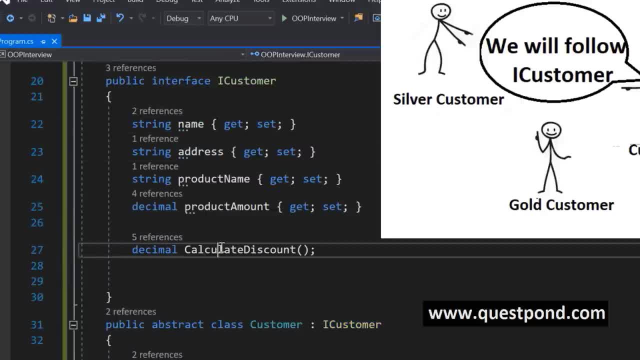 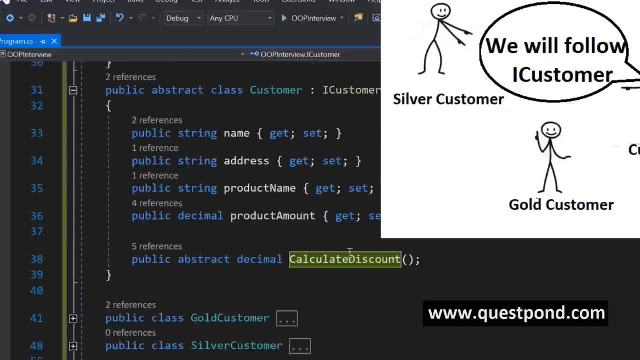 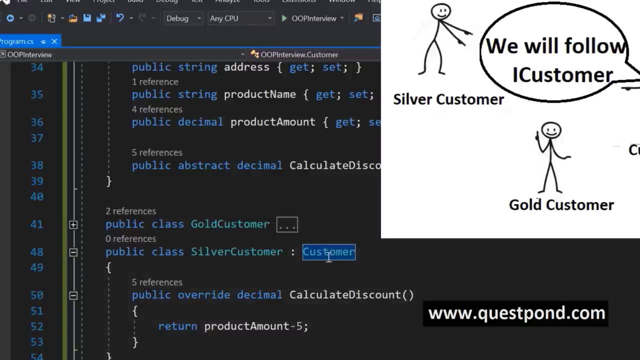 So whatever are the property names, The method names and the function names, right, he will follow as it is religiously right and any classes down below. for example, you can see now this gold customer is inheriting from the customer class right and if you see silver customer which is inheriting from the customer, 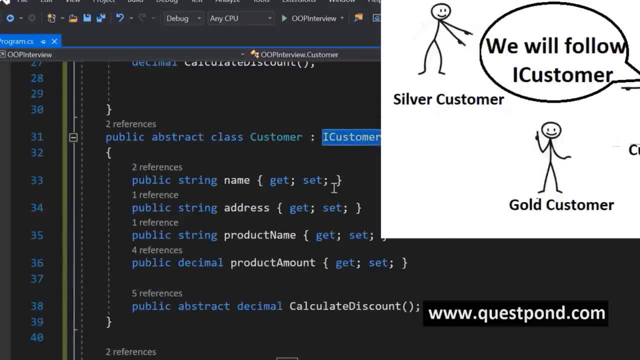 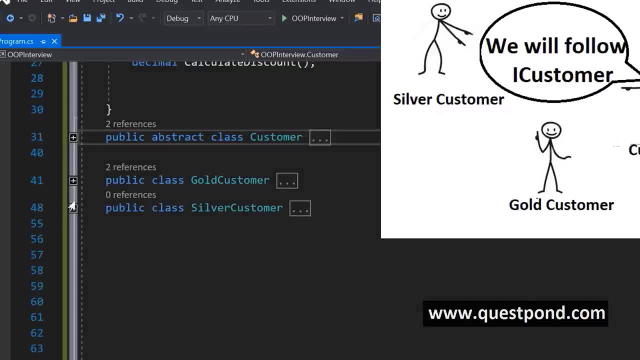 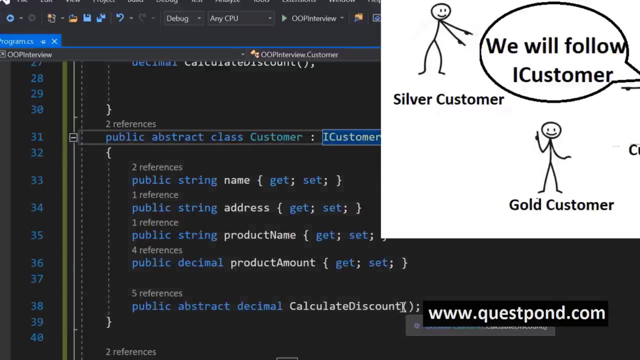 class. they will also follow this I customer because it is coming in the same inheritance, right. So all these three classes out here promise you know that they will follow I customer religiously. In other words, if this customer out here, customer class developer out here goes and changes, 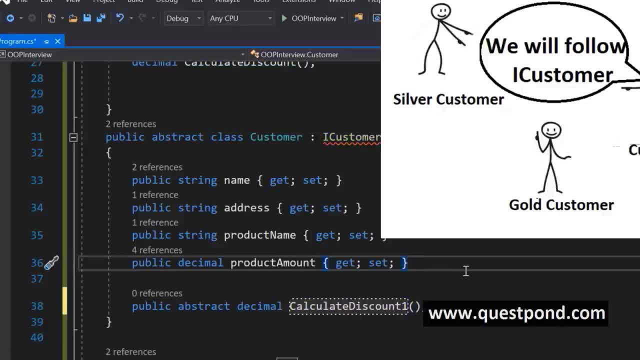 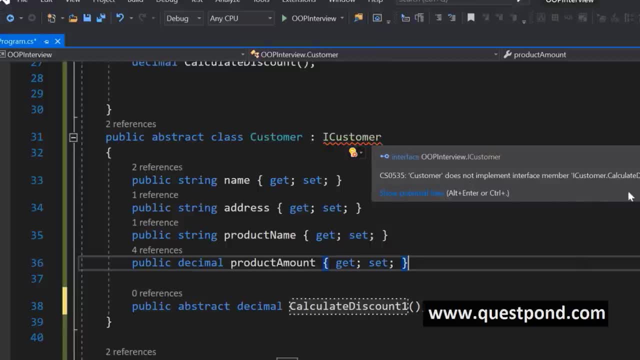 this to calculate discount one. the interface will actually send an alert here. you can see that there is an alert here saying: or there is a compile time error saying that it does not implement calculate discount. please go and implement calculate discount right. So once you implement the interface, you have to follow all the properties and all the methods. 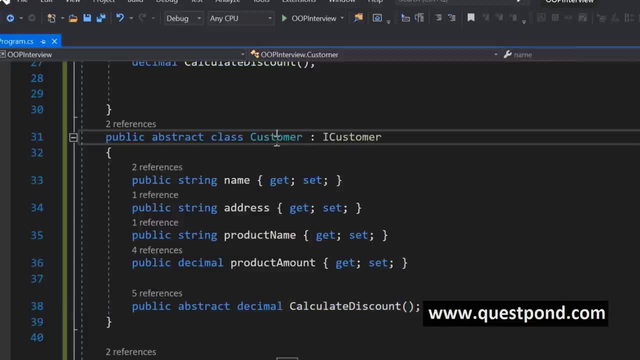 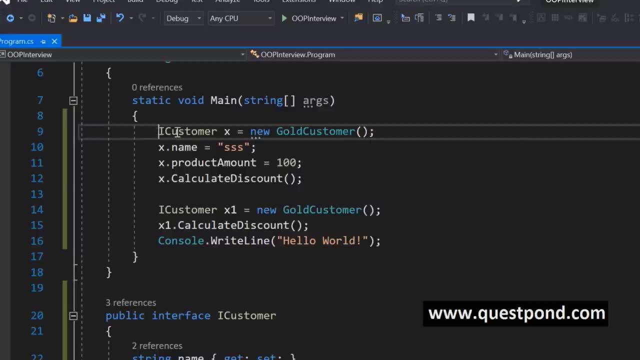 religiously. So that means that This customer class you know wherever it is getting consumed. for example, now you can see here it is getting consumed in two places, here in line number nine and in line number fourteen. so here, when I say, I customer is equal to new gold customer, you can see polymorphism. 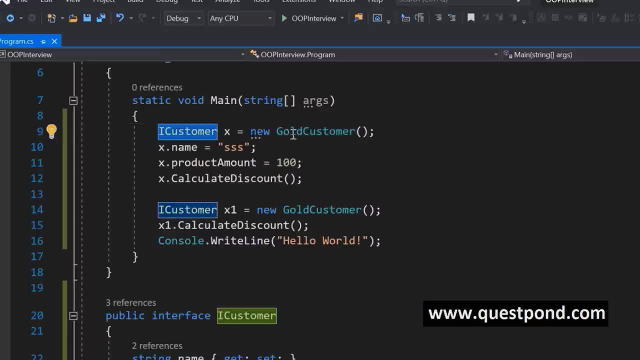 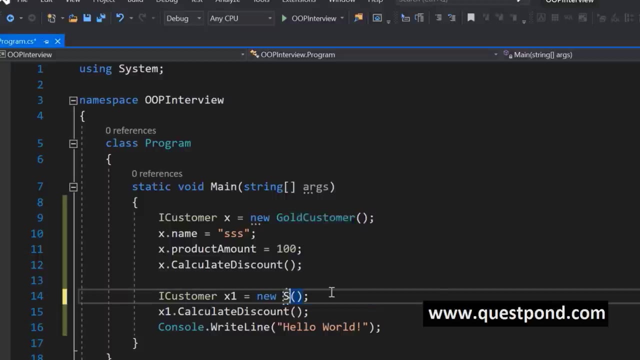 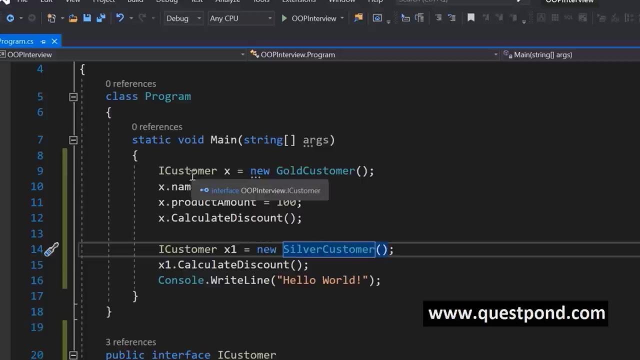 in action. remember, in polymorphism on runtime, you can point to different, different instances. right? so you can see, I customer interface can point to gold customer. it can also point to The other type of customer, which is silver customer, absolutely right. So now here, wherever the object is getting consumed, the class is getting consumed, right? 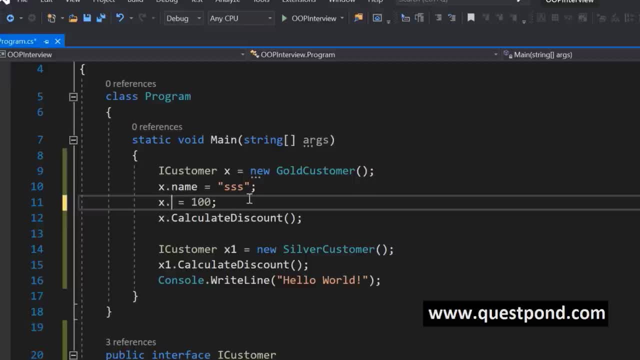 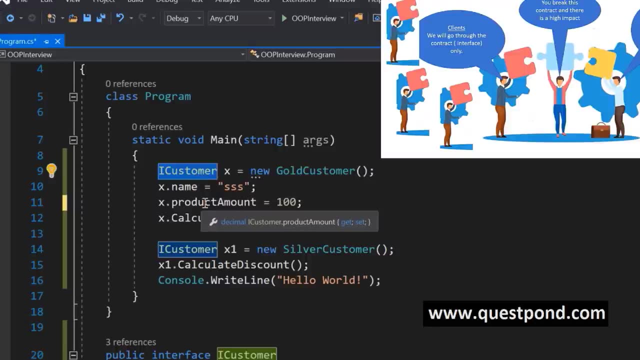 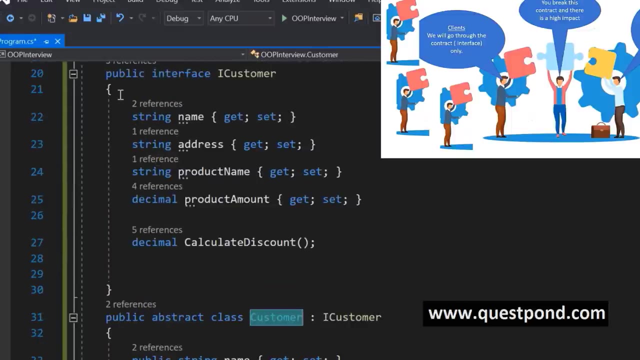 I'm saying I customer X, so that means now these methods will be followed very religiously. so now, the consumer or the developer who is using your class, and the developer himself: they haven't. they are now bound with a contract. they are now bound with this contract. 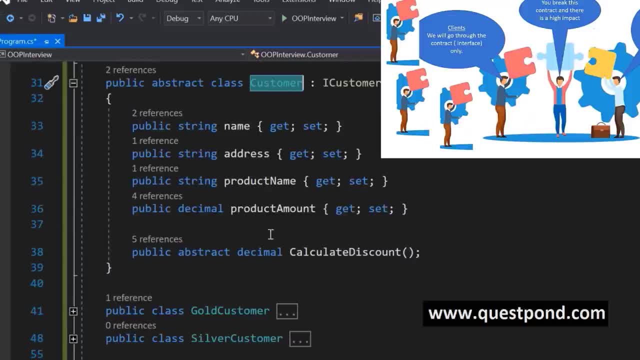 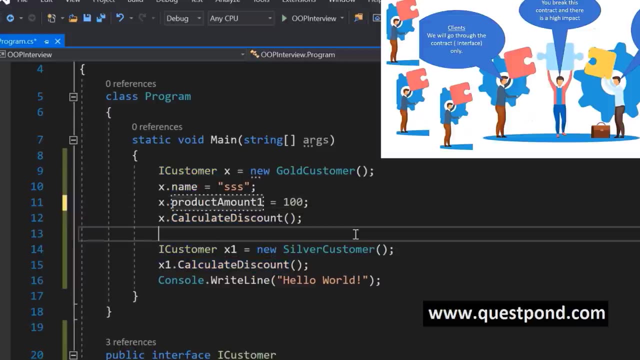 I customer and no one can break it. So if this developer breaks this contract for some reason, if he says calculate discount one, he gets an error, right, he gets an error. and if this client out here, if he goes and put some other name out here, definitely is going to get an error. 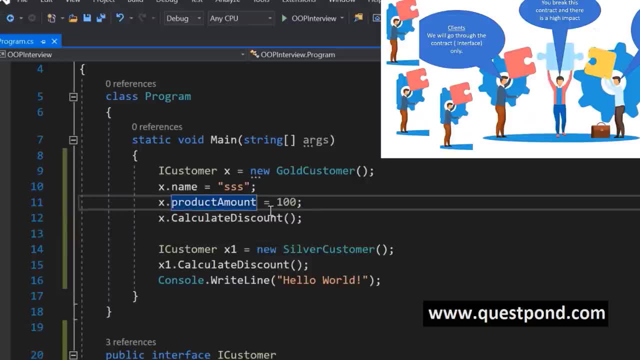 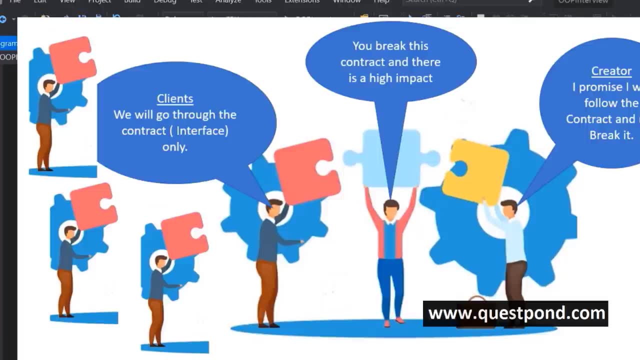 So both of them are now bounded with a contract, both of them have pledged. you know, that they will follow this contract and this contract should not change. But again comes the same question. so by having a tight contract, you know, between the consumer, who is consuming the class, and the creator, who is creating the class, what is the benefit? 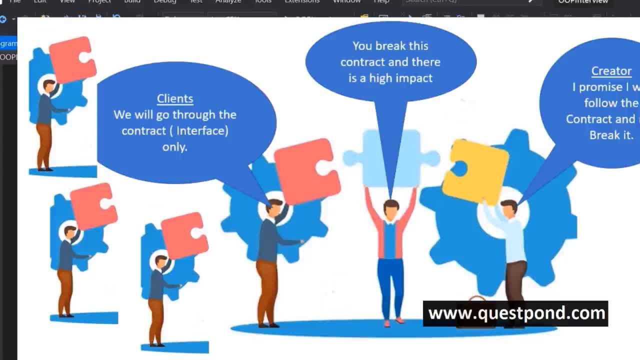 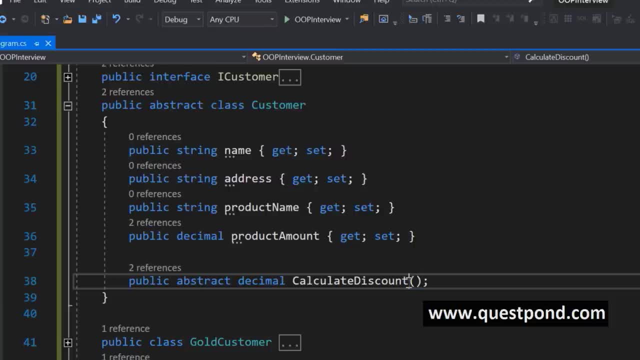 of it right Now- think about this- that this developer who is creating this customer class out here does not have an interface. assume that there is no interface out here. So now what happens is if he goes and if he changes this to calculate discount one, he 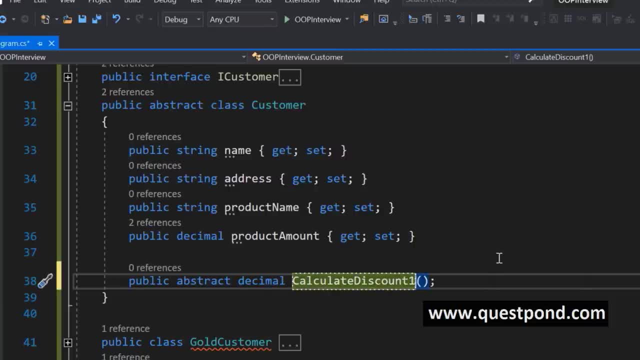 has no idea where it can impact. There is no alert out here. he thinks that he is working in a silos. he thinks that if he changes this, no one is getting affected, right? But now, if he has an interface right now, if he has an interface out here, and if he goes? 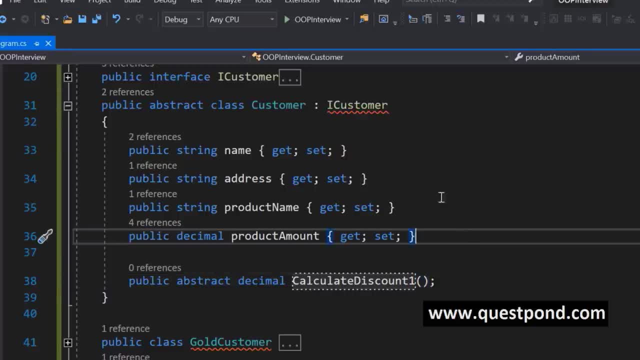 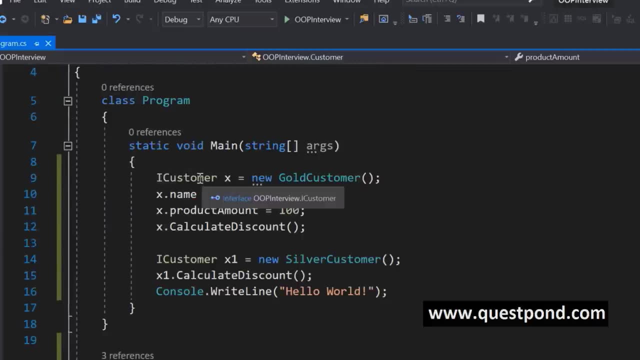 and changes something out here. now there is an alert here. there is an alert here saying that, hey, if you are going to go and change this, lot of people will be affected. it will affect Line number 9. it will affect line number 14. it will affect in some web pages it will. 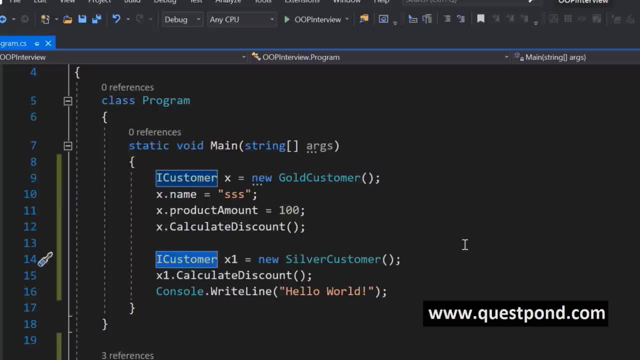 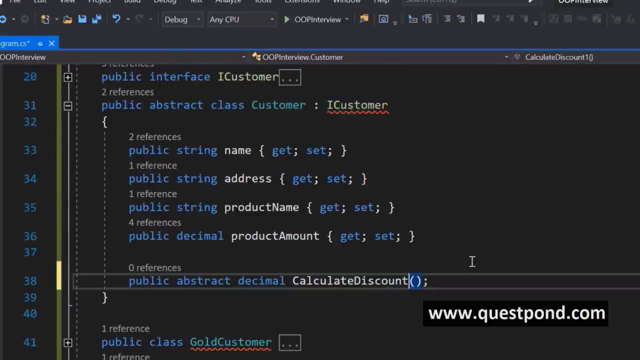 affect in some MVC controller, it will affect in lot of places. So by having a tight contract right, we do better change management, we do better impact analysis. remember that when you change at one place it can affect at lot of places, Specifically in a big software project when it once it goes to production. if you change, 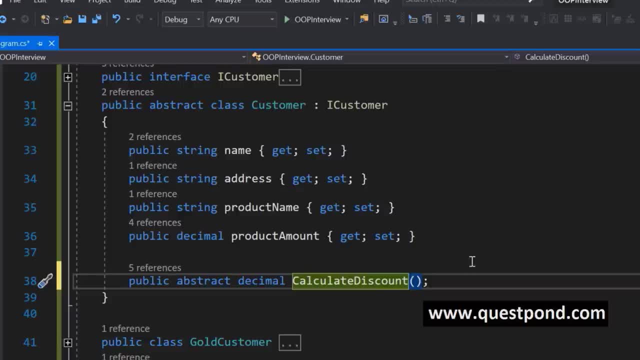 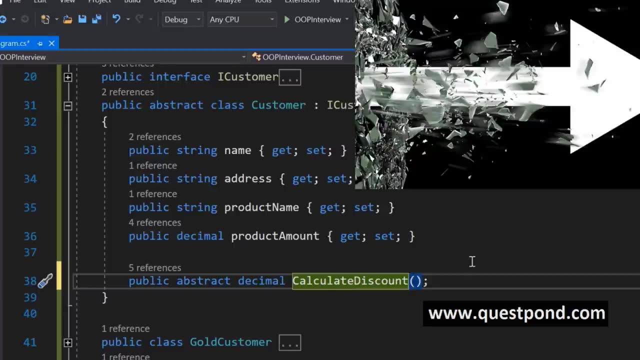 at one place. There should be some kind of an alert mechanism to tell you that. oh like, if you are going to change this, it is going to have breaking changes. it will break in lot of places. So when interface says that it's a contract, it means that both the parties are following. 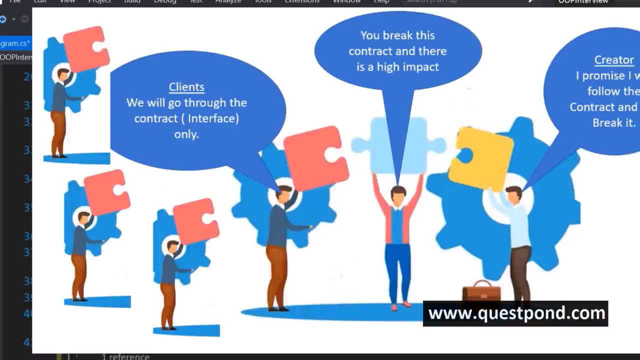 the interface and by doing so you have better control on the impact analysis. you have better control on the change management. also, when you change at one places it will not go and affect in lot of places. So that's why lot of people say interface is a contract and if you follow the contract, 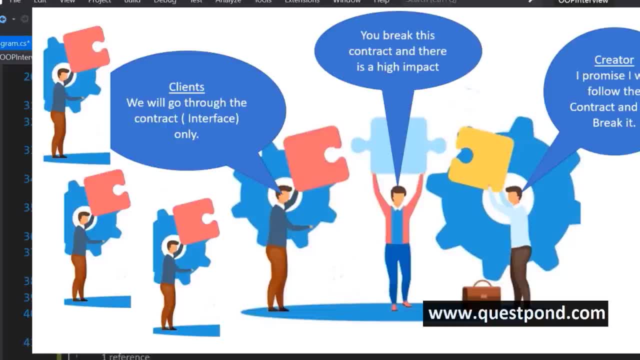 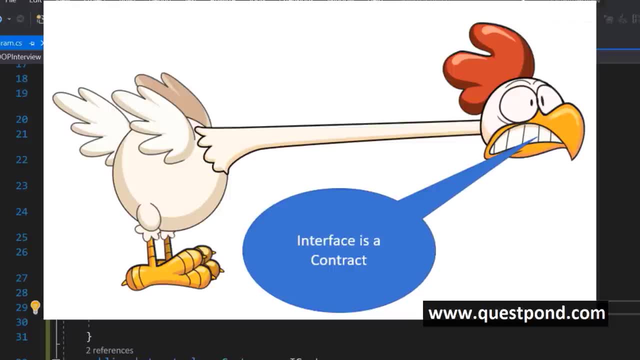 if you don't change the contract, you have a better software running in production, Once you have stuck your neck by saying that interface is a contract, it cannot be broken, and so on. right, if you break the contract, it will have an high impact analysis. the next: 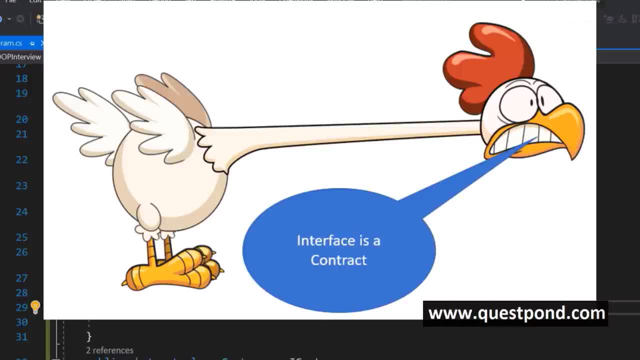 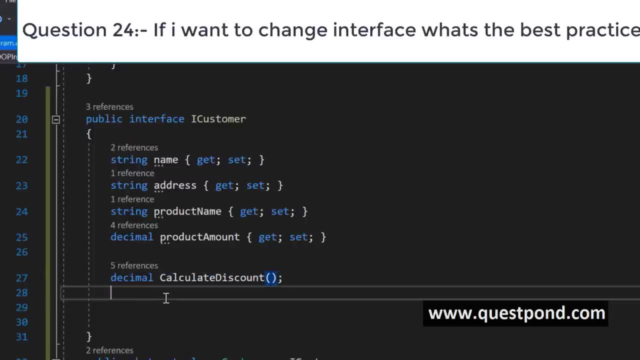 question will come: is that? what if I want to break it? What if I want to change it Right? so let's say your application is running in production and you have a calculate discount out here. what if I want to go and add a new method here saying that this customer will 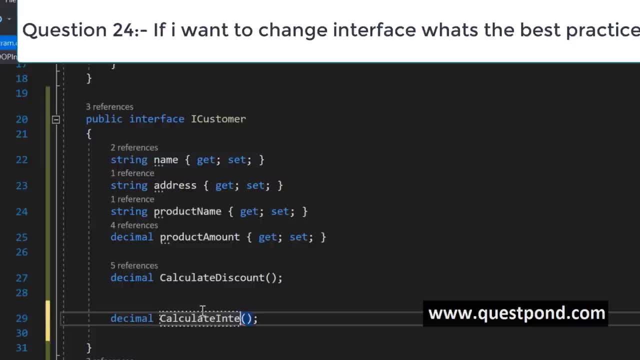 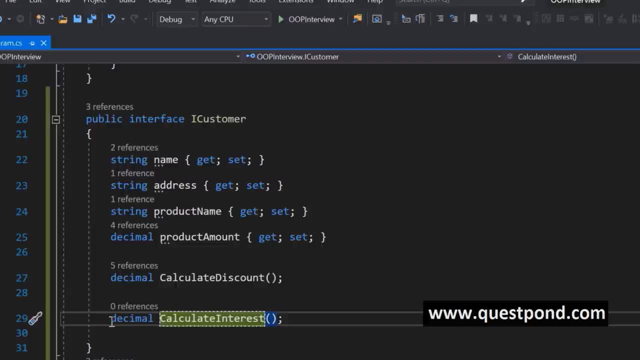 have calculate interest right. so in case if the customer does not pay money, I want to go and add a new method here called as calculate interest. so how does this work? right Now, the interviewer who are who will ask you know this question. you know what happens if. 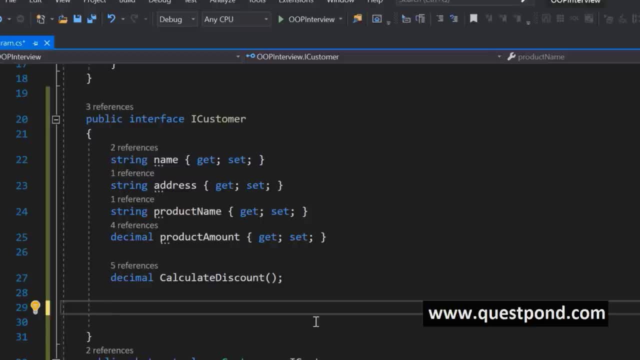 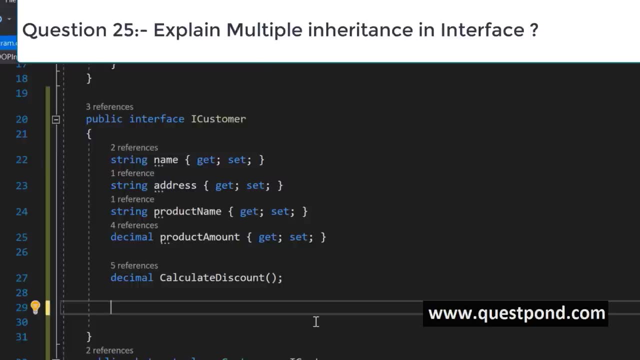 the Interface can be changed are also those interviewers you know who love to hear that interface can do multiple inheritance. remember I said interfaces have lot of benefits. one is that some interviewers think that interface is a contract, which is good. some of the interviewers think that 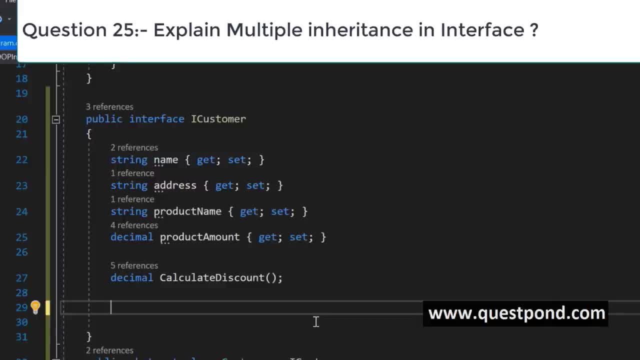 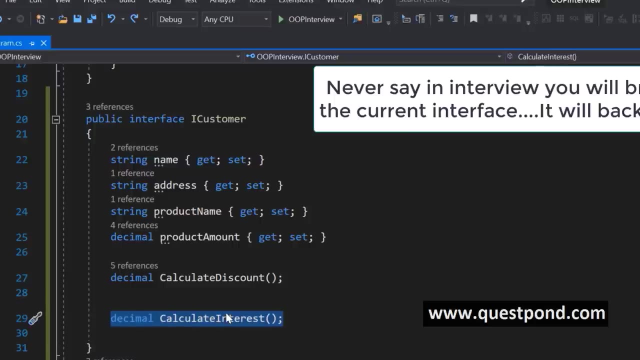 interface is meant for multiple inheritance. so the interviewers you know who look at the answer of multiple inheritance is looking at this answer, that how will you handle changes in interface? So first thing, when someone says that yes, go and add a new method like this: calculate. 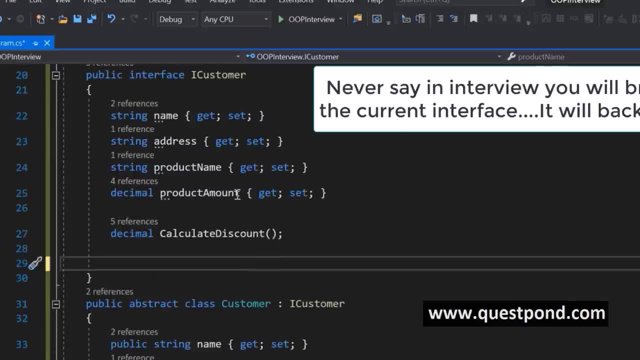 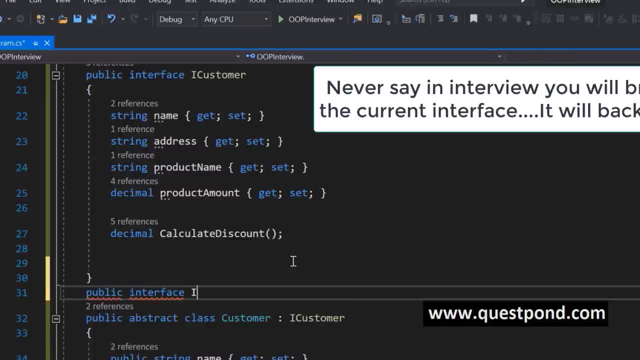 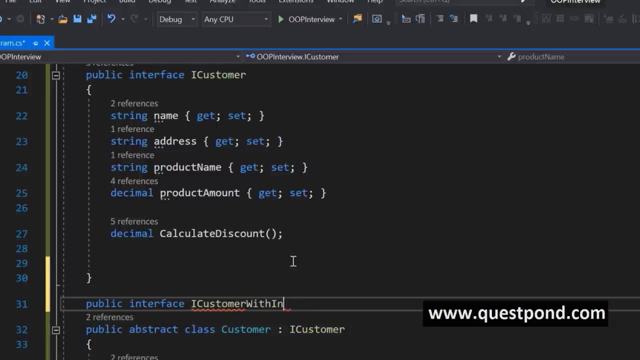 interest. you will definitely not do in the current interface. you will actually create a new interface. so what you will do is you will say: public interface, I customer interest, I customer with interest. Now this I customer with interest will have all the things of I customer watch this it. 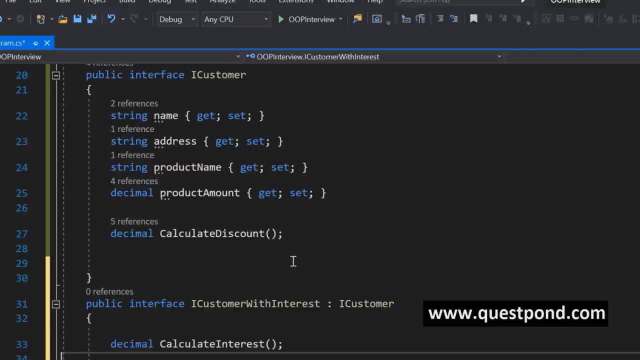 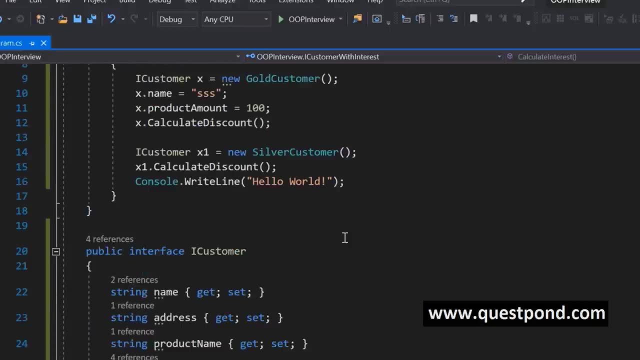 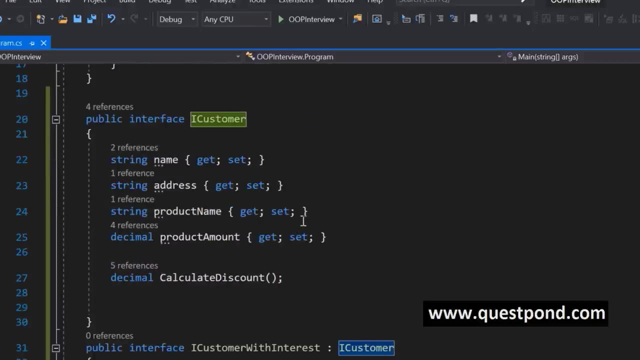 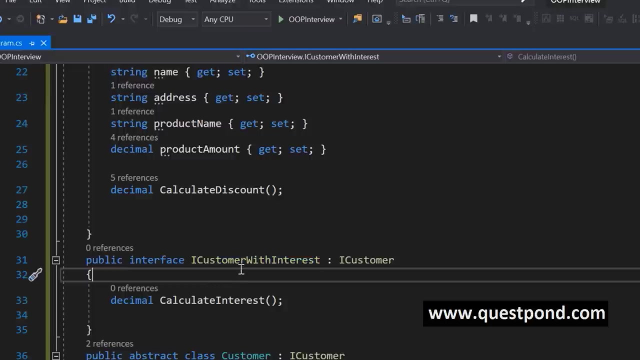 will have all the things of I customer and he will have this extra method out here. So what it means: wherever you know we are referencing I customer, we are referencing I customer here, we are referencing I customer here. all the old places, wherever we are referencing I customer, will not be affected. but you know the new customers who are there or the new. 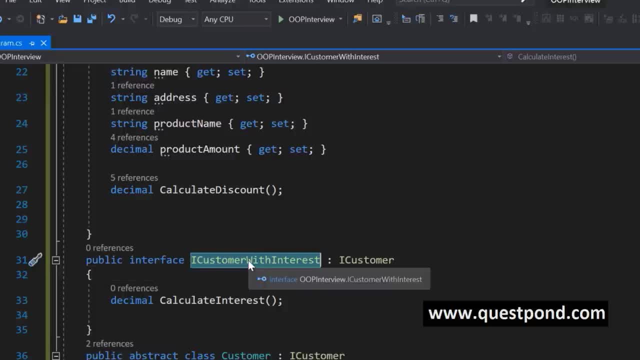 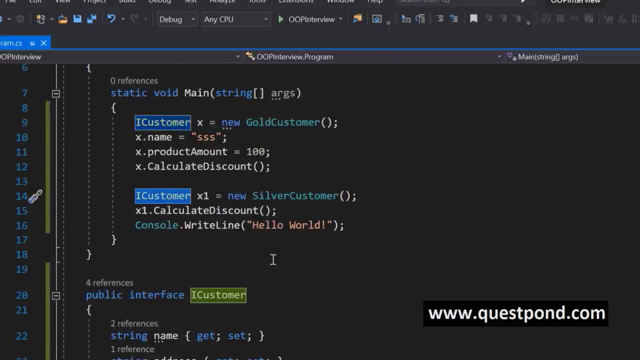 places you know where you want to go and use this interface, they can use it happily, right? So in this line number nine, in this line number 14, we are still not touching them. so whatever is working at this moment will work as it is, because you did not change the 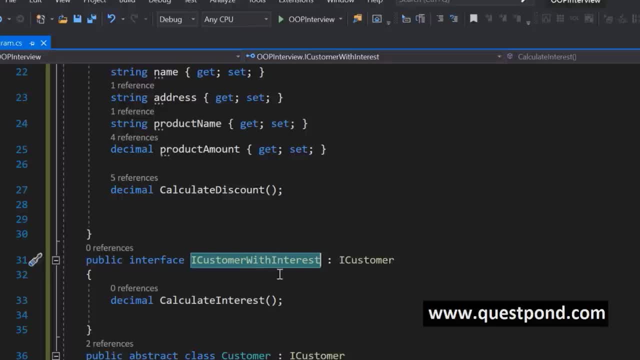 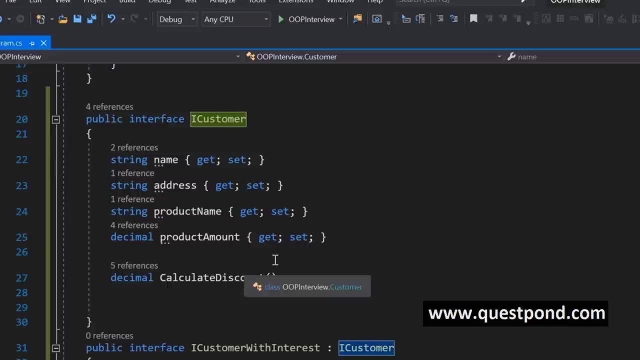 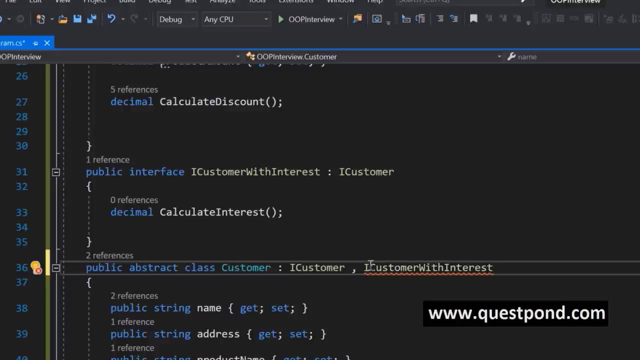 current interface. you actually created a new interface- I customer with interest, right. and now what you can do is you can go and say: okay, so this customer class will implement I customer as well as it will implement I customer with interest. so once you say I customer with interest, 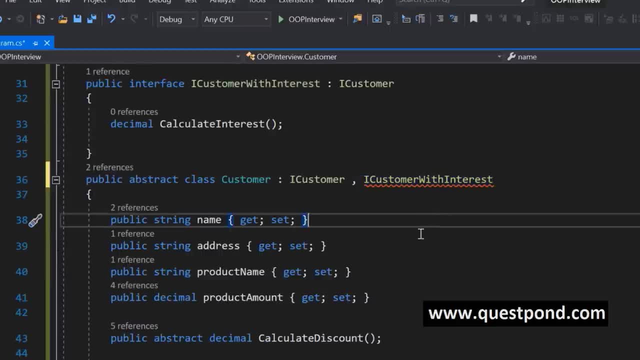 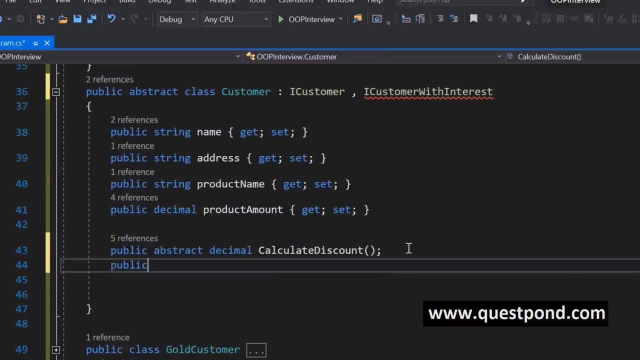 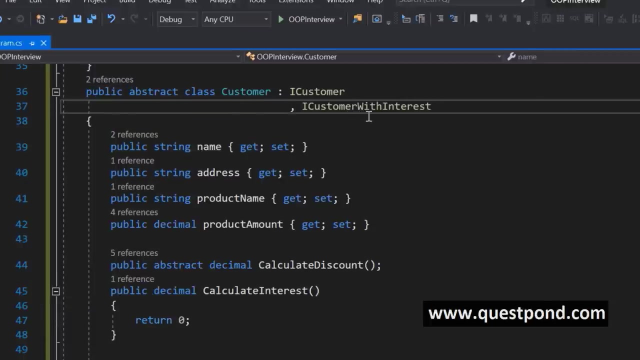 You can see here. now he is complaining here, saying that you have said that you will implement iCustomer with interest, so we need to now go here and implement this method. Once you implement this method, you can see that the error goes away. This is termed as multiple inheritance, so you do multiple inheritance when you want. 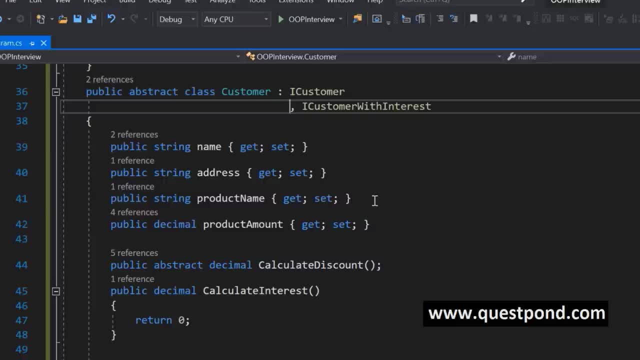 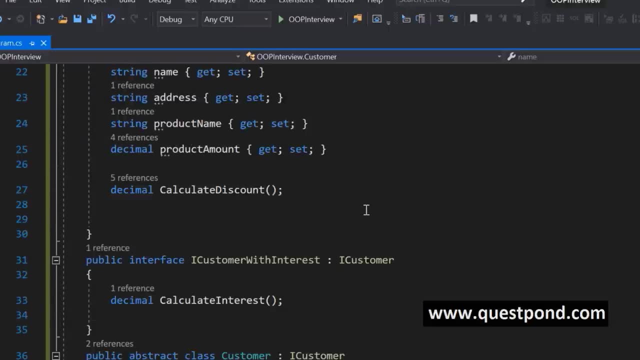 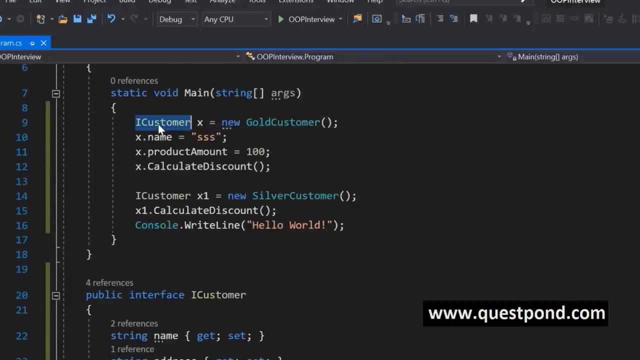 to change the interface. One of the scenarios when you do multiple inheritance is that when you want to go and say that now I want to go and add new interface or new methods, then you go and you create this interface. The old code works as it is iCustomer and whoever wants this new method with interest. 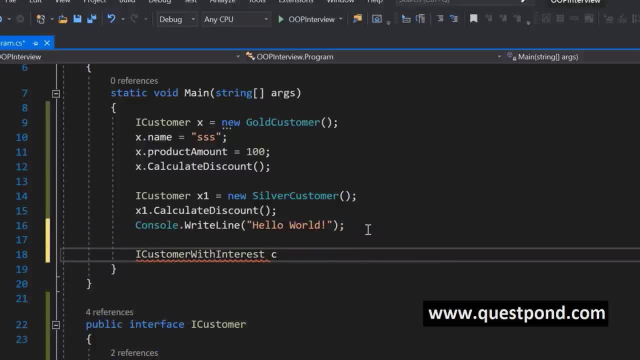 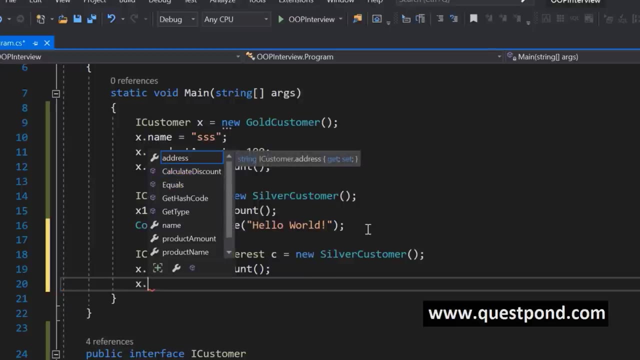 will use. this one, he will say, is equal to new SilverCustomer. He gets calculateDiscount from the old interface and he also gets calculateInterest. One of the things wherein we use multiple inheritance is for versioning. This is iCustomer for the old interface. 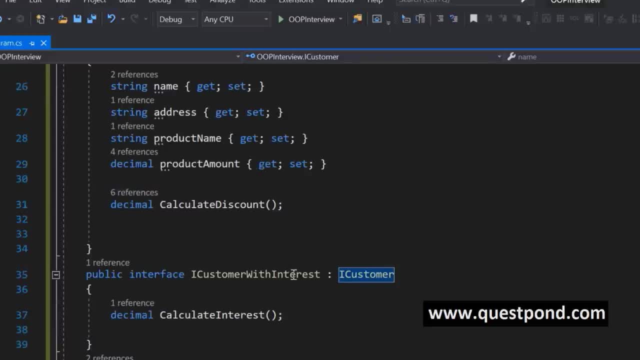 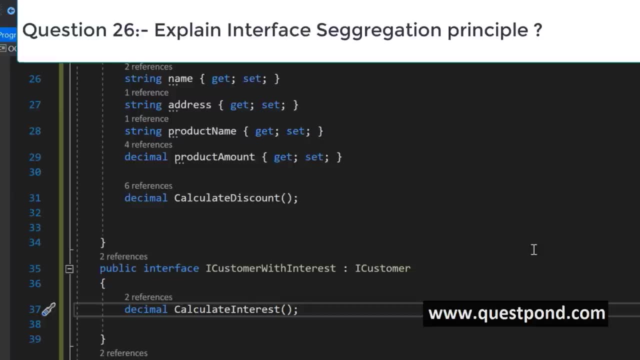 The old places where the customer class is getting consumed, and iCustomer with interest for the new places where they are interested in calculateInterest. Also, interviewers who are very specifically interested to hear about multiple inheritance or multiple interfaces. they would love to see that you understand SOLID principles. 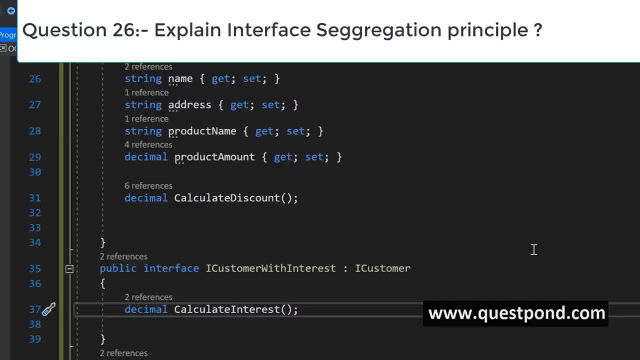 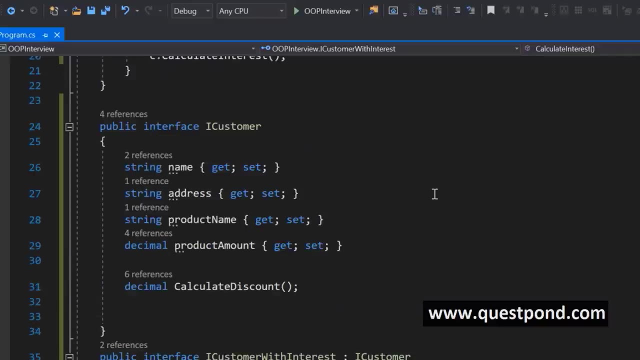 SOLID principles in that i stands for Interface Segregation. A lot of interviewers would love to see that the splitting of the interface which you are done out here is nothing, but it is following Interface Segregation principle. Interface Segregation principle means that you do not force the client to use unnecessarily. 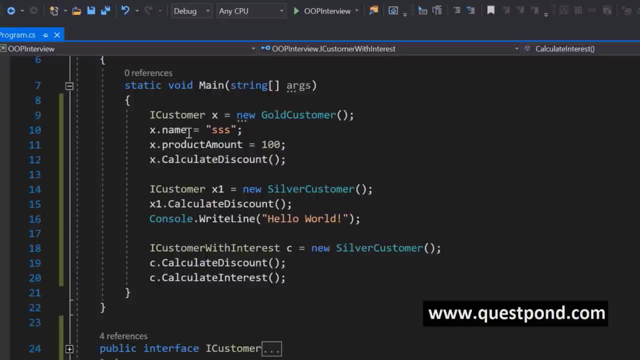 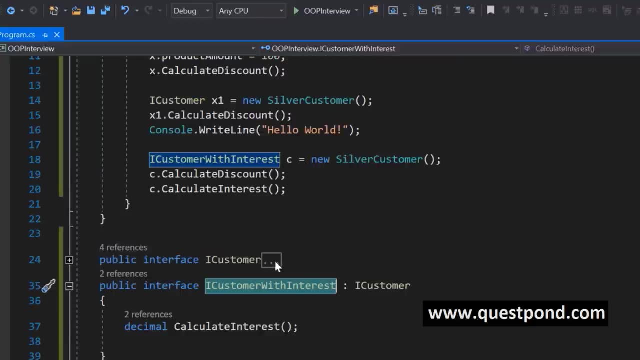 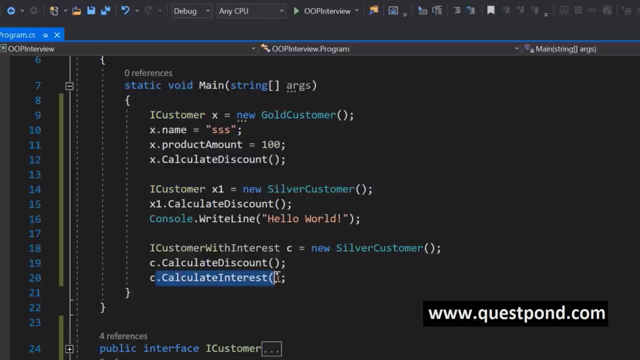 methods which it is not supposed to use. For example, this iCustomer does not have this method called as calculateInterest, while the iCustomer with interest has this method called as calculateInterest. The clients: wherever they are using iCustomer, they are not forced to use calculateInterest. 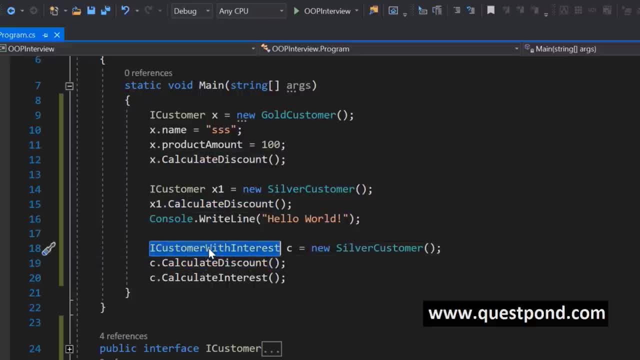 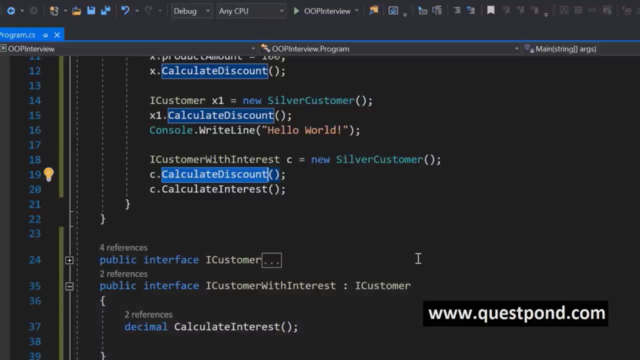 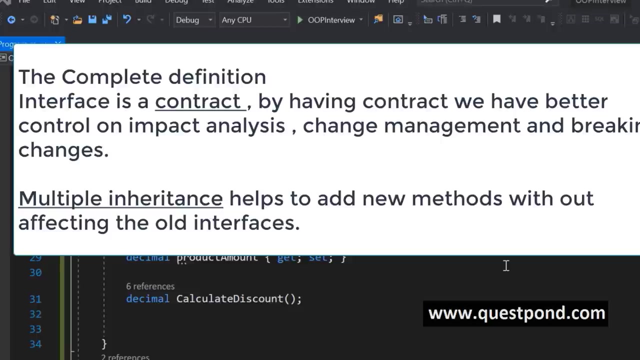 the clients who are seeing this iCustomer with interest. they want to see both the methods. Interface Segregation principle also says that you create different interfaces and you do not force your client to use unnecessary method which he is not interested to use. with all the discussions we have done till now, let us go ahead and put a nice holistic. 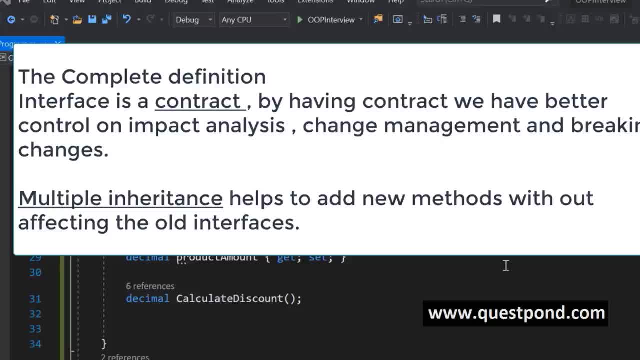 and a complete answer before the interviewer for interfaces. Interface is a contract and by having a contract between the creator and the consumer, we have better change management, we have better impact analysis control and we have better control on the breaking changes. that is the first thing. Second thing: if you want to change the interface, we go and create. 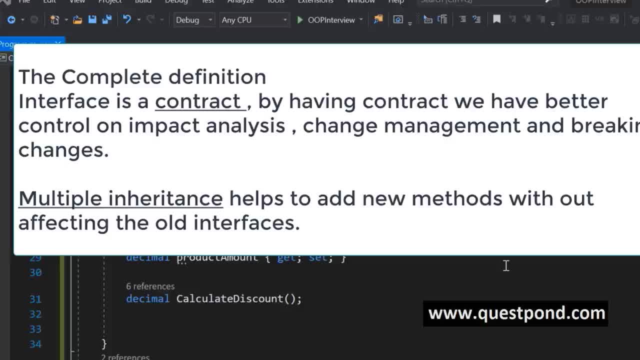 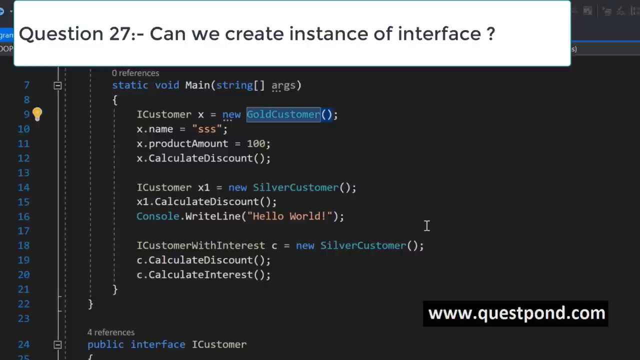 a new interface, because interface also supports multiple inheritance. When we are answering this question, please make sure that you have multiple inheritance and contract properly communicated to the interviewer. So again, some small yes and no questions. can we create instance of an interface? no, you can create an instance of an interface, neither you can. 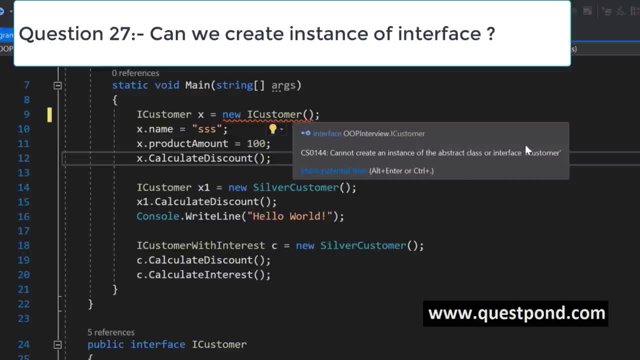 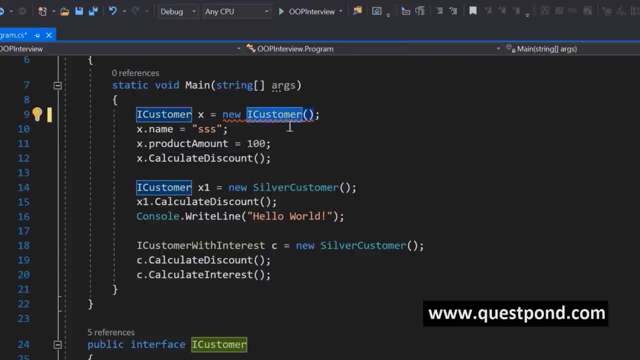 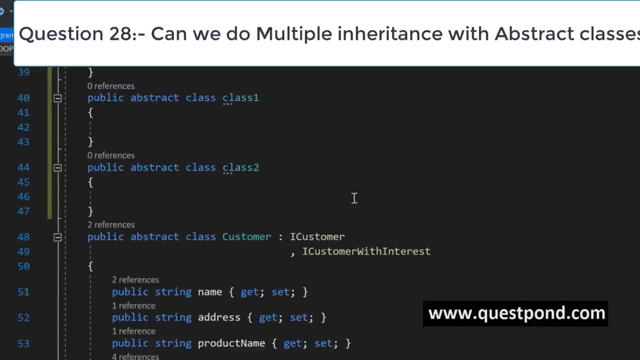 create an instance of an abstract class. You can't create an instance of an of an interface, or you can't create an instance of an abstract class as well. Can we do multiple inheritance with abstract classes? No, you can't. We have two abstract classes here: class. 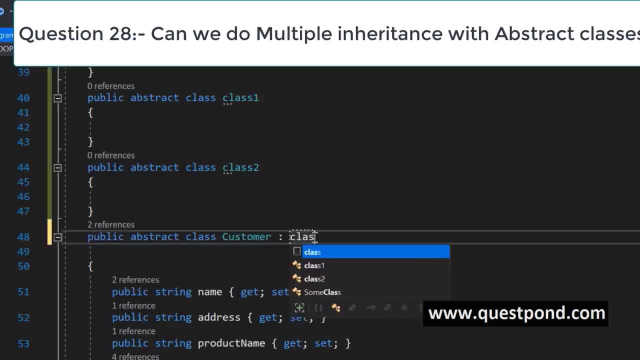 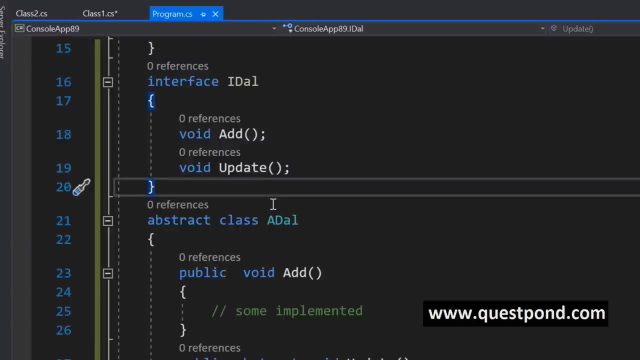 1 and class 2. you can't go and say inherit from class 1 and class 2.. You can't do multiple inheritance with an abstract class or a simple class. You can only do multiple inheritance with an interface, One of the places where the interviewer can really take you for a 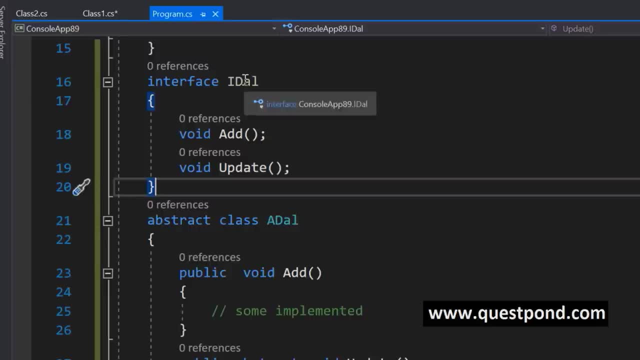 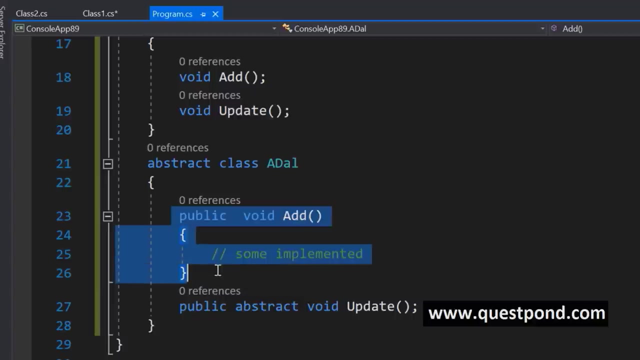 ride is by asking you: what is the difference between an interface and abstract class. Why is this question even asked? because interface is a contract. it does not have implementation. when we talk about abstract class, it's a partial class. some methods are implemented and some methods are not implemented. so why even this? 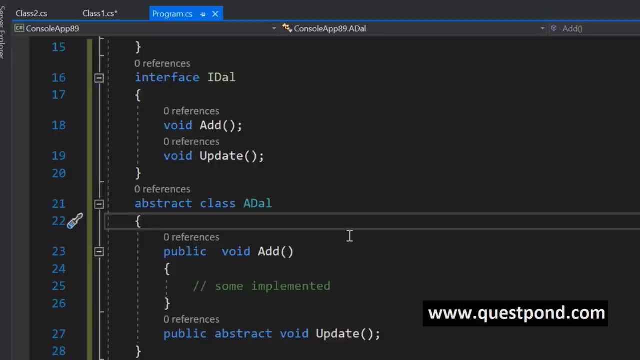 question is arising. There is one place where abstract class and interface look very similar technically. For example, you can see here: this is an IDAL method, which is add and update, and this is an abstract class, ADAL. If I want, I can make all my methods as abstract in abstract. 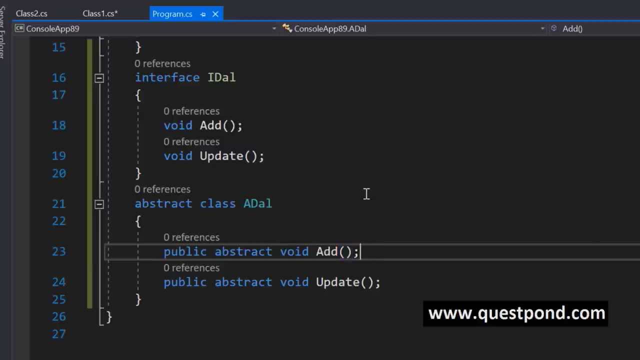 class. If I do this, then there is no technical difference. technically, there is no difference between an abstract class and interface. That's why this question comes up and it is one of the most confusing questions. I would suggest everyone that if you are asked this question, 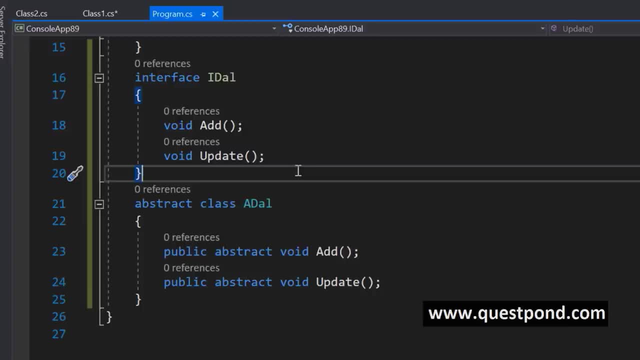 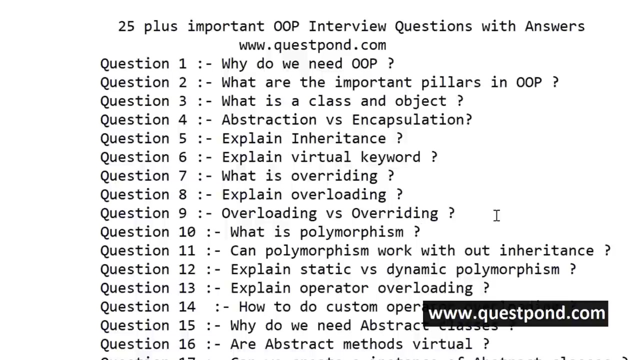 in the interview that when all the methods are abstract and between an interface, what is the difference? If you know the answer, you can go ahead and put down in the comments below. That brings us to the end of this session. out here this one hour session approximately. 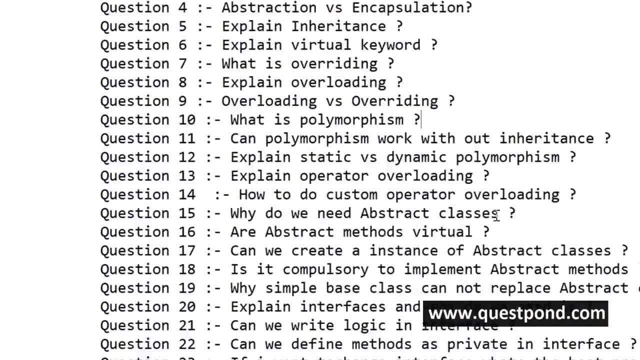 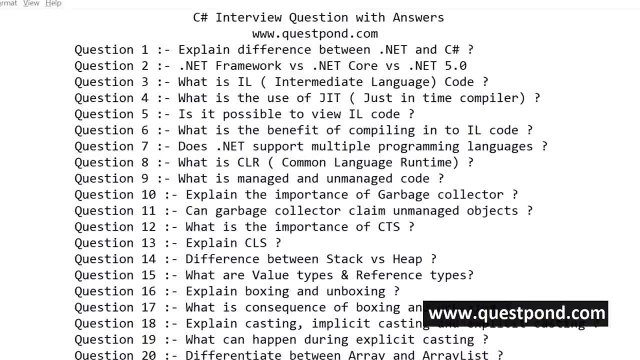 and I am very sure that even if you prepare these 25 plus questions, you should be able to handle most of the questions around object oriented programming Said and done. when you say that you want to go and crack a C sharp interview in a more confident way, in a more professional way, you want to ask for higher salaries, then I would 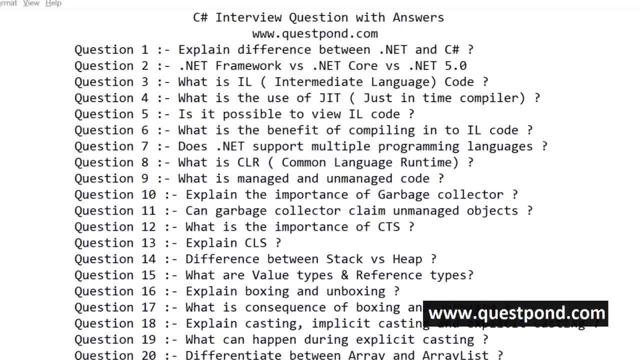 really suggest you to go and prepare holistically. Here is a full end to end C sharp interview question with answers tutorial, which I have created and in this I have covered lot of important topics. for example, when you talk about C sharp interviews, you are asked around garbage collector. you are asked around stack. 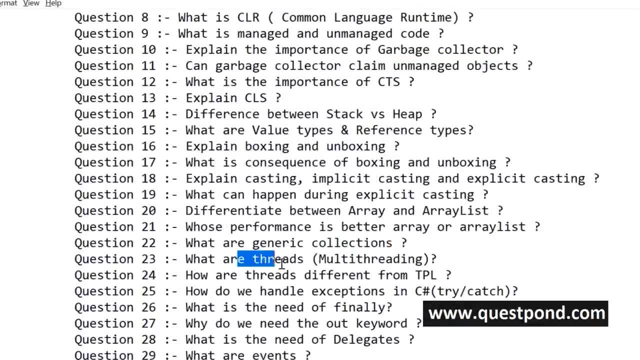 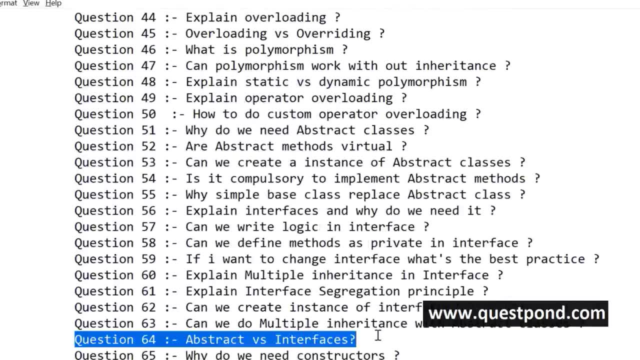 you are asked around heap boxing, unboxing collections, multi-threading, delegates, events- it keeps going. One of the questions which we discussed over here- abstract class versus interfaces- that last question. I have dedicated like 30 minutes only answering that. how can 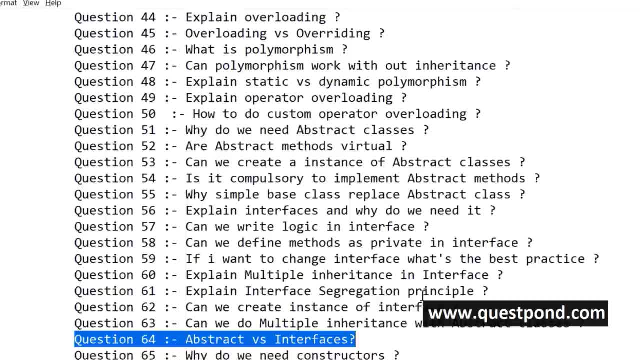 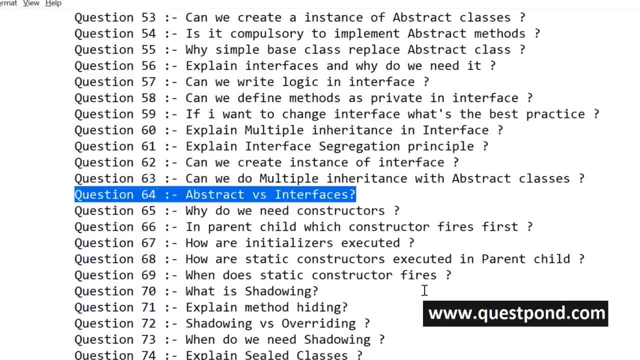 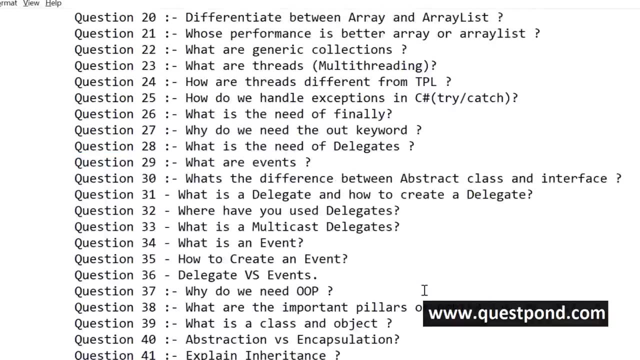 we answer the question around abstract class versus interfaces and if you keep going down below, shadowing sealed classes, access modifiers, solid principles, aggregation, composition, association, partial classes and so many questions out there, When you say you want to really, really crack a C sharp interview. 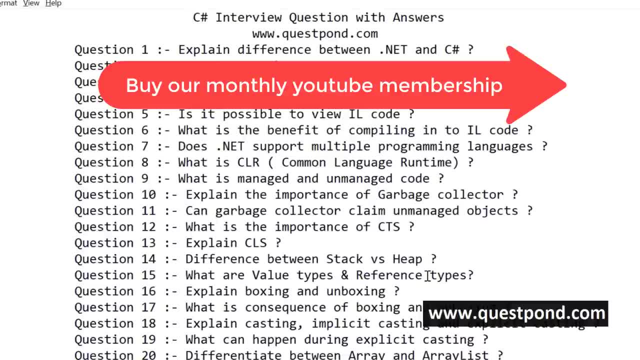 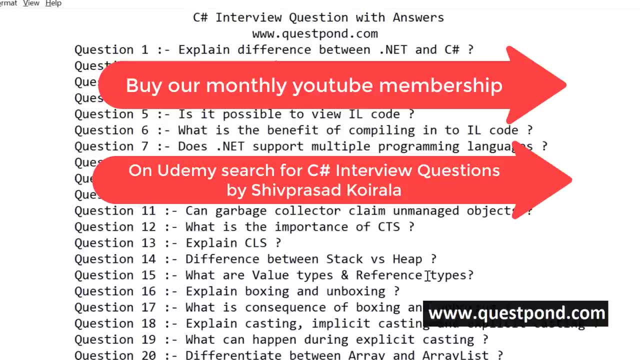 Then this is the course for you. you can get this course from this channel. you can go and you can subscribe to our paid membership if you want. you can go to Udemy and subscribe- we know that also, we have uploaded our tutorials. or else you can go to questpondcom if you.